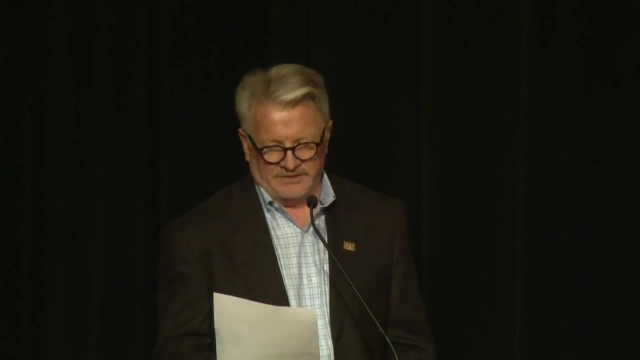 twin of our own solar system is a stretch. so tonight we meet SETI data scientists and Kepler science team member, Jeff Smith, and we also meet Chris Shalhoub, who's a senior research software engineer on the Google AI team and who led the effort to train AI algorithms to mine the Kepler data. so 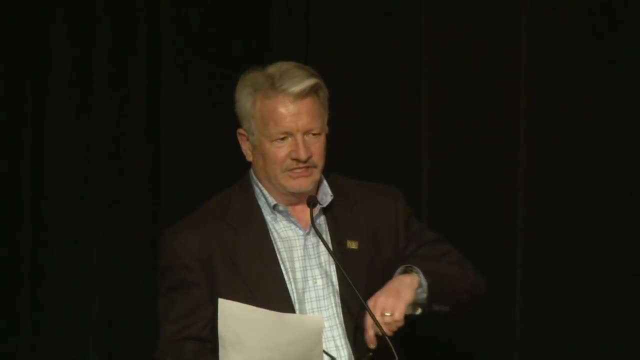 they're going to entertain you and, while you are here, we're going to talk about some of the new discoveries that have been made in the past. and we're going to talk about some of the new discoveries that have been made and inspire you tonight to talk about this new discovery and how. 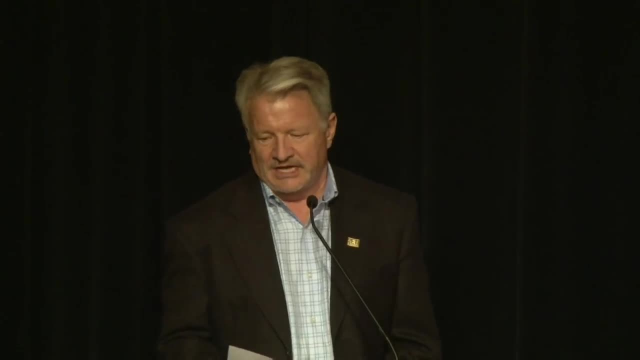 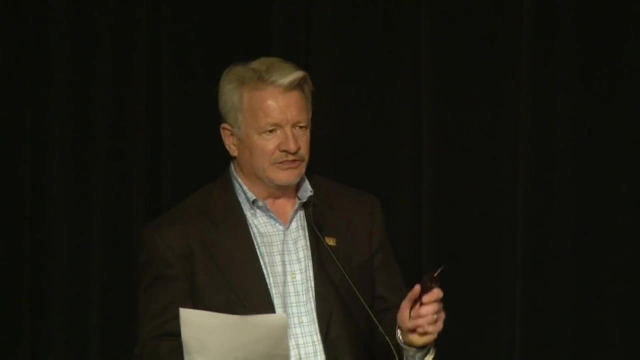 artificial intelligence was leveraged for this, this purpose, and my good friend and colleague Frank Marchese, planetary scientists at the Institute, will introduce our speakers with their biographies and will also host a discussion after the presentations. and then a final little announcement on behalf of somebody in the audience. 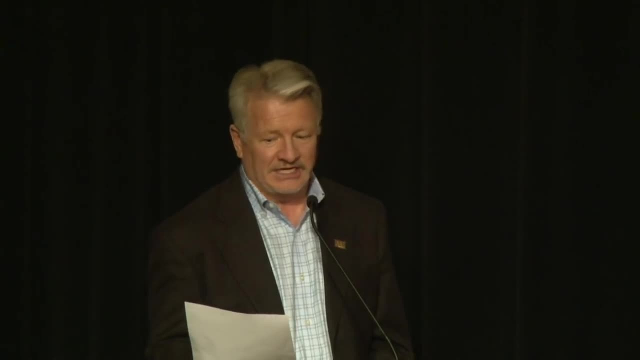 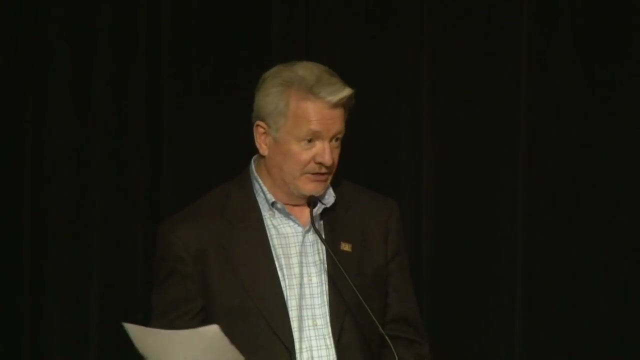 so thanks a lot to Frank and to all our panelists for joining us today, and thank you very much so we'll see you tomorrow at 6 pm. thank you everyone, and I look forward to seeing you at the launch junkies tomorrow morning. at 617 am, out of Vandenberg, a Falcon 9 will be launching. 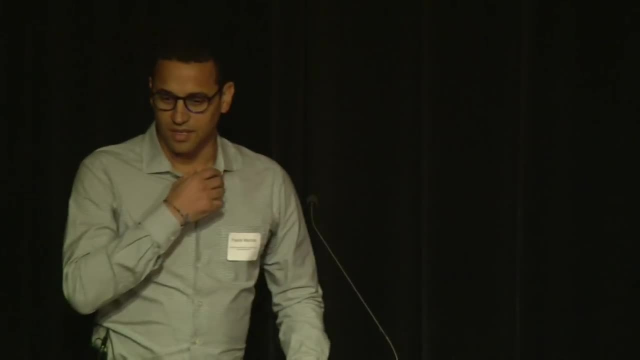 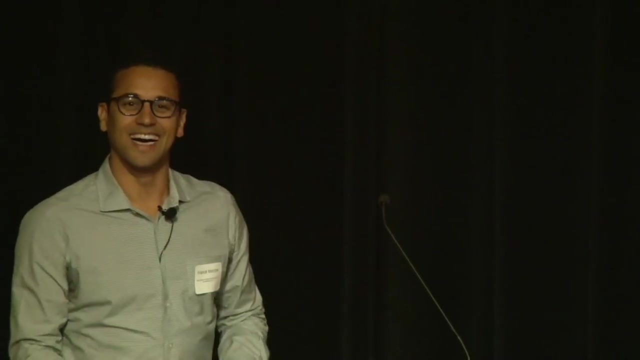 so it's possible, if the skies are clear and you're up that early that you might be able to, you know, get out even around here and a few minutes after launch. see, It was very short, thank you. So I heard that we are kind of slow to start this talk. 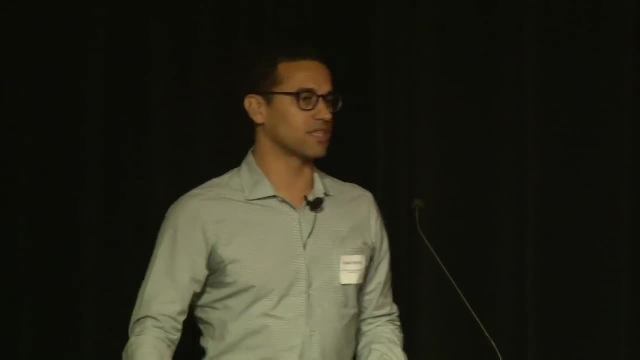 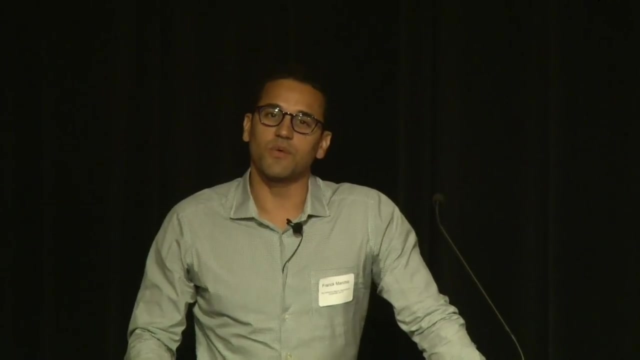 so I'm going to give a very short introduction. My name is Frank Marchis, I'm a researcher at the SETI Institute and I'm going to be hosting this SETI talk today. Today, we're going to talk about how artificial intelligence can help astronomers. 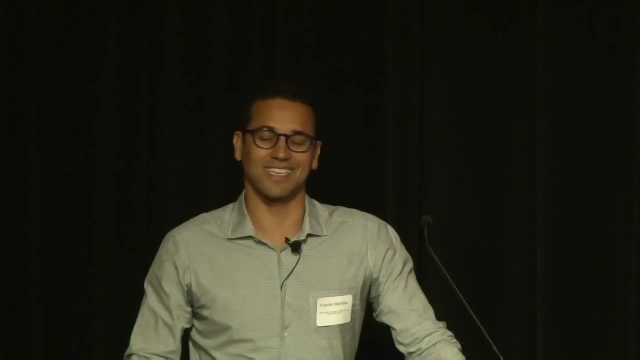 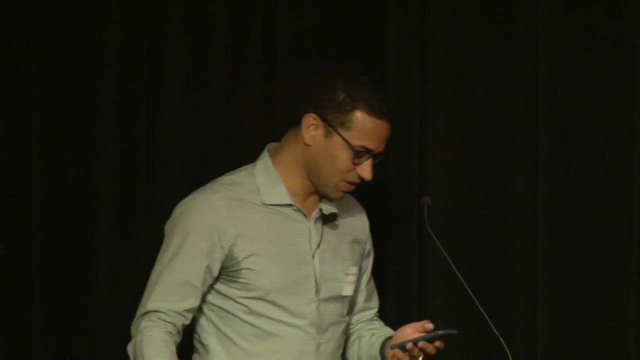 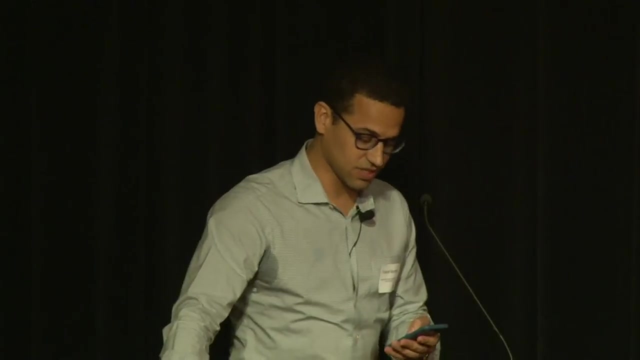 and why we need artificial intelligence in today's modern astronomy, And for this purpose, I invited these two remarkable researchers. The first one is Jeffrey Smith. Jeff is a researcher at the SETI Institute. he's a data scientist at the SETI Institute. 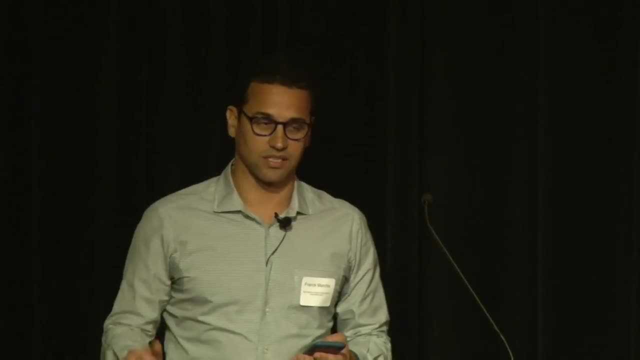 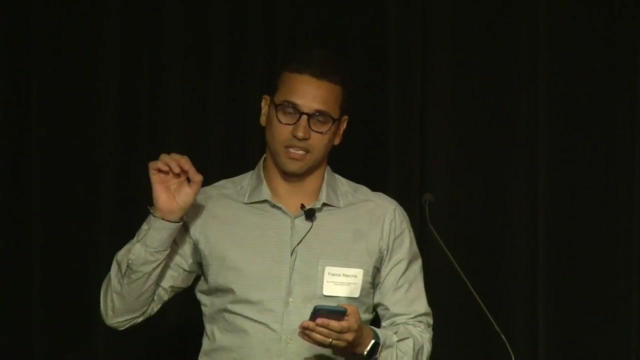 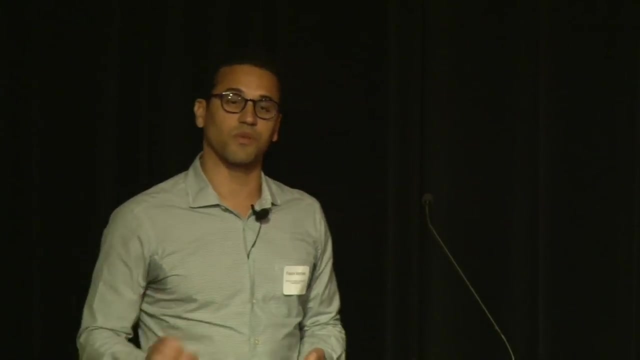 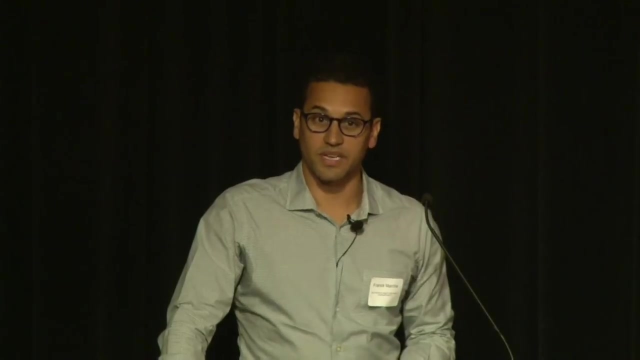 He's basically dedicated most of his career at the SETI Institute to develop pipelines to search for signals of transiting exoplanets in Kepler data. In fact, I discovered today that Jeff did not study astronomy. he studied astronomy right away. He decided first to study the physics of particle accelerators. 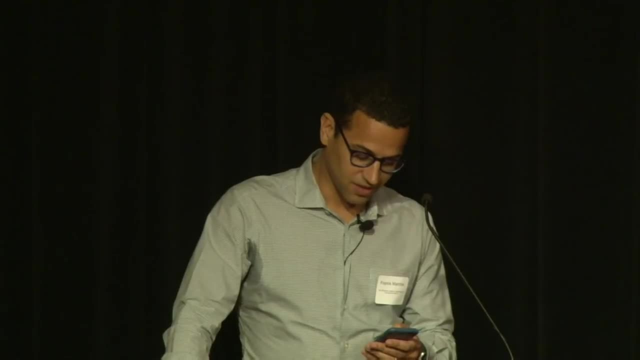 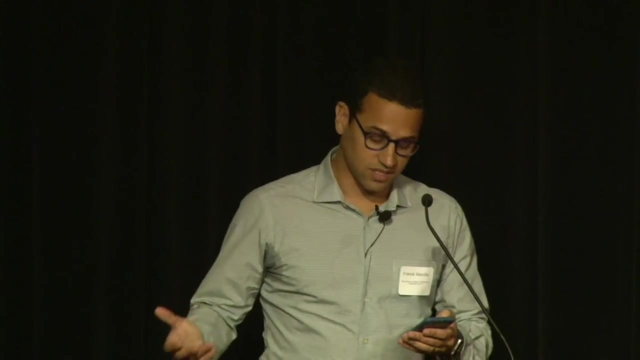 and he did his PhD at Cornell on this topic, specifically on the design of the International Linear Collider, which is a 22-mile long electropositron accelerator that will complement the discovery of the LSC. So, after joining the Institute, Jeff worked on the Kepler data analysis. 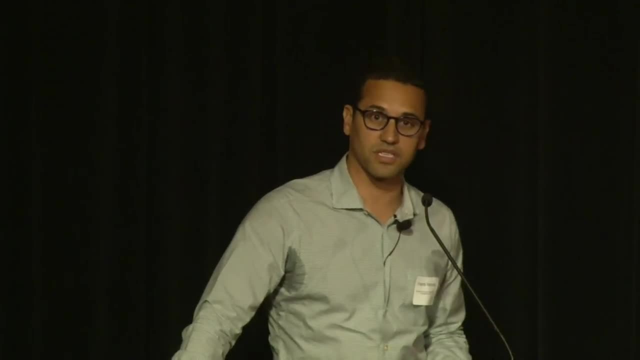 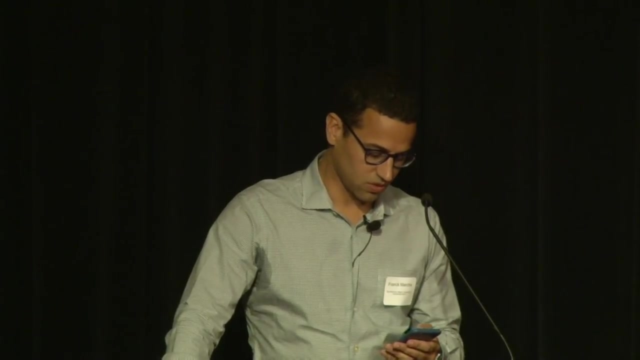 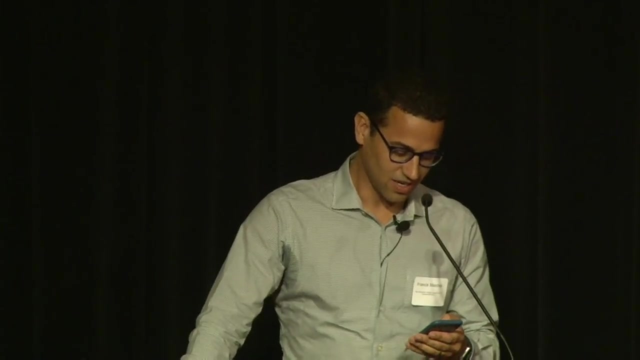 but he's also now very interested in using his expertise to develop the pipeline for the test mission, And he's going to talk about this, of course, during his talk. The second speaker is not an astronomer per se. His name is Chris Shalu. he's a senior research software engineer at Google. 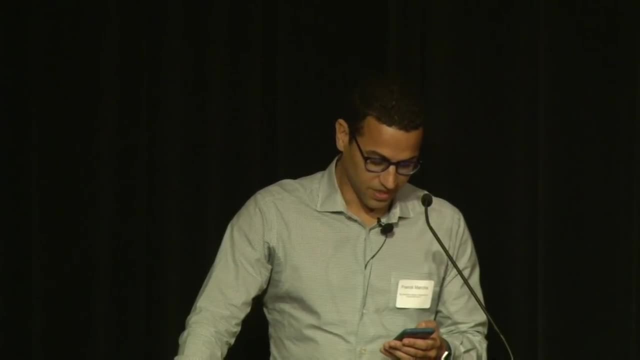 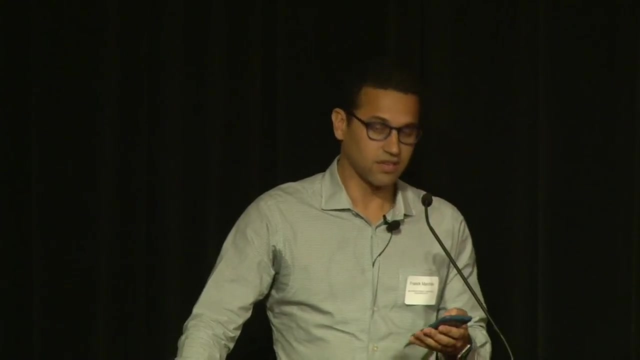 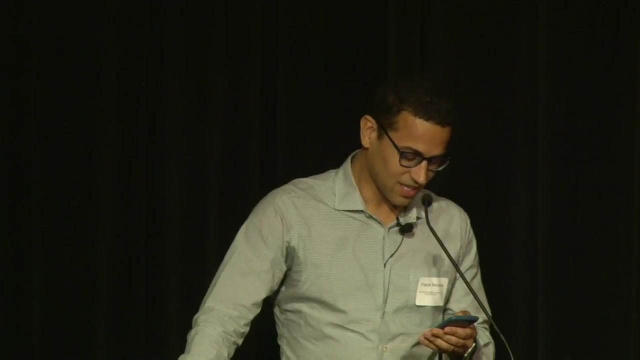 not too far away from here in Mountain View. His research is mostly focused on machine learning techniques for identifying planets in data coming from the Kepler spacecraft, But Chris also works at Google, so he's also interested in using machine learning for plenty of applications. 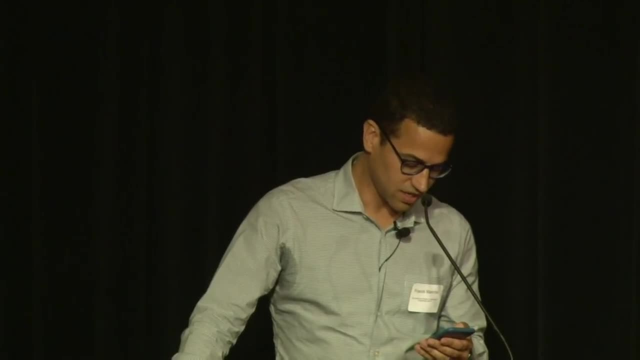 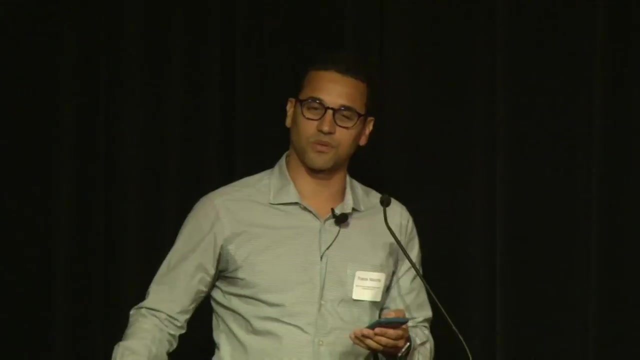 such as image captioning, natural language modeling, and he's also been working on Google Ads. So when you see an ad on the side of your screen, when you are on Google Gmail, that's because of Chris. Thank you very much, Chris. 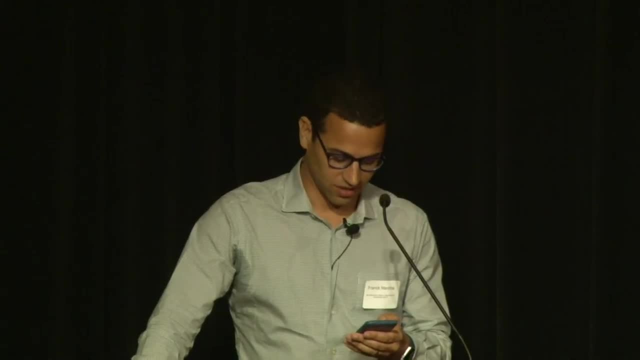 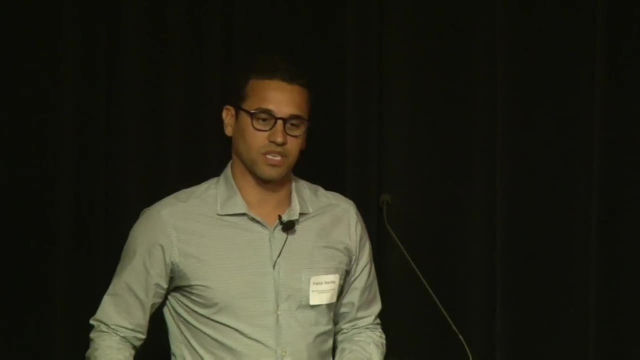 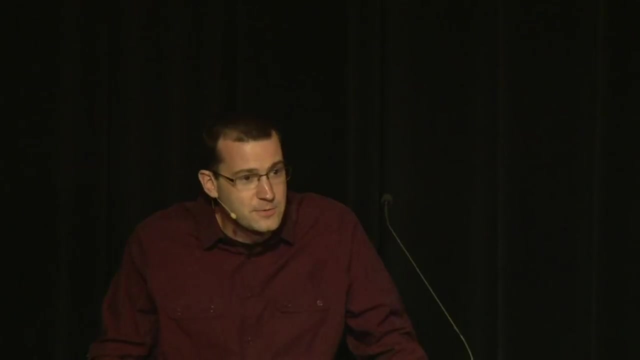 And I should also mention that Chris, before joining Google, was teaching, studying and researching mathematics. So please join me in welcoming our two speakers, and we're going to start with Jeff. Hello everyone. So I'm here to discuss the simple little problem we have. 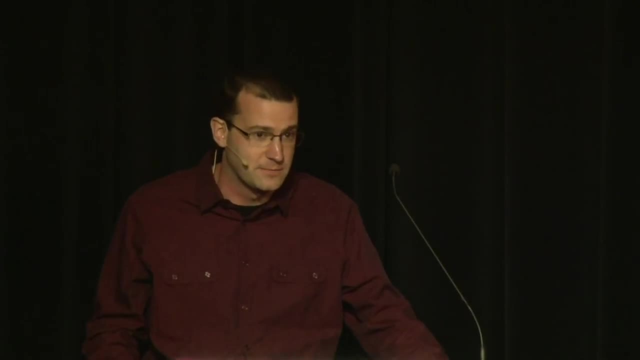 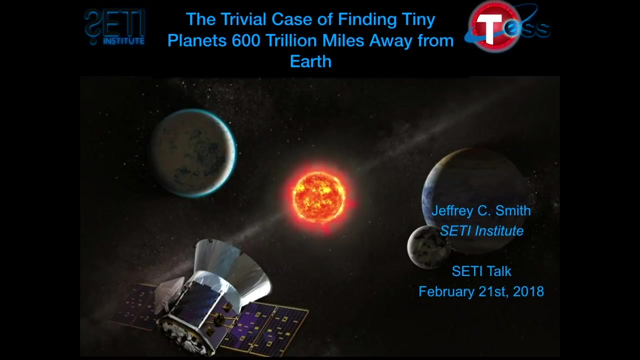 of finding tiny planets 600 trillion miles away from Earth, And this is actually more difficult than it sounds. So I work on the TESS mission. As Frank said, I work on the team that develops the signal processing and transit detection algorithms. Before that, we worked on Kepler, and they're both very similar missions. 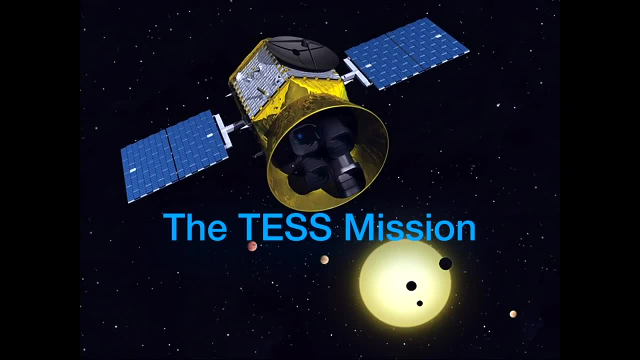 both searching for extrasolar planets, But there are some differences. First of all, TESS is going to launch Right now. the plan is in April. We'll see, but that's the current plan right now And there are many similarities between them. 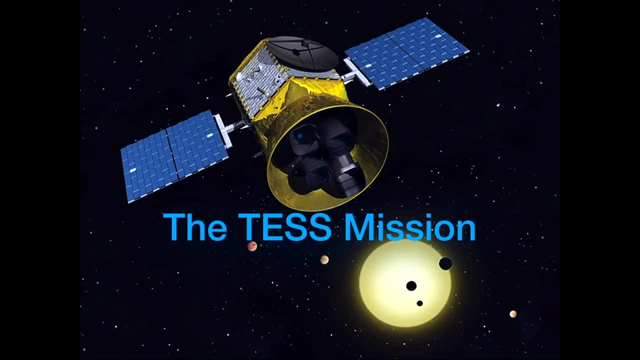 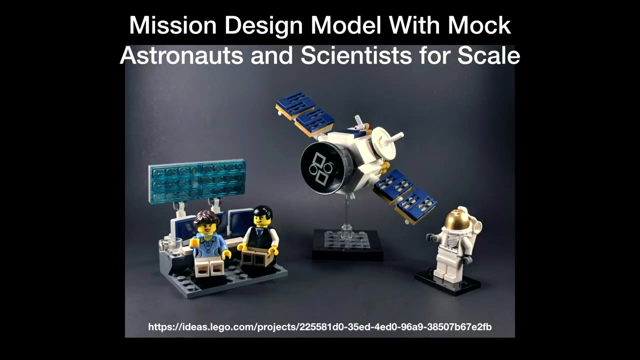 but I'm going to show a couple of the differences. First of all is the size. So this is a NASA mission Design model, Conveniently with mock astronauts and scientists. you can see the scale And it's a little tiny thing. 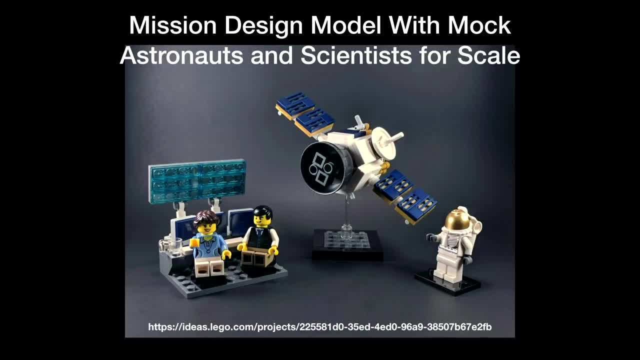 It's about the size of a human. It's about that tall, And this is in contrast to Kepler, which was about the size of a school bus. So it's a little tiny thing. It has four little telescopes in there. Each telescope is small enough you could hold it. 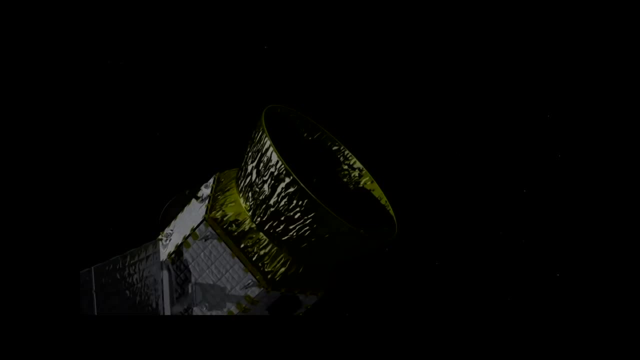 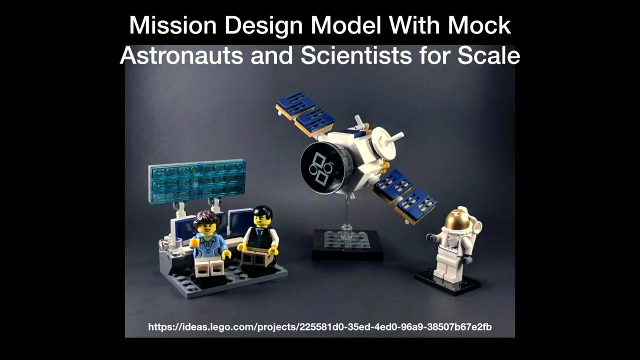 cradle it in your hands. So it's a little thing. However, it's going to be surveying a much larger, much larger section of the sky than Kepler, So this is a short video. As I mentioned, it has four cameras. 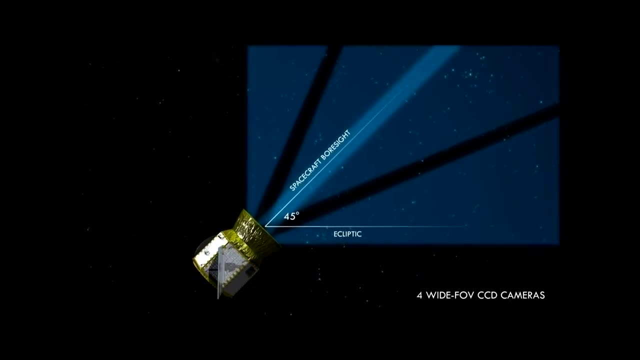 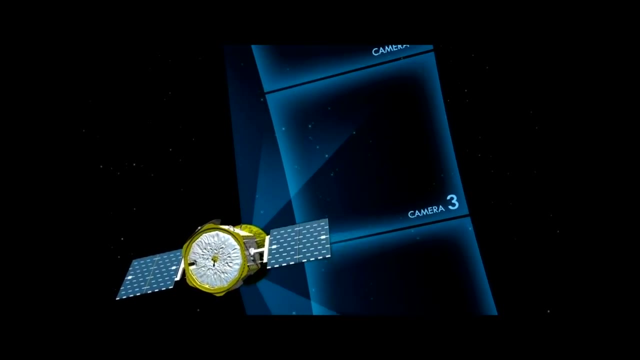 The four cameras are set up in such a way so you can have this huge 90-degree field of view. So at any one time TESS is going to be searching at a 90-degree sector of the sky. It's going to search at that section for about 27 days. 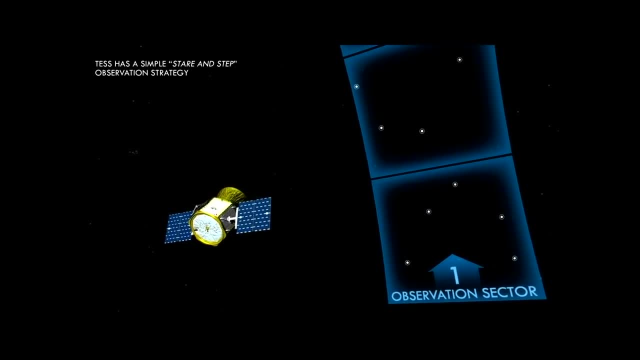 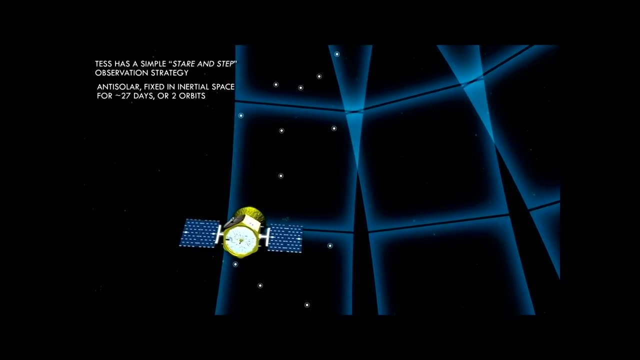 looking at the stars, trying to find planets, Then it's going to rotate. look at another section of the sky, Again for 27 days, Rotate again 27 days Over the course of an entire year. it's going to cover an entire hemisphere. 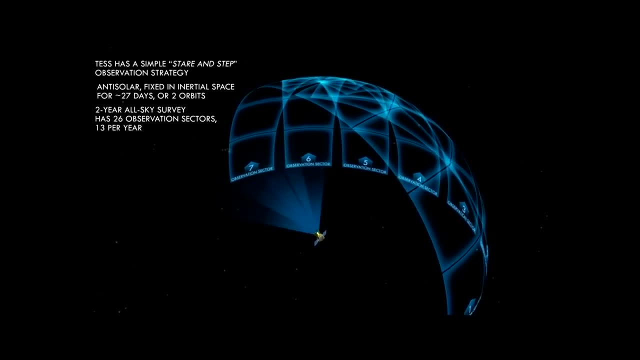 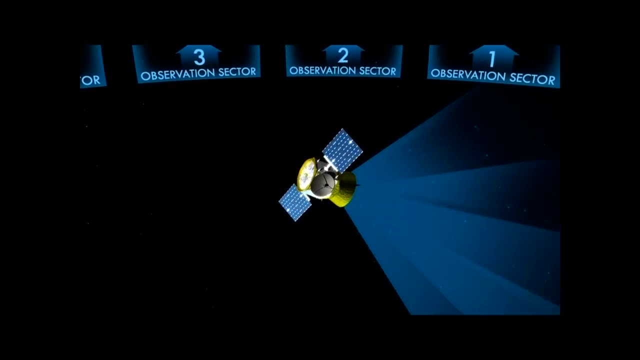 It's going to start with the southern hemisphere of the sky. There's also going to be this region right at the top of continuous viewing zone where it's going to collect data for an entire year. Once it's done, it's going to flip over. 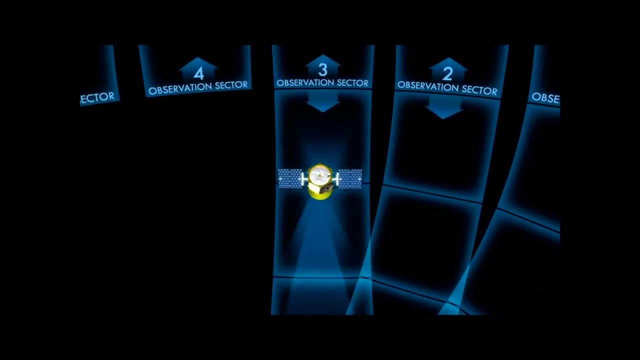 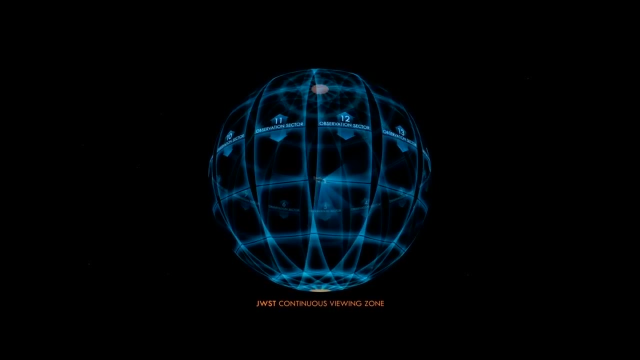 and do the same thing again for the northern hemisphere. Once it's done, it's going to have almost a complete survey of the sky. There's going to be a couple slivers there where it's not going to see things, But for the most part 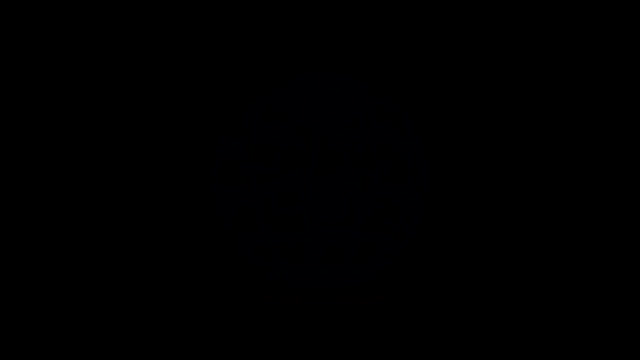 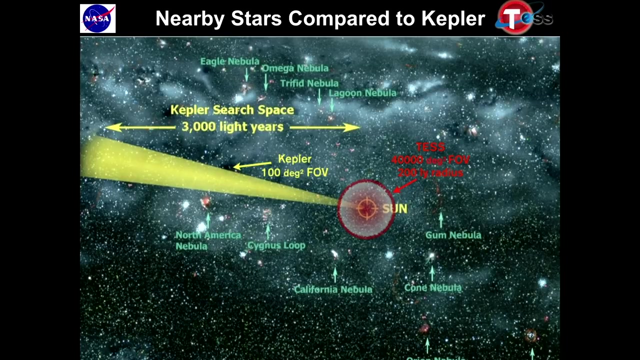 it's going to be a complete survey of the sky. So there is another big difference between Kepler and TESS. Kepler was essentially a statistical mission. It was to calculate the frequency of Earth-like planets in the galaxy, And Kepler has been a resounding success in that regard. 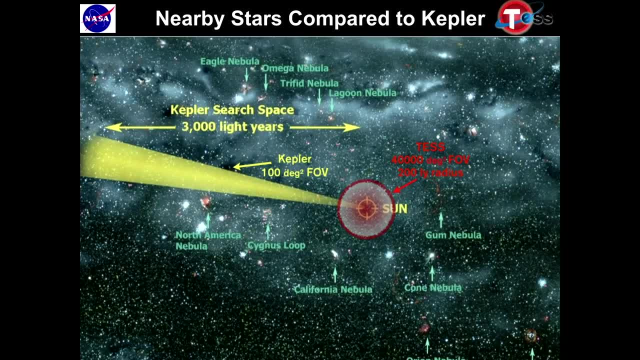 TESS is more of a cherry-picking mission. It's searching for the nearest Earth-like planets- really any planets we can find, but Earth-like are the most interesting- And it's only going to look out tens to a couple hundred light years away. 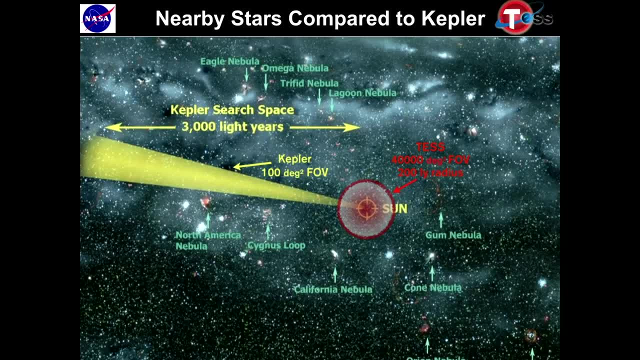 And the critical thing here is that these planets and these star systems are going to be so close, it's going to be much easier to do follow-up measurements So we can measure the mass of these planets and therefore the density, and see if they're rocky planets or not. 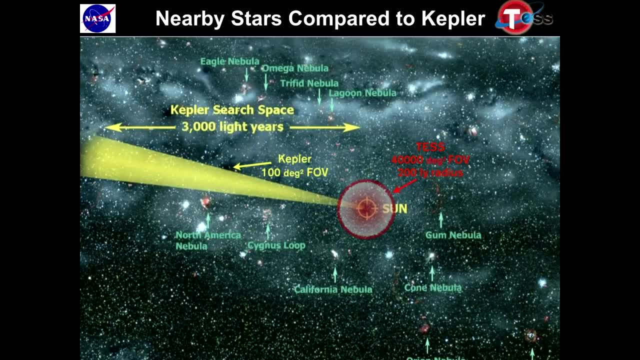 And then eventually we can measure the atmospheres of these planets and hopefully someday detect biosignatures in these planets or in the atmospheres. But before we do that we've got to find the planets. So I'm going to show you a simple video. 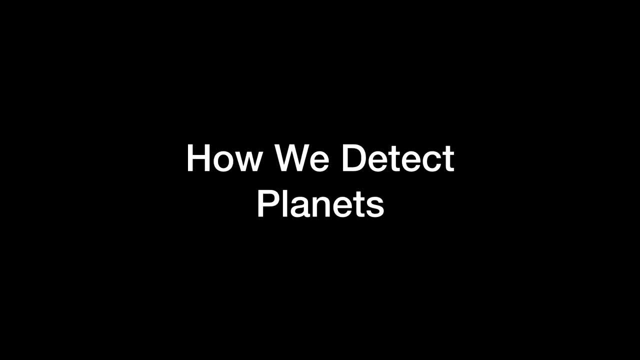 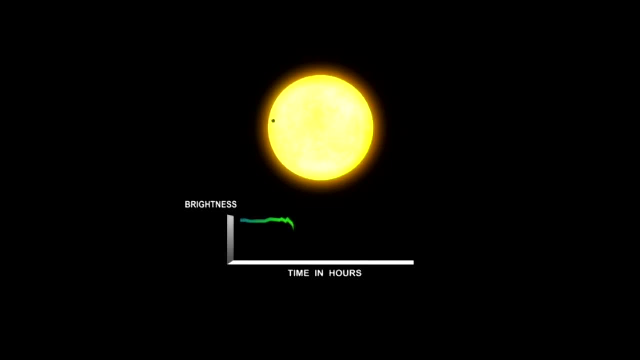 You may have seen this video. It's been around for a while, but it's just a very good video showing you the basic idea of how we detect planets. So you're going to stare at a star and then you're going to collect the entire amount of light. 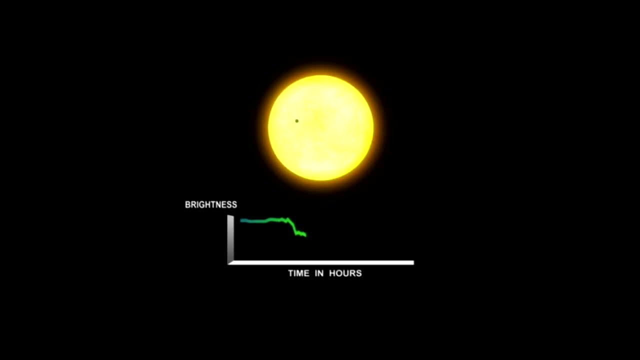 the total brightness from that star. Then, as a planet passes in front of it, as you can see there, the total amount of light or flux from the star is going to dip down a little bit. The depth of that transit is going to be proportional. 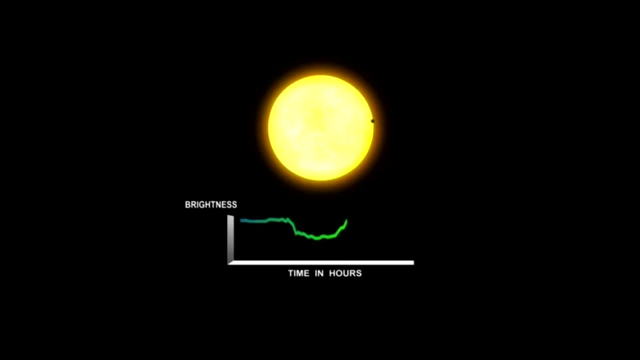 to the ratio of the little planet and the size of the star. So you know the size of the star, you know the size of the planet And then, after one orbit of the planet, if it comes around again, you're going to see another dip. 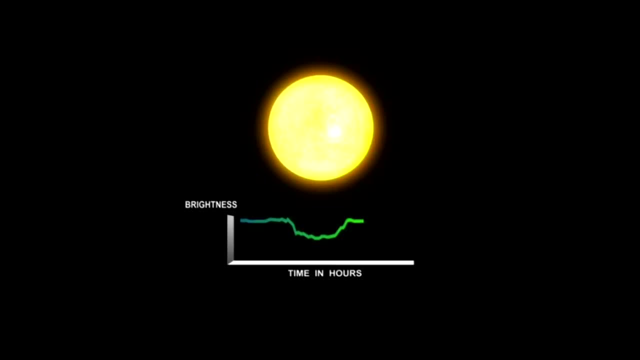 And if you see this periodic dip, that's the tell-tale signal that there's a planet transiting this star. And well, in a way, that's it. That's all we do. Unfortunately, it's a little bit more difficult than that. 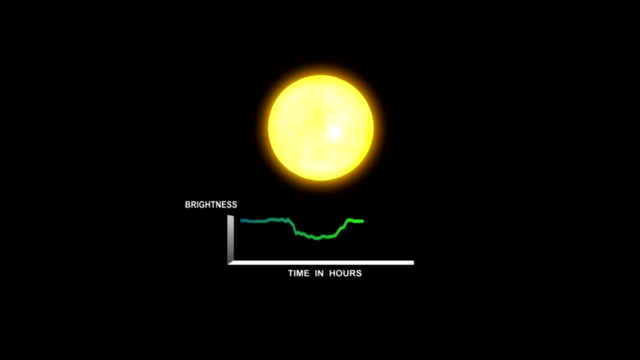 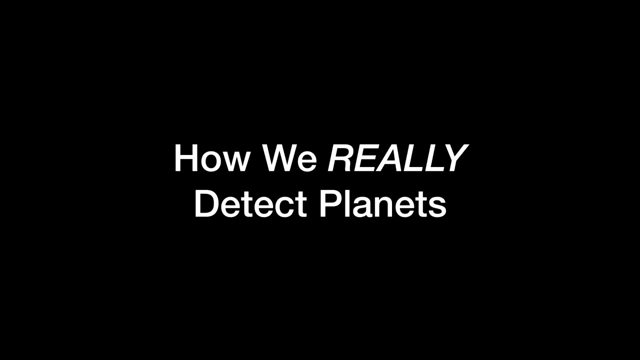 And the reason we're here is to discuss ways that machine learning can aid in the discovery process. So, in order to do that, I'm going to tell you how we really detect planets. It's a little bit more involved, but let's see if I can summarize this. 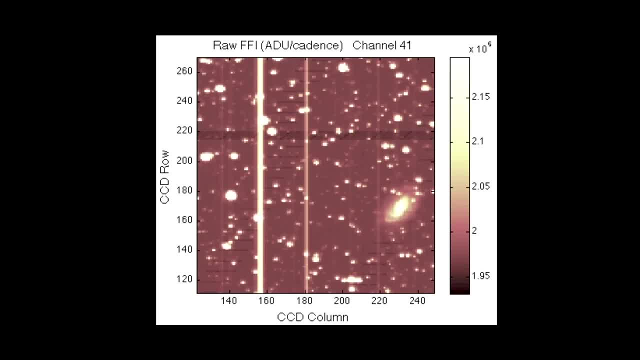 So I'm going to start with the beginning, at least from a data perspective, and that's the CCD array. So, as most telescopes, or many telescopes, you have a CCD array that's collecting the light, And this is a step that's kind of passed over a lot. 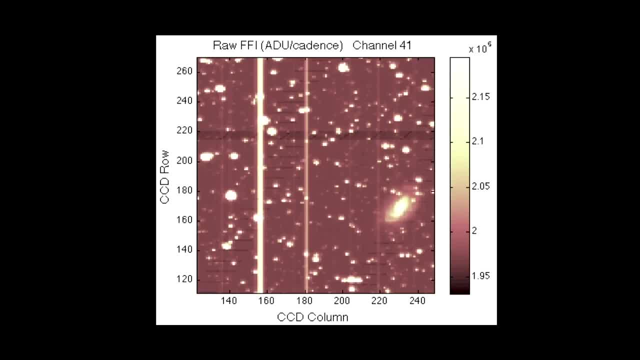 but it's actually absolutely critical. This is a raw image from Kepler. This is a raw CCD image And you see all kinds of junk in there. You see a bleeding star- that's a bleeding current- and the pixels around it. You see video crosstalk. 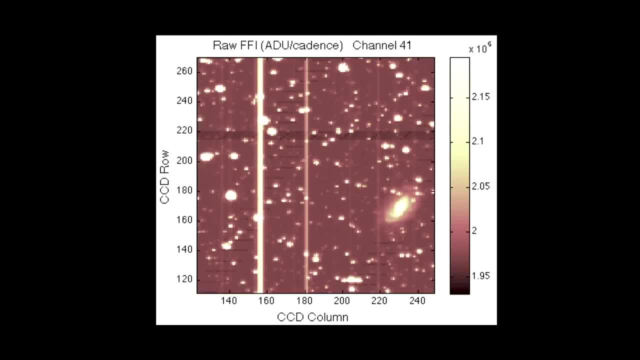 You see issues with readout errors, You see flat fielding errors. There's all kinds of junk in here, And before you do anything you've got to get this out. So I would love to discuss it. It would be an hour-long talk on its own. 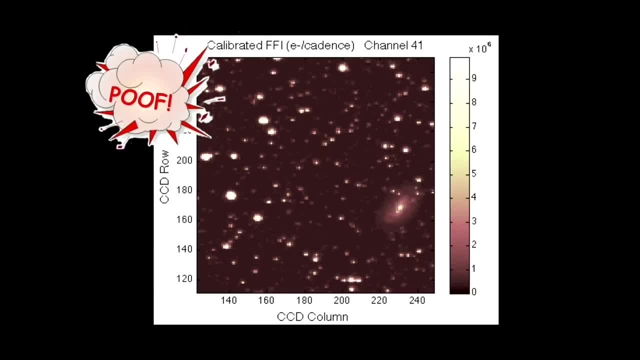 So I'm just going to say poof, and it goes away. Once you do that, you have a nice clear view of the night sky, And now we can actually start searching for things in this calibrated image. But don't forget that. 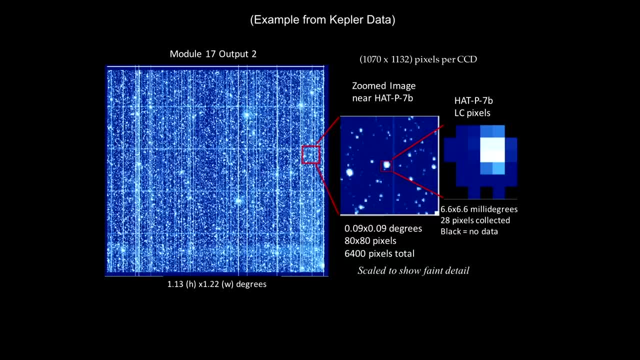 That's really important and it's always skipped over. So now that we're looking at this CCD array and this is real Kepler data- again, There's no real test data because it's not launched yet- We're going to pick some stars in here. 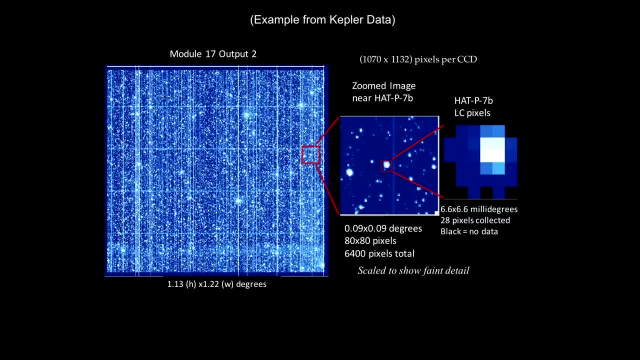 that we really want to look at. and well, that looks like a good one, Let's look at that one. So we're going to pick some pixels around it, figure out what's a good pixels to find, and then we're going to collect. 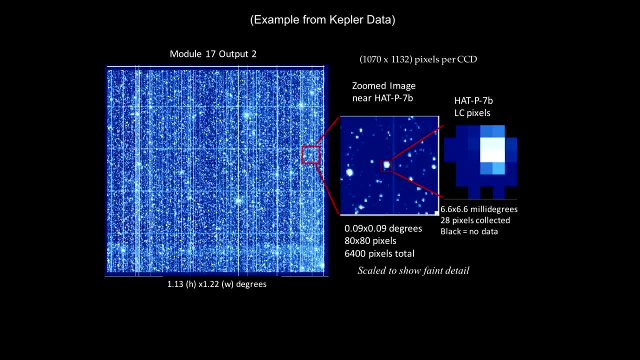 all the light from that star And we're going to create this light curve and we're going to look at it for at least 27 days, if not for a year. We're going to collect this, we're going to bring down the light curve. 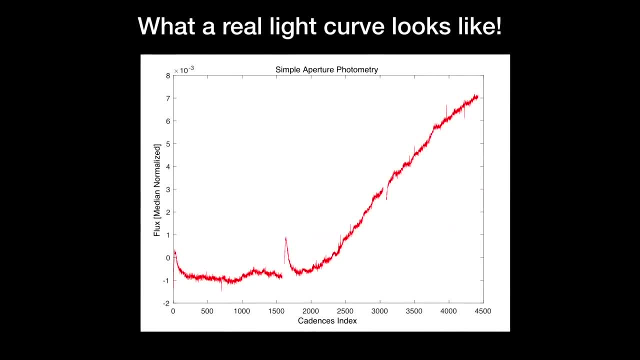 and it looks like that, Not what you want to see. Now, there could be transits in here, maybe, possibly, but they're obscured by all this other crap that's going on. And well, all this crap's actually coming from the spacecraft. 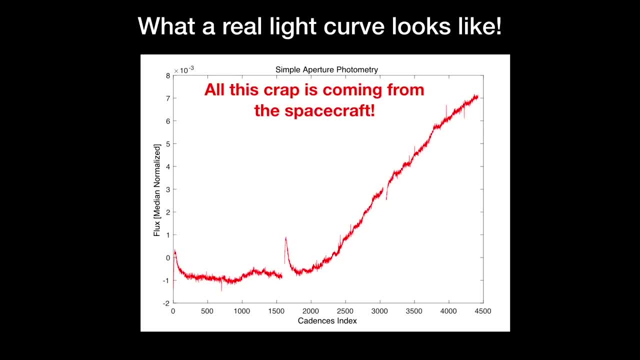 Because when I mentioned that we're staring at a section of the sky and we're pointing, really well, we're not moving because we have really good reaction wheels that do not break, But even so, in reality it's really going like that. 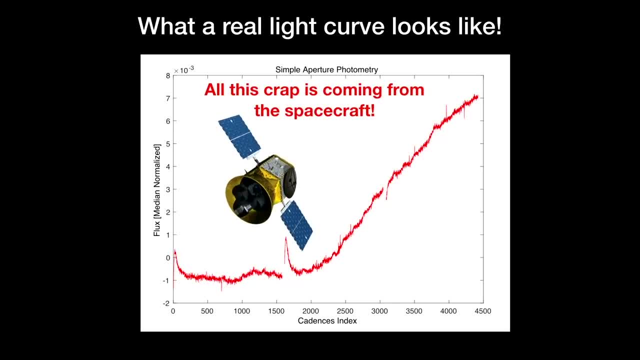 It's shaking around, there's all this stochastic noise and occasionally we're not pointing where we think we are and we have to do an attitude tweak and put it back. And in addition to that, we're staring at a section of the sky. 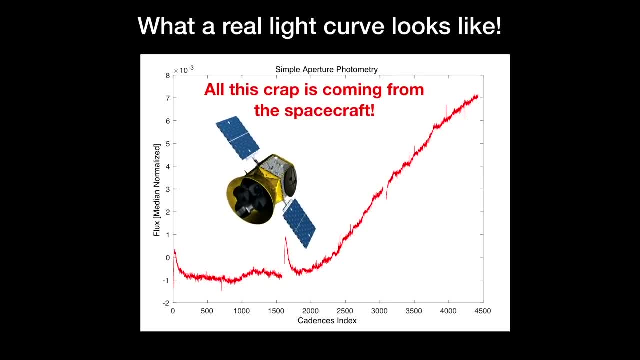 and the sun's moving relative to it. So different sections are heating up and cooling down. so there's thermal expansion and thermal contraction. that causes the optics, the telescope, to expand. So you have focus changes and you get all these long-term drifts. 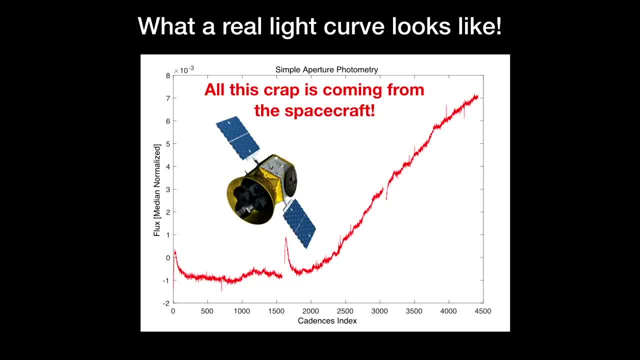 You get something that looks like this, And this is huge compared to the little tiny transits we want to see. Fortunately- oh, this is just a video of it going out of focus. Fortunately, all this crap can be characterized and we can identify what's going on. 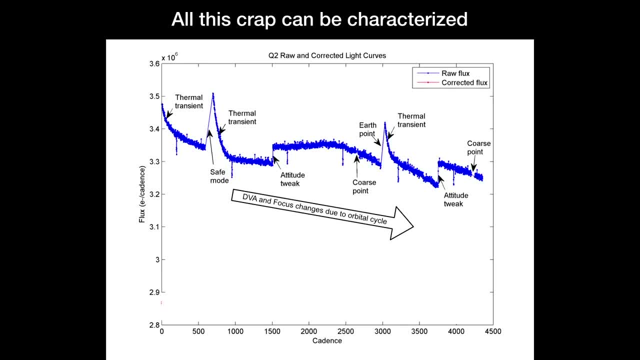 in each one of these cases and we can remove it. We can remove it very well. I would love to discuss it, but we don't have time, so I'm just going to say magic And it goes away. And now we have a nice. 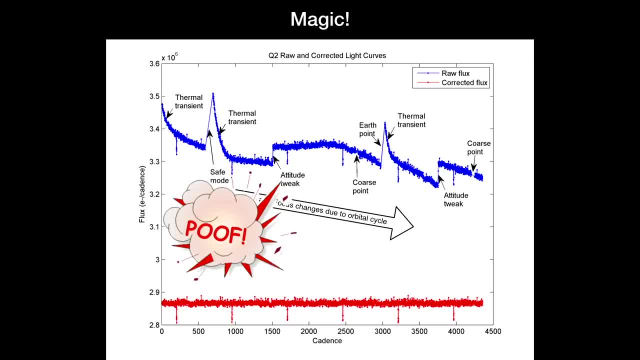 clean light curve and you can see the transits just dangling down underneath it and a discovery right. Well, not necessarily, because just because we see something that looks like a transit doesn't mean it actually is a transit, because the stars are working against us too. 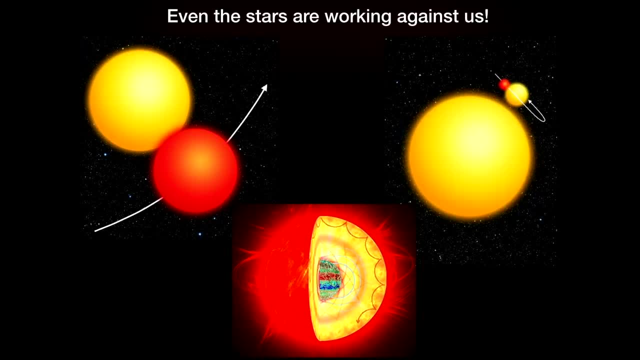 Stars are not glowing orbs in the sky. They're giant fusion reactors and they're pulsating and vibrating, and many of them are giving off flares all the time. And in addition to that, you could be staring at a star and just over its corner. 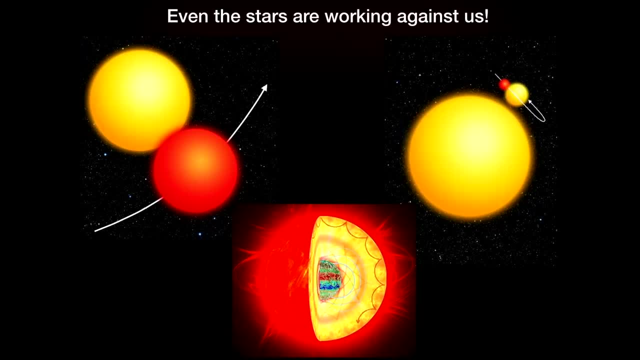 there could be an eclipsing binary, because binary star systems are all over the place And you can't resolve that from the star you're looking at. so when you look at the total light curve, it looks like there's a little tiny Earth-like transiting planet. 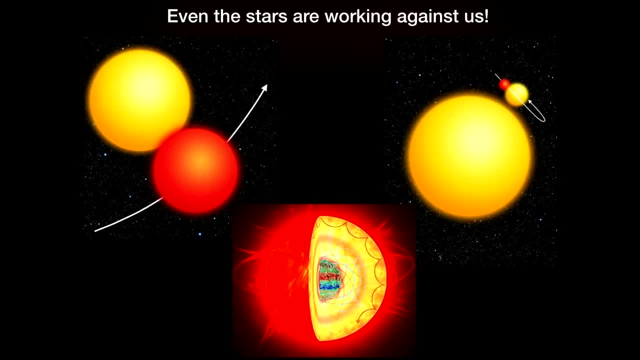 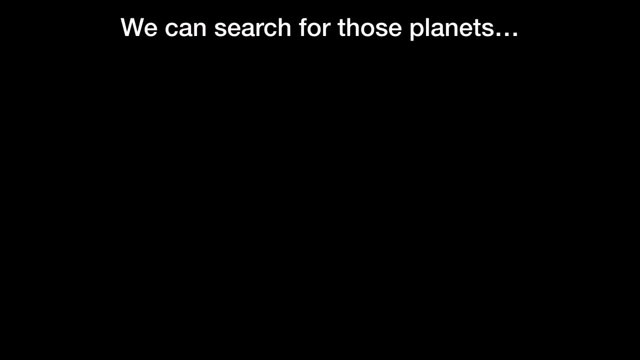 but it's actually a giant star that's eclipsing away in the distance, So you've got to know very well what's going on in the sky around what you're looking at. So, in summary, we can search for planets and we can search for Earth-sized planets. 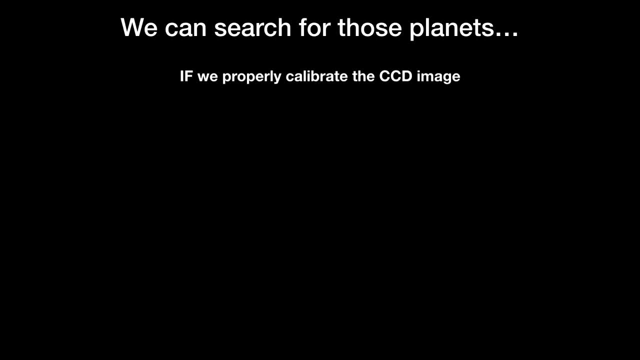 but only if we properly calibrate the CCD image, if we properly collect all light from each star, if we properly remove all instrumental artifacts in the light curves and if we properly account for all stellar objects around each star and know how they are behaving. 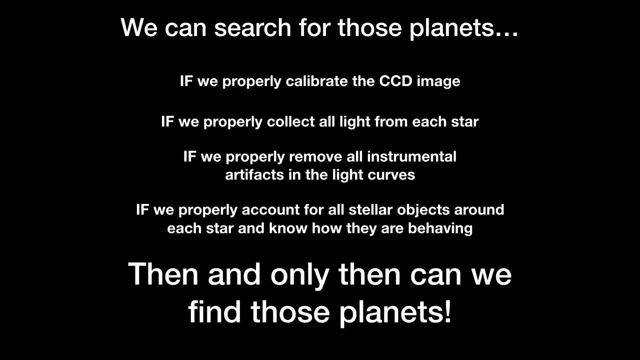 Then, and only then, can we actually find the planets. And even though we're really good, we don't necessarily always do this right and sometimes you get little residual artifacts in there that look like planets and they're really not, and that's a challenge. 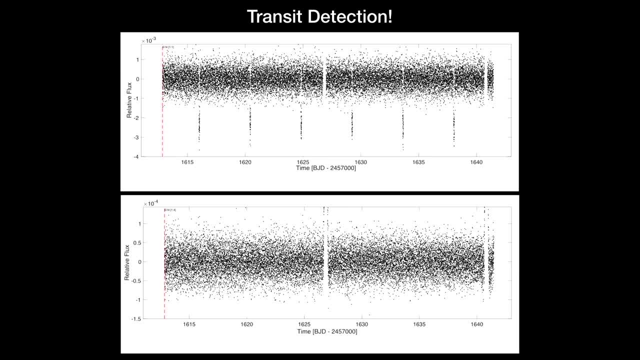 But say that we can remove all of this and you're going to get a light curve, something like this, and you can see the nice transits dangling down and again, if that's all it was, we can all go home. We can do this. 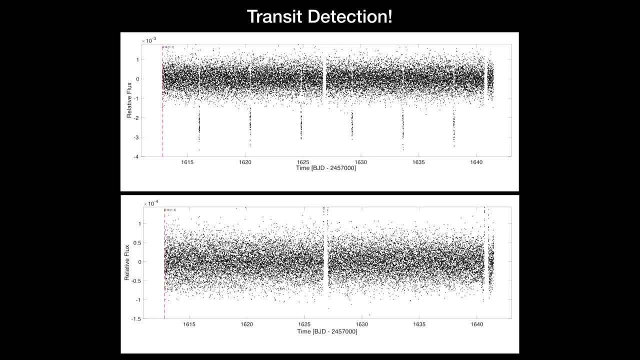 The problem is the Earth-sized planets. the interesting ones make a light curve like that, And this is simulated test data. There's an Earth-sized planet in there. I can't see it. I'm guessing you can't either. Fortunately, there are rather sophisticated algorithms. 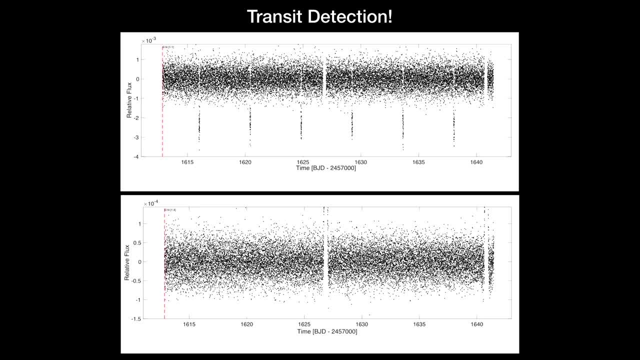 that can detect these little tiny weak signals. I would love to discuss it, but we can't. I'm just going to say we can detect them And there they are, and I bet you didn't guess there were that many in there. 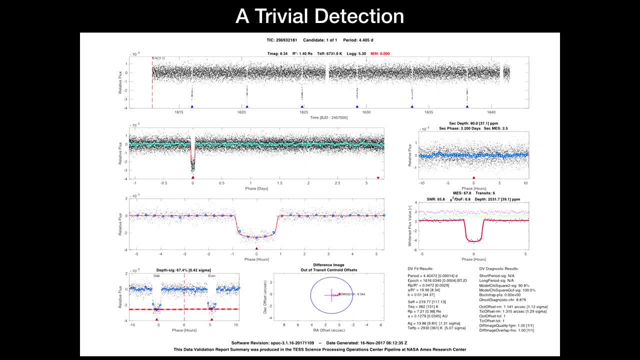 So we process all this data in the test pipeline, just like Kepler, and we develop these huge reports with all this information in it. I'm not going to explain all of this, of course, but we can characterize the transit and we can fit this red line to it. 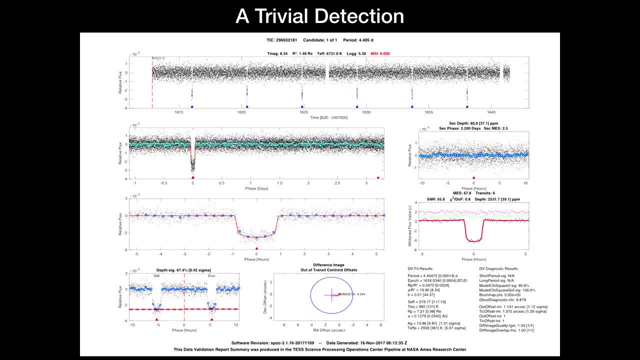 and think we have an idea of what it is. And again, if all the transits look like this, there'd be no problem. This is simple. The problem is the interesting ones look like this. Here's a light curve simulated test data. 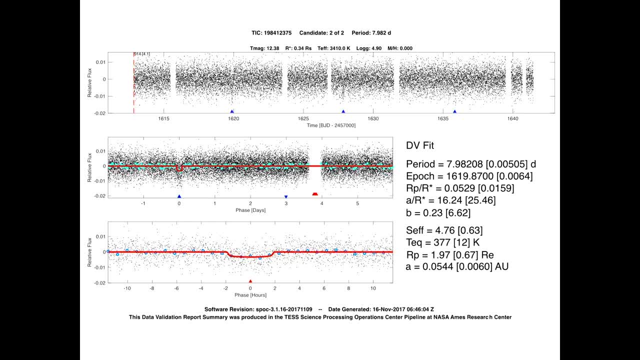 and the pipeline detected three transits and if you phase-fold at the right period you can net transit. Well, okay, it kind of pops out And the pipeline says: this is about a 2-Earth-radii planet, 377-degree equilibrium surface temperature. 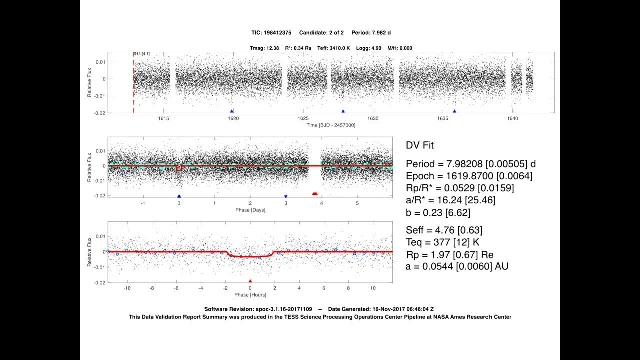 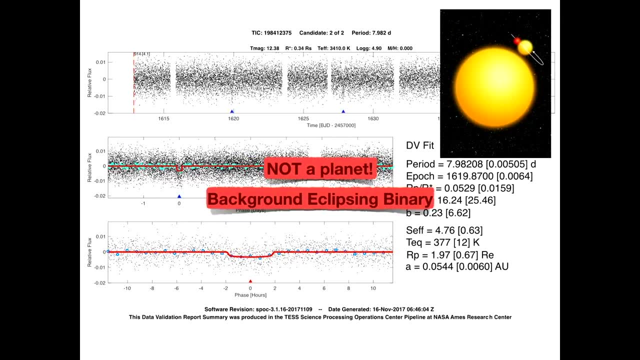 And so is it. Is this really a detection? Well, in this case, it's not. This is just a background eclipsing binary. This is just one of the things I was talking about before, So forget about that one. Here's another example. 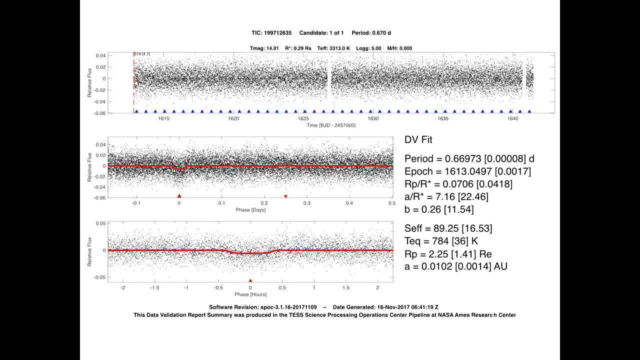 Detected lots of transits. We phase-fold it and yeah, okay, you can kind of see something there. Pipeline again says about a little bit over a 2-Earth-radii planet, radius planet. Is this real, This one's real? 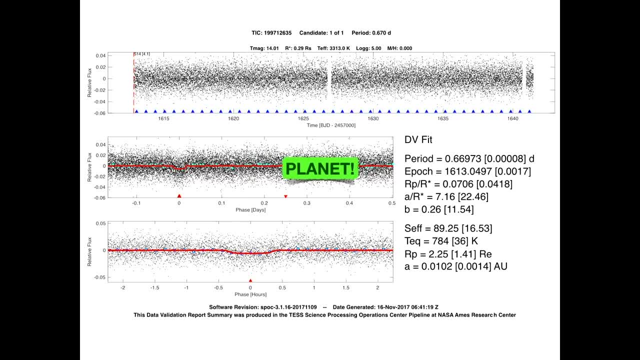 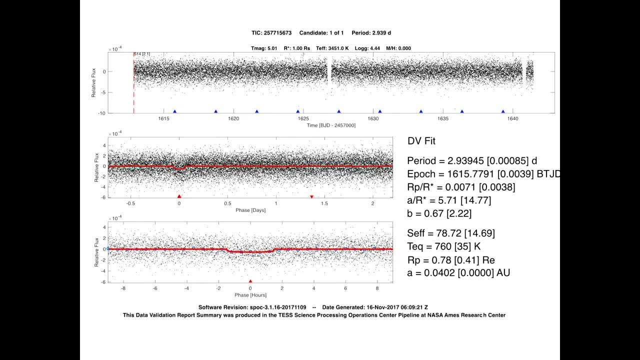 This is a planet. This is a successful detection. Here's another example. Looks very similar to the one I showed before. You can barely see any types of transits. No type of signal there whatsoever. Pipeline says it's a 0.78-Earth-radii planet. 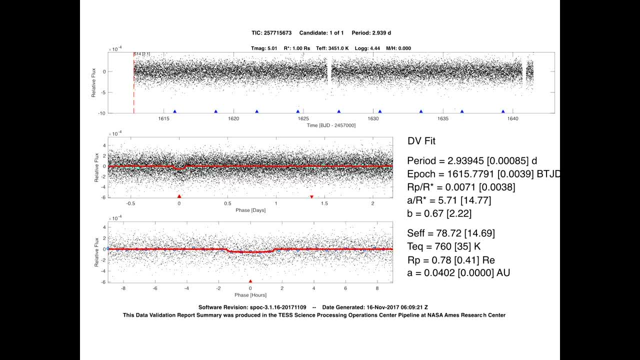 This is smaller than the Earth. This is a paper. It's not a paper. This is random noise. This is just chance correlations of the data. There's not really anything there. Here's another example. Looks just like the previous one. 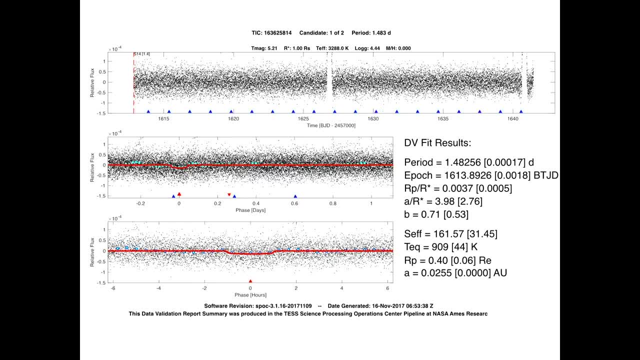 Pipeline says this is a 0.4-Earth-radii planet, but it can't possibly be. This is just noise again, right, This is a planet. This is a successful detection. This gives you an idea of the challenge we have here. 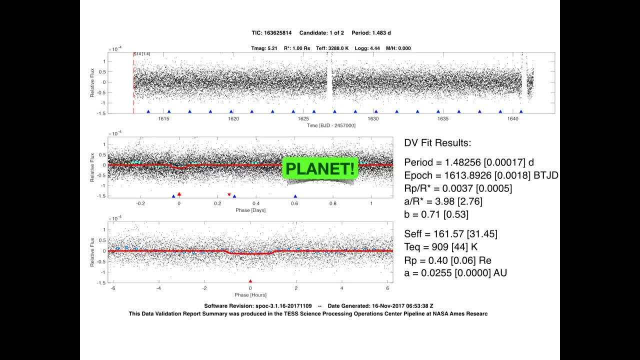 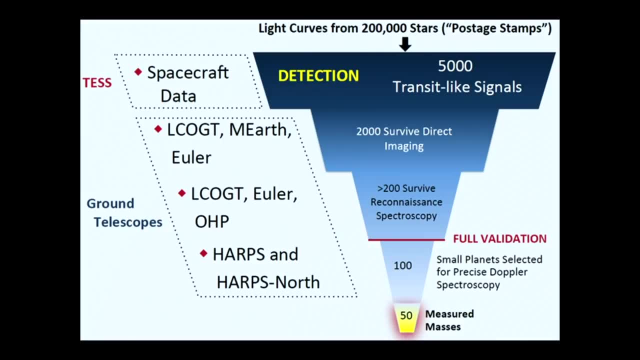 We have all this data, We collect all these signals. Then we've got to figure out what's real or not. Every 27 days we're going to be collecting all of these signals. Then we've got to vet these, We've got to classify them and figure out what is interesting enough. 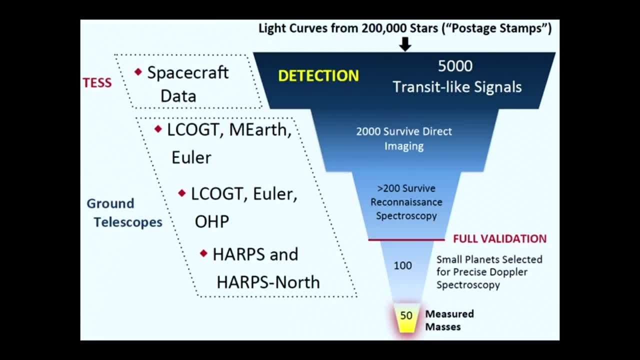 to do follow-up measurements, ground-based measurements, to confirm that they really are planets and which ones are just junk. The thing that's going to make this more difficult for TESS and Kepler is that we've got to do this every month. 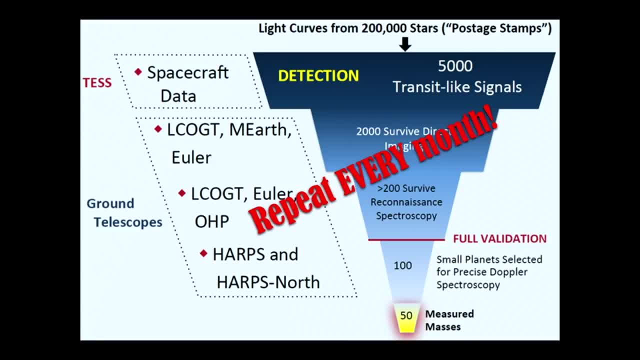 Kepler. we collected data for four years and we've been analyzing it ever since. Every month. we want to do this and find what are real and what are just some other artifact in the data. On that note, thank you very much. 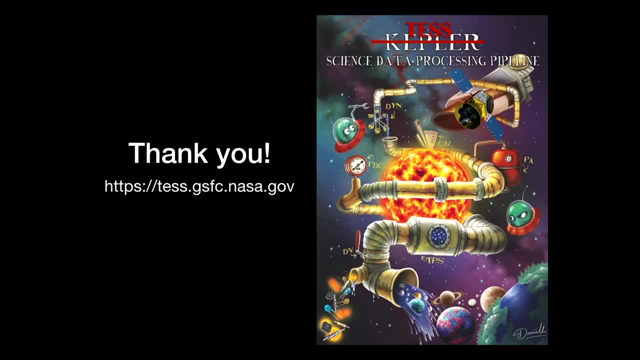 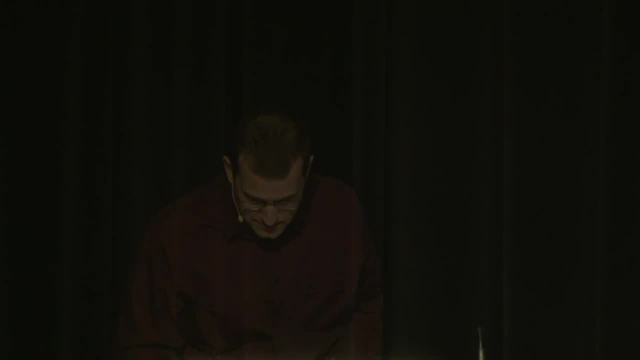 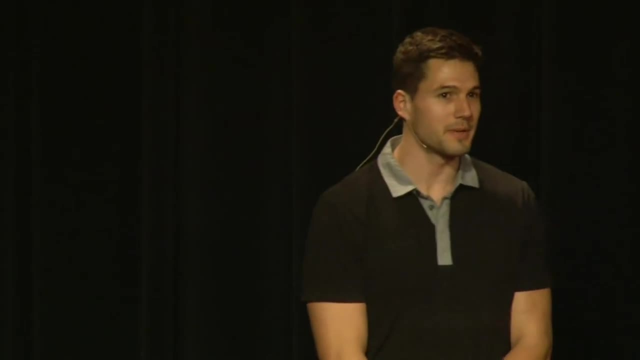 I want to pass the mic over to Chris to give you an example of a particular machine learning method that helps in this exact problem. Thank you very much. Hi everyone, Since the topic of tonight is searching for exoplanets with AI, I thought it would be a good place to start. 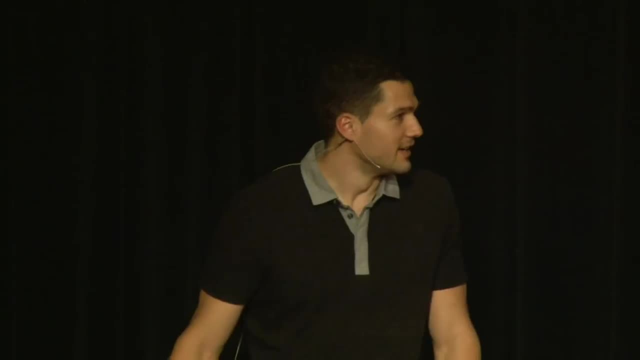 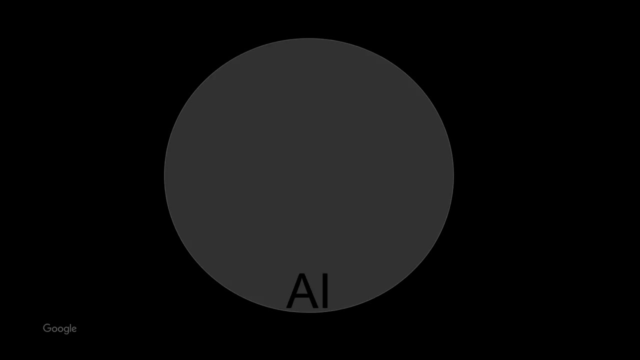 by asking: what exactly is AI? AI is simply a term that means making machines smart. There's lots of ways we can do this. I could write a computer program that would be very good at playing tic-tac-toe, for example. I could do that by just programming in: 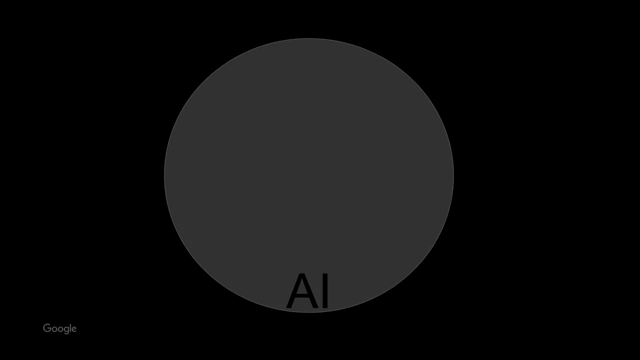 what move to make at every possible position on the tic-tac-toe board. But, on the other hand, another approach you can take to AI is machine learning, which is a set of techniques that allow the machine to actually learn rules for itself from data. 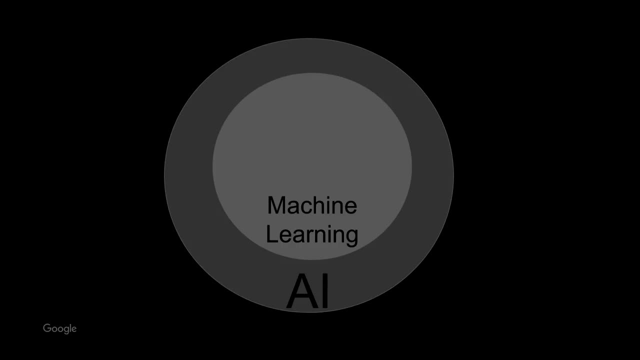 as opposed to humans programming in the specific rules. Now, there's many different approaches to machine learning, and I won't go into them all today, but there's a particular type of machine learning that I focus my research on, and that's called artificial neural networks. 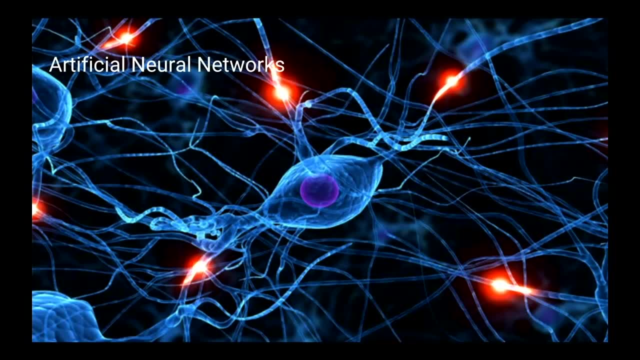 So what is an artificial neural network? Have we successfully recreated the human brain? The answer is no, we have not, although the media sometimes like to run with that angle. The reason for the name artificial neural networks is because the technology actually did. 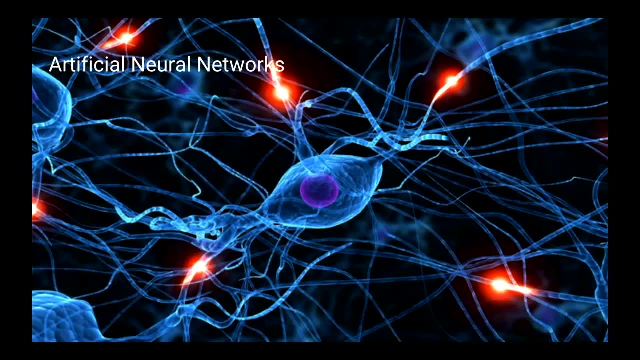 originate back in the 1940s as a method to actually study and try and understand the human brain. But more recently, in computer science, we've actually been using these artificial neural networks not just to study or replicate the brain, but to solve a host of other practical tasks. 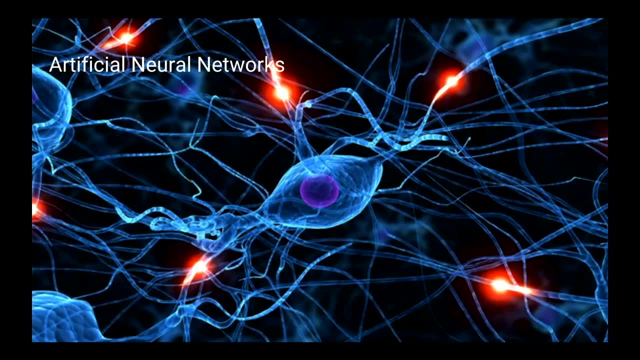 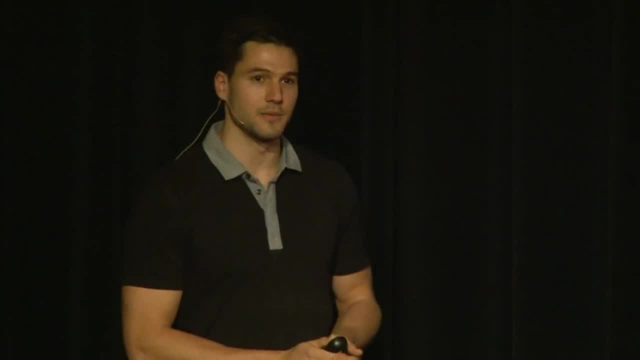 So artificial neural networks I mentioned, they sort of the research sort of began in the 1940s and for many decades it was sort of a niche area of research up until about five or six years ago when suddenly the interest really took off. 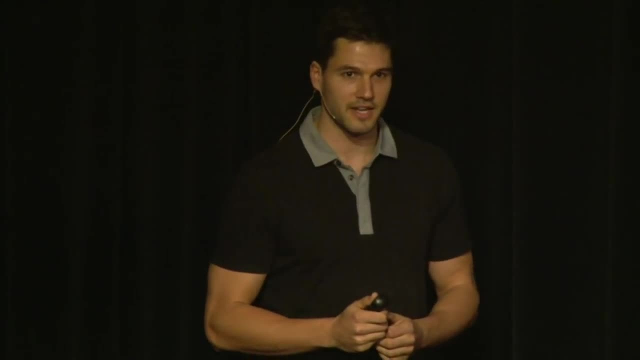 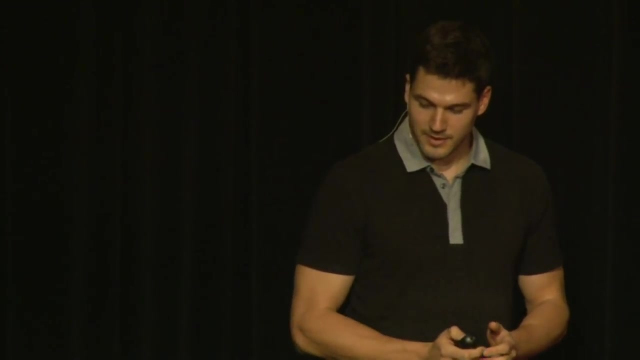 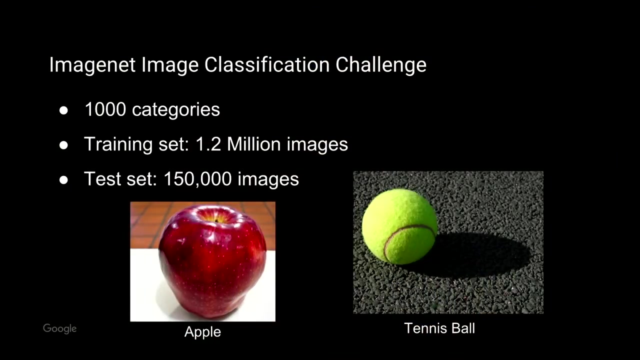 and now most of the tech companies here in Silicon Valley have entire research departments devoted to artificial neural networks. So what happened? Well, the story is best explained through the ImageNet image classification challenge. So this is a yearly challenge run by the computer vision group at Stanford. 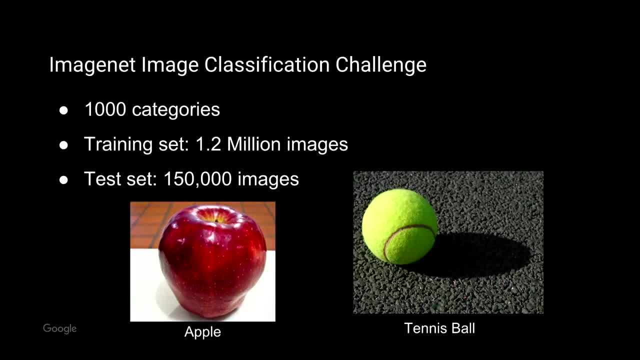 and some other groups as well, And the challenge is they're going to give you a training set of 1.2 million images, And these images are going to be things like apples and tennis balls. There's a hundred different categories that these images could be in. 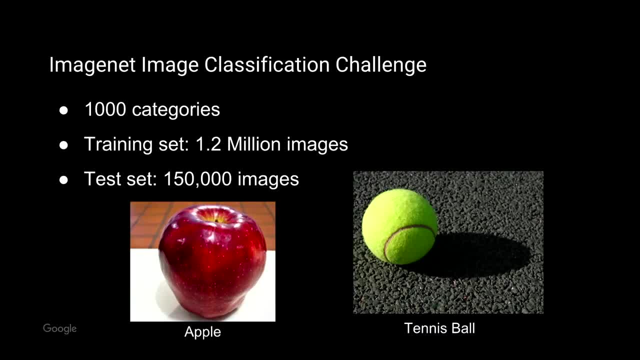 And your challenge is to use these 1.2 million images to train some sort of model to successfully label new images. There's 150,000 images that you don't have the labels for, And so the challenge is: who can train the system? 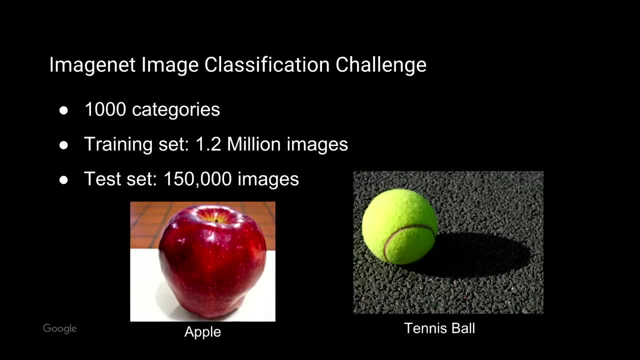 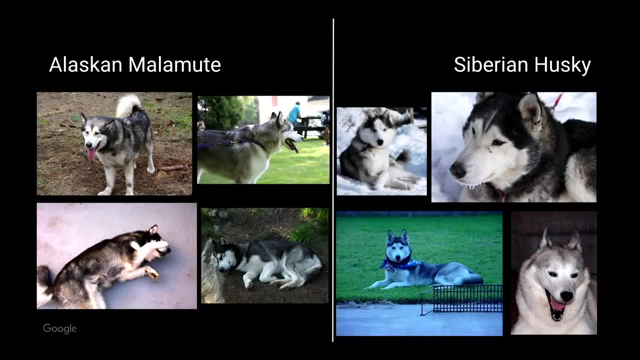 to achieve the best accuracy on these 150,000 images. And so, before you think this problem is too easy, here is an example of two of the classes in this training set: Alaskan Malamute and Siberian Husky. They look very similar to me. 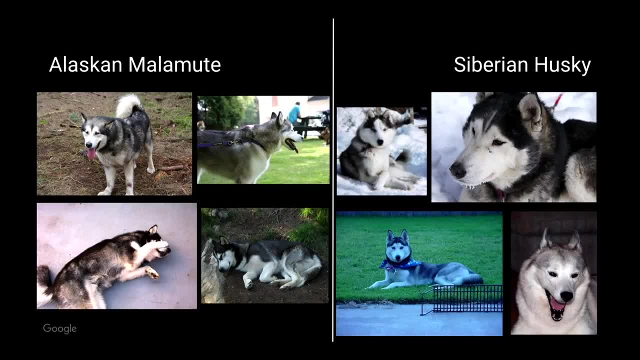 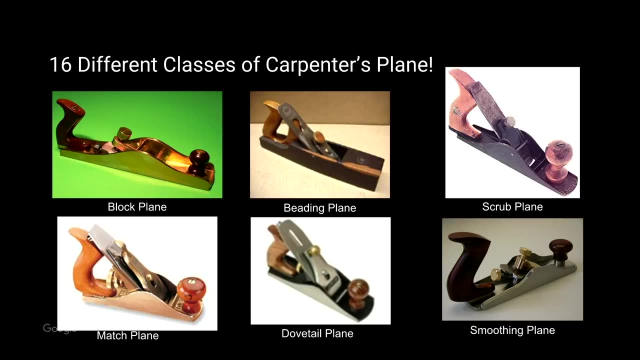 but these are two different classes And you'll notice that the dogs are in all sorts of weird poses and positions and different backgrounds, And additionally there's 16 different classes of Carpenter's plane in the data set. These all look very similar to me. 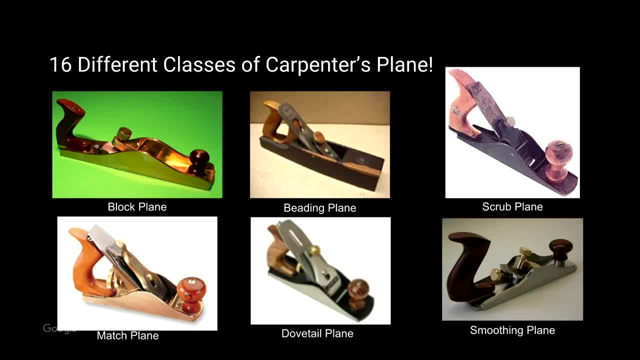 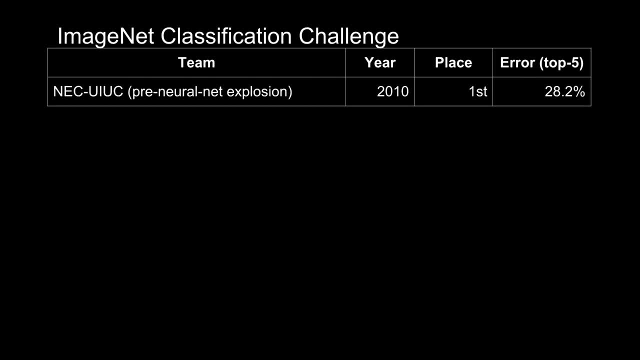 but they're all very different categories So it's quite a challenging task in computer vision. So the very first year of this challenge was 2010,. and this was September 2010.. So it was just over seven years ago. 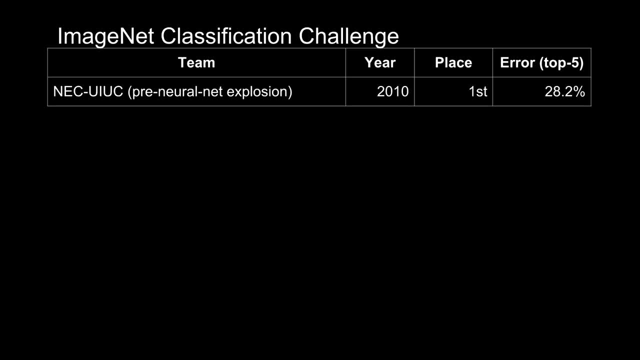 which is generations ago in the machine learning community. So this was before neural networks really had their recent explosion- And the winning team got 28.2% error. This is top five error because under the rules of the competition, each system gets five guesses for each image. 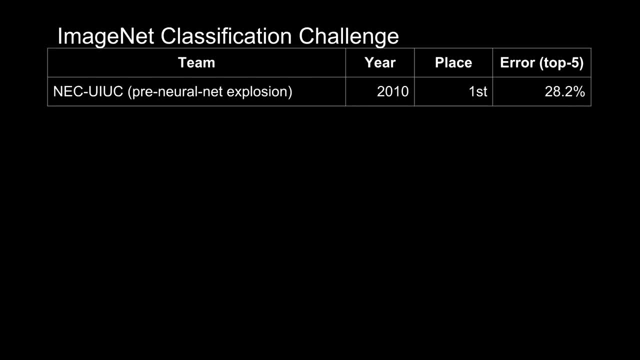 because sometimes there could be multiple images or multiple different objects in each image. So in 2010,, the winner got 28% error, And then in 2011,- this is still before the neural network explosion- the winner made some improvement. 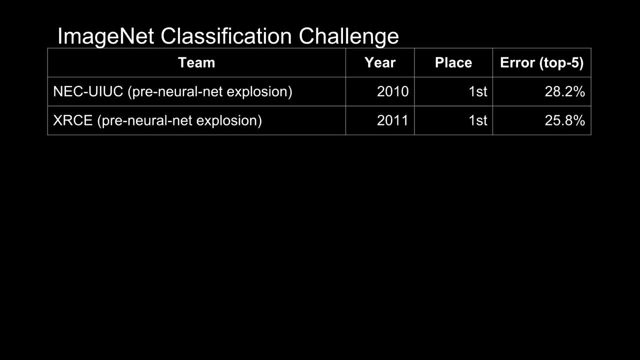 and got 25.8% error, And then 2012 came along- So this is just over five years ago- And this paper came out. It's called AlexNet And this was a neural network that cut the error down all the way down to 16.5%. 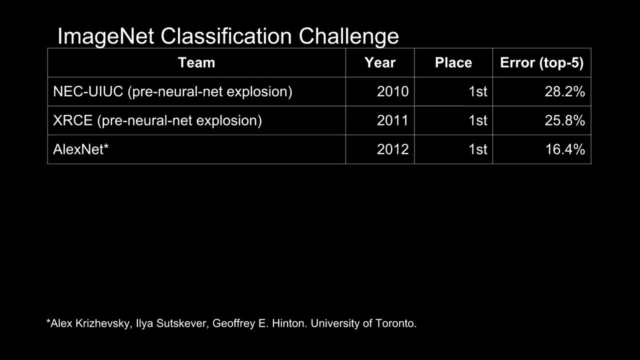 to 24%. This was work done by Alex Krzyzewski and others at the University of Toronto. That's why it was called AlexNet. This really fueled this revolution in machine learning that made neural networks become really, really popular, And so since 2012,. 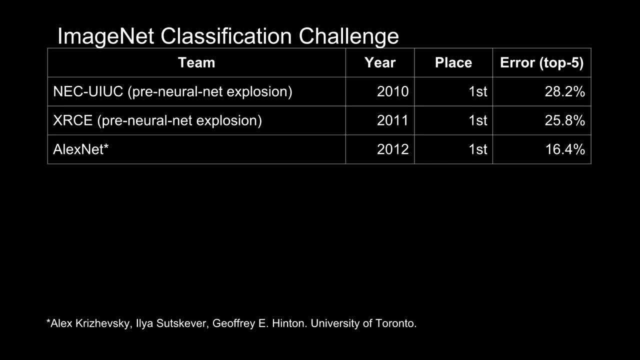 the winner of this competition every year has been a neural network, And so what happened? Well, in 2013,, the next neural network came out that cut the error down to 11.7% 2014, 6.7%. 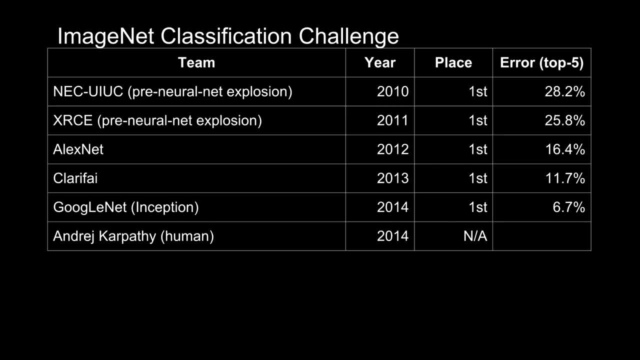 And at this point someone named Andrej Karpathy decided to see how well a human would do at this challenge. So he wrote a very entertaining blog post about this. but he actually sat down and trained himself on these 1000 categories. 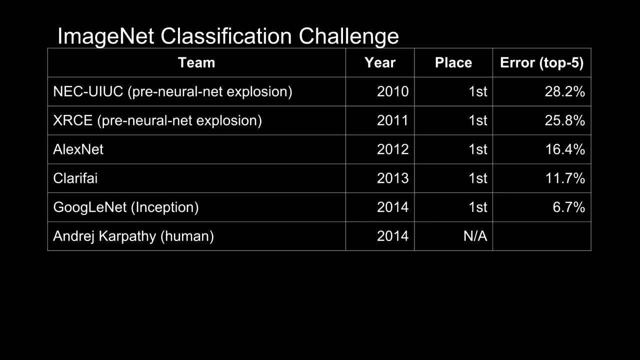 There's like 120 different species of dog, 16 types of carpenter's plane and so forth, And he managed to get 5.1%. So it was a win for the humans until 2015,, when the next model came out with 3.4%. 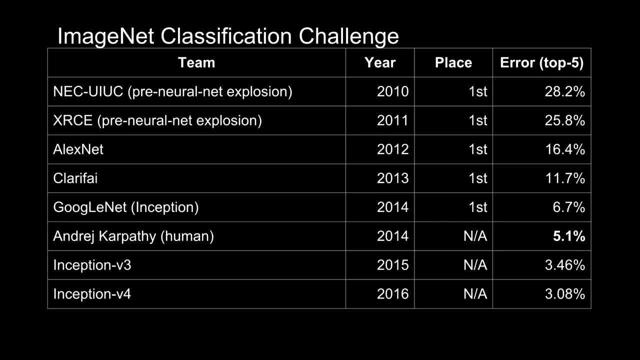 And then 2016,. 3.08% And finally last year the error came down to 2.25%. So in the past seven years, this is the sort of progress that has been made in computer vision, And it's been driven by neural networks. 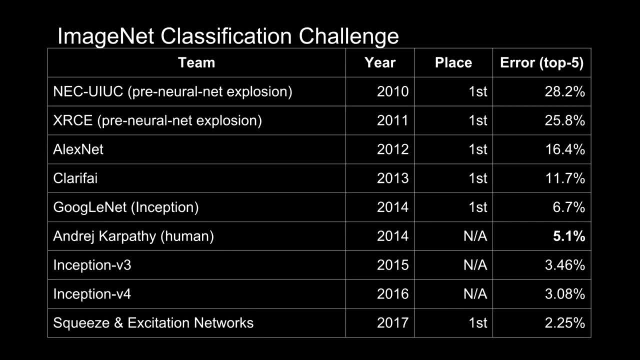 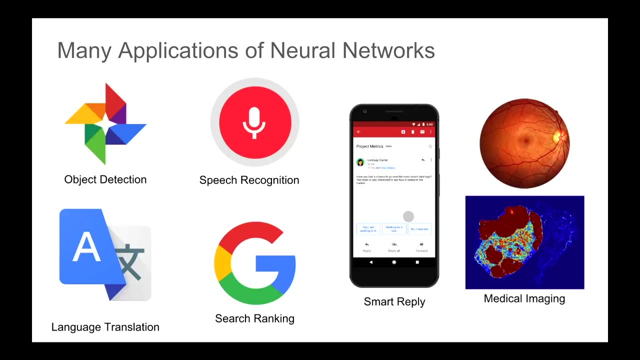 So in this time everyone has become really excited about neural networks and they've really become very mainstream. I'm not sure if you've heard of them before, but they actually power many of the technologies you would use every day. So I've got some. 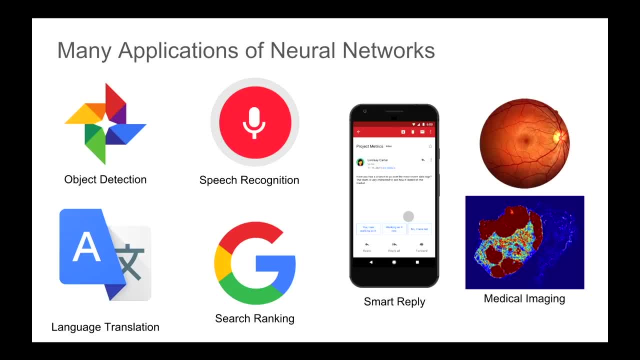 Google products there that you might be familiar with. But another area which I think is really exciting is in medical imaging. So neural networks have been shown to accurately diagnose diabetic retinopathy and also accurately detect tumors- cancerous tumors, in biopsies of the lymph nodes. 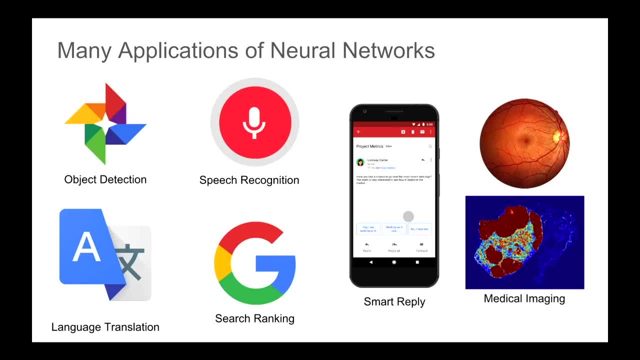 And in both cases they can do that with equal or equal or better accuracy than actually trained professionals. So this is actually really exciting. But, yeah, so because this talk is about exoplanets, you might be able to see where this is going. 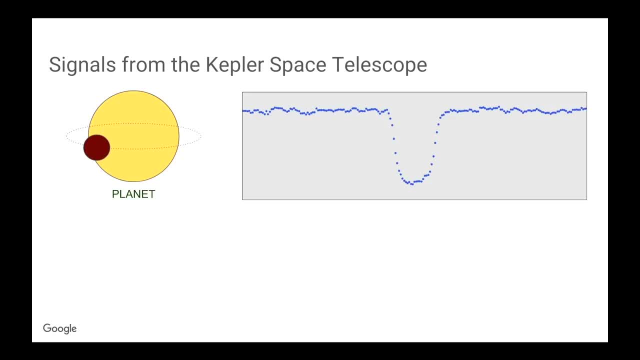 Does it work if we apply the same sort of techniques to signals from the Kepler telescope? So here is an example of a planet from the Kepler telescope. This is a nice strong detection, like Jeff was showing us before, And we've already searched. 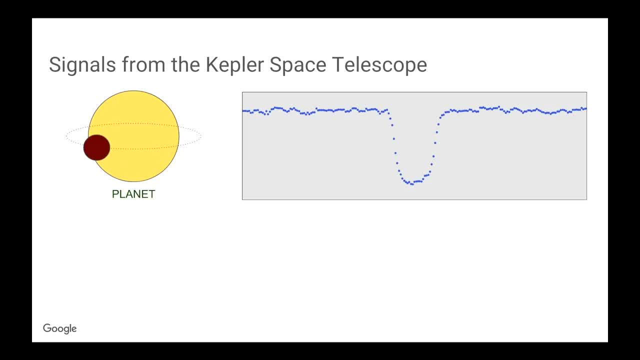 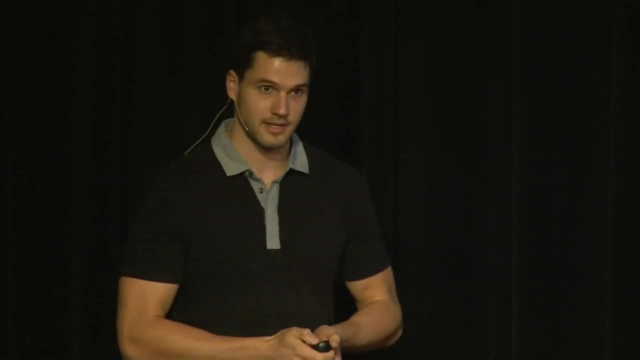 the data from the Kepler telescope right. Humans have manually vetted over 30,000 different detected signals from Kepler And we've confirmed, I think, over 2,500 planets so far, and there's 2,000 more candidates in there. 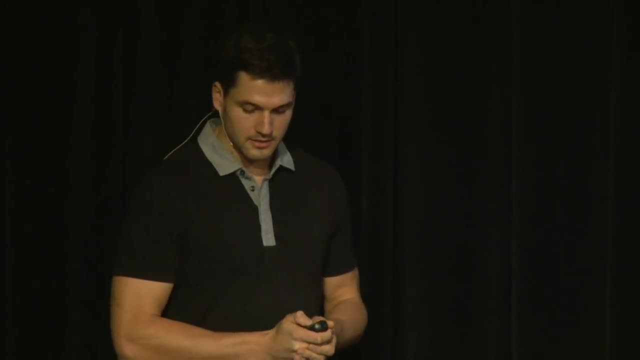 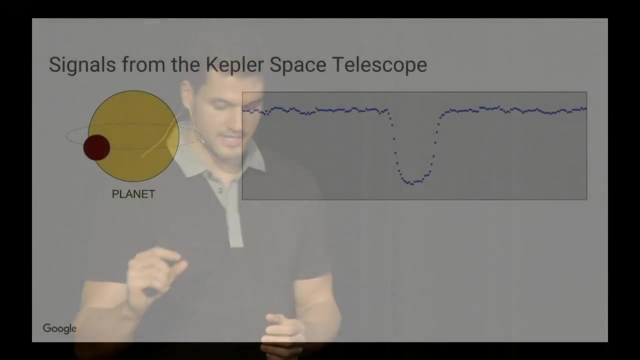 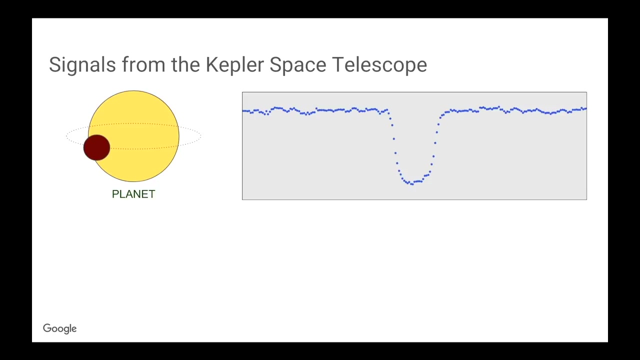 that may in fact be planets, But there are still more signals in there. potentially. There are signals like right on the edge of the detection threshold that have not been thoroughly examined by humans. So here's an example. Is this a planet or not? 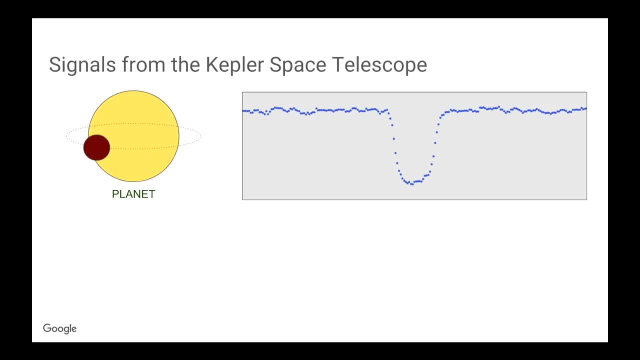 What about this? What about this? These have not been closely examined by humans yet. In fact, these last two examples are planets. They're planets that our model actually found, But I'll get to that in a couple of slides, So I won't really dwell too much. 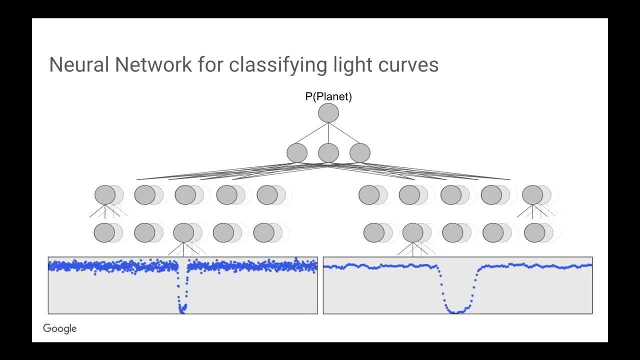 on the technical details here, but what we did was we came up with a neural network model that takes as input these light curves that have already been processed and calibrated by the Kepler pipeline that Jeff worked on. So they take a light curve and they output the probability. 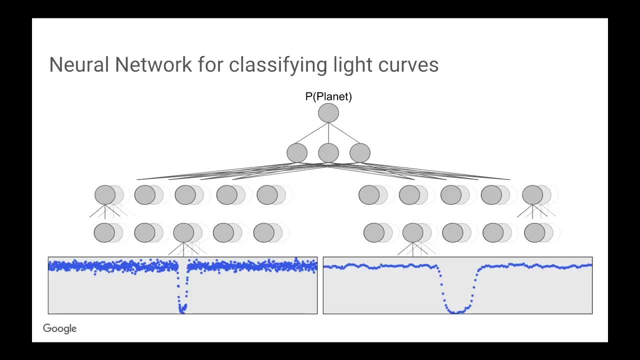 that that light curve is actually a planet, And you'll notice that it actually takes two light curves. They're actually two versions of the same light curve. We found this was one way that we could improve the accuracy of our model. We include one wide view. 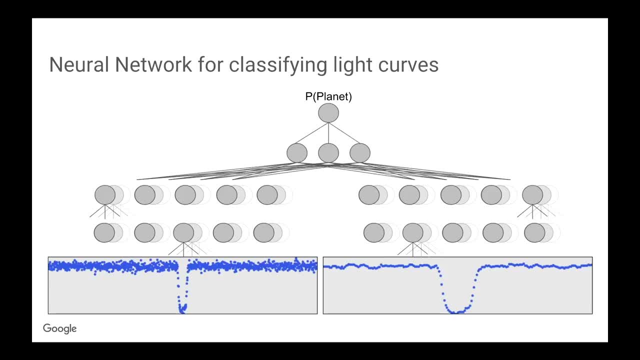 of the light curve and one zoomed-in view of the light curve, And the zoomed-in view gives our model the ability to really look at the shape of the signal, and that really gave us a boost in accuracy. The other thing that we need: 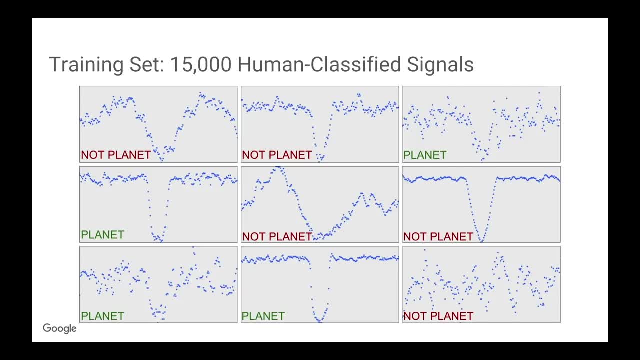 in machine learning is we need a training set of labels, of labeled data, to train our model on. And luckily humans have already gone through thousands and thousands of signals from Kepler So we were able to use these to train our model. So once our model had trained, 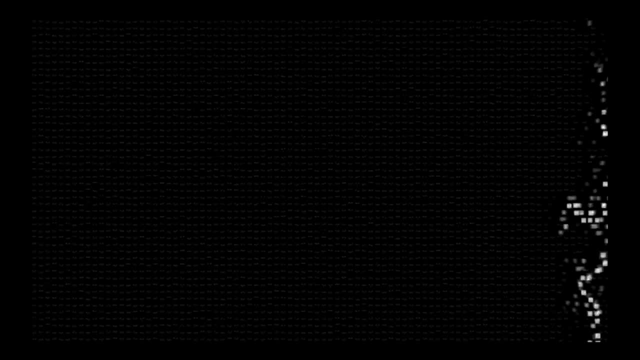 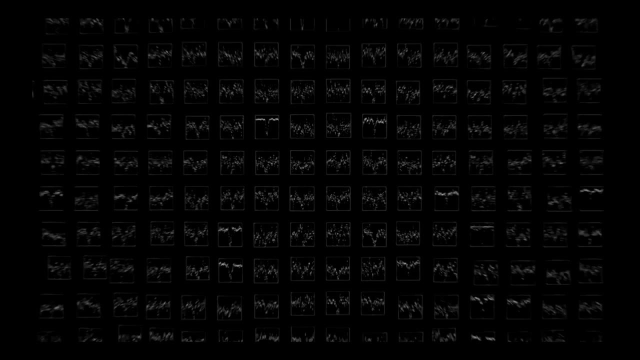 on these 15,000 signals. we then turned our model to a search of 670 stars from the Kepler. data set out of 200,000.. And we really did this just to sort of test our method and see if we could come up. 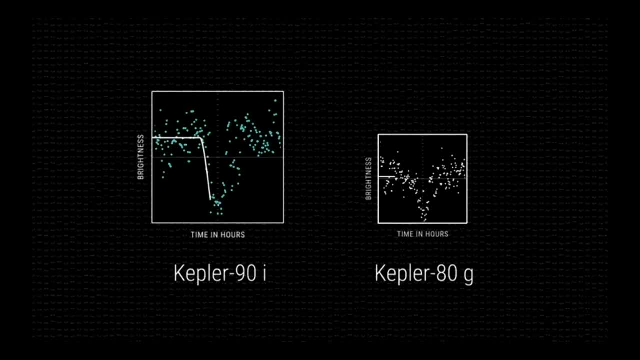 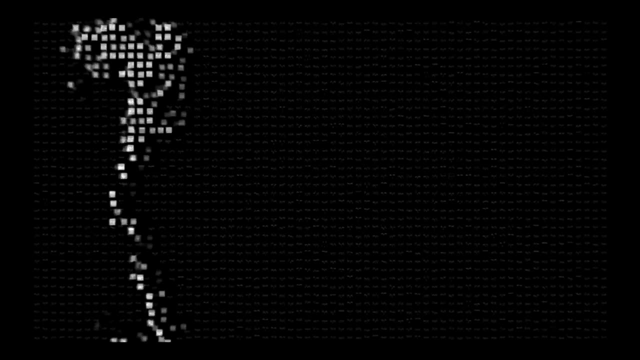 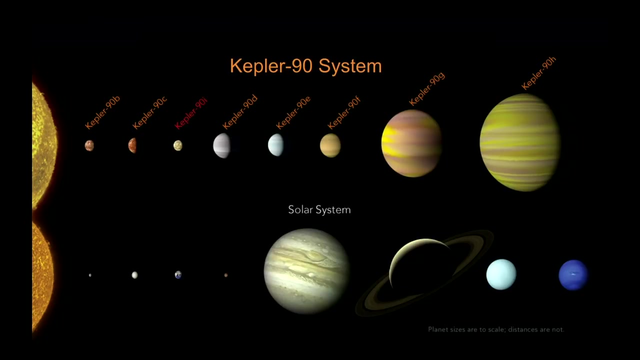 with anything interesting, And in fact we did discover two new planets, one of which was the exciting planet Kepler-90i, which just so happened to be the eighth planet that was discovered in the Kepler-90 system. So I've spoken mainly. 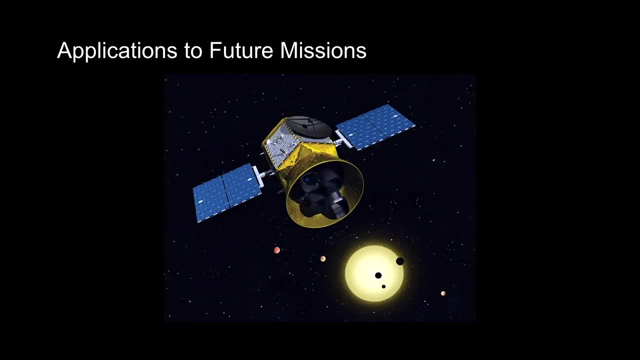 about Kepler, but what about TESS? So I very much hope that we'll be able to apply these same techniques to the TESS mission. I think one challenge that we're going to have is that because the TESS mission hasn't started yet, 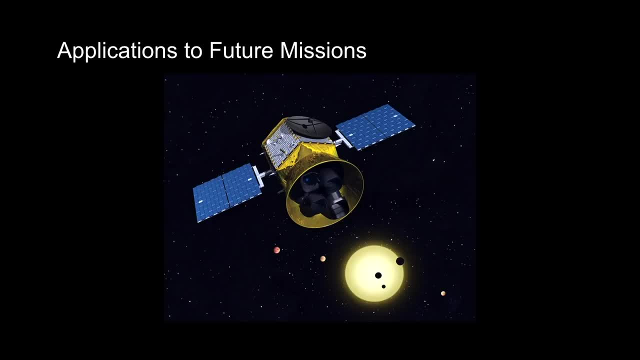 we don't have the ground truth data, We don't have these signals from the TESS mission that have been classified by humans yet. So the question is whether we'll be able to accurately simulate a training set, to feed into our model, to actually train a model. 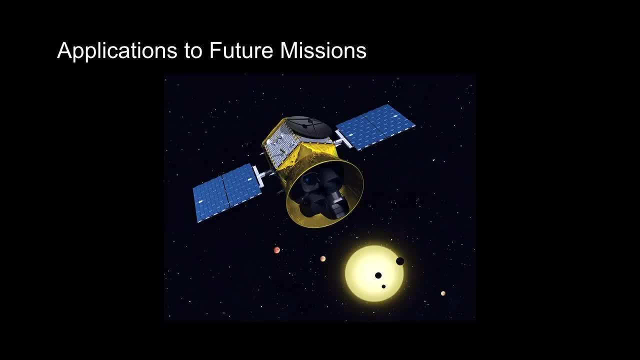 accurately enough to you know for the same technique to work in TESS data without having the big corpus of human classified data. So that's an open question and it's something we are actually talking about working on this year. Cool Thanks. 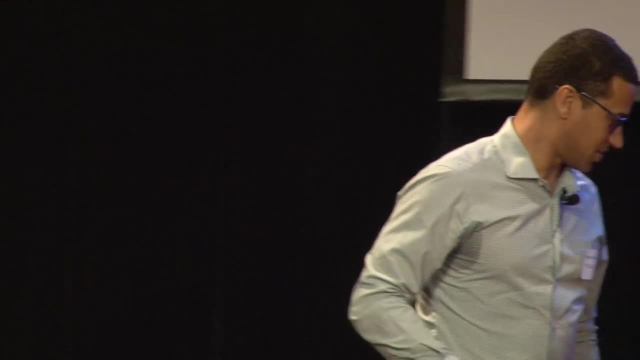 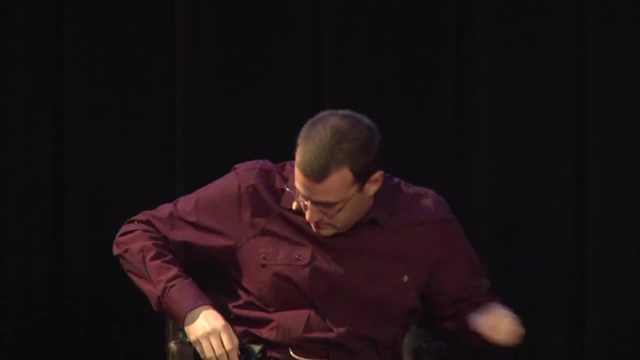 Okay, Thank you very much. So the next step here is to have a very simple a basic conversation on what you did And, in fact, before we go into the science and all the details about the algorithm, et cetera, 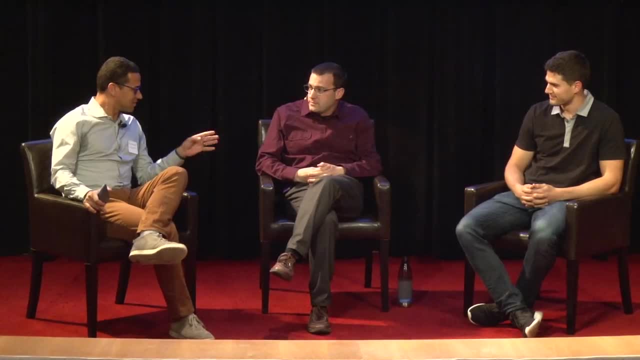 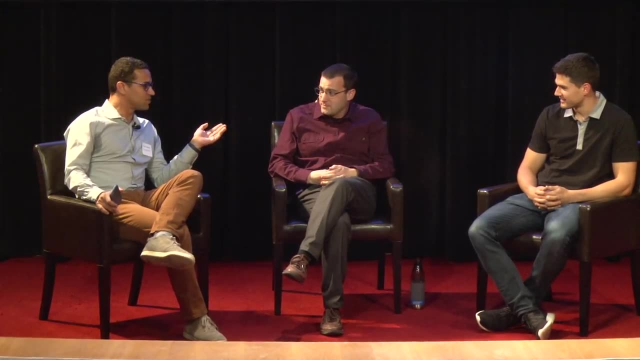 I have some kind of personal questions for you, But don't worry, not your social security number, nothing like this. Just Jeff. First of all, how did you come to work on Kepler? Why did you take this mission impossible of going through this? 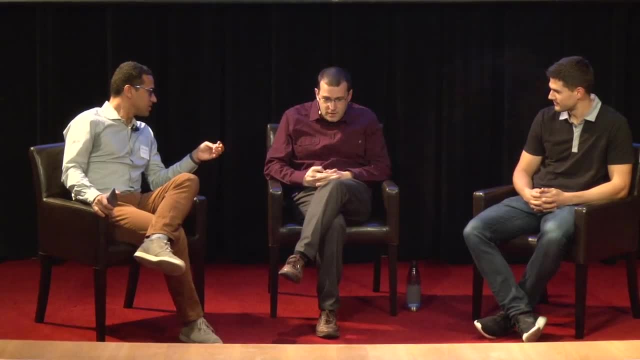 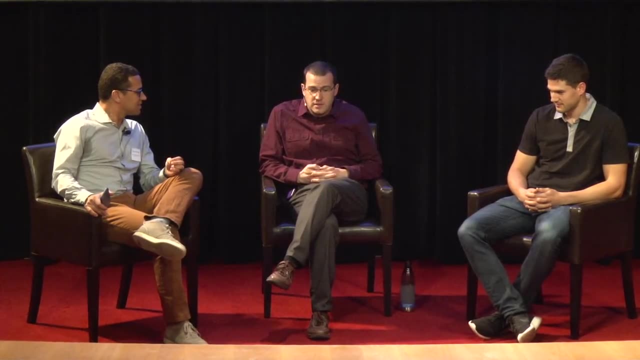 developing this pipeline. What motivated you? Well, as you mentioned before, I started in accelerator physics and I really enjoyed it, And I had always, as the way I phrase it, I was looking into the smallest of inner spaces, just looking at the tiniest. 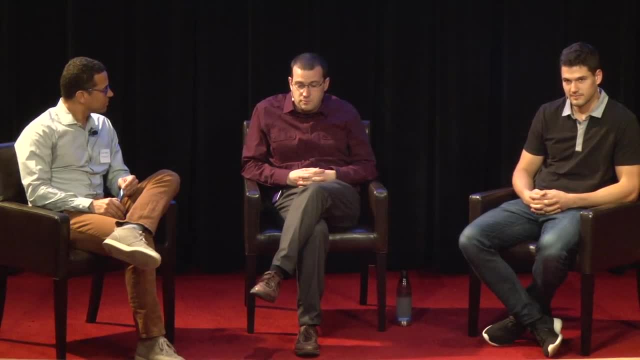 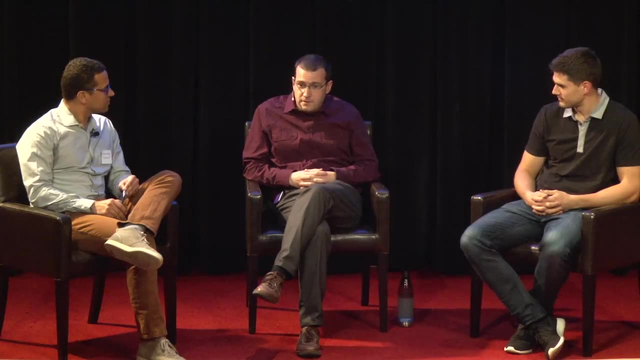 little things, developing machines that are miles long, if not 22 miles long, searching at these little tiny things And I really enjoyed it. But you know, due to funding situations, I decided to start looking for other things. It's still not certain. 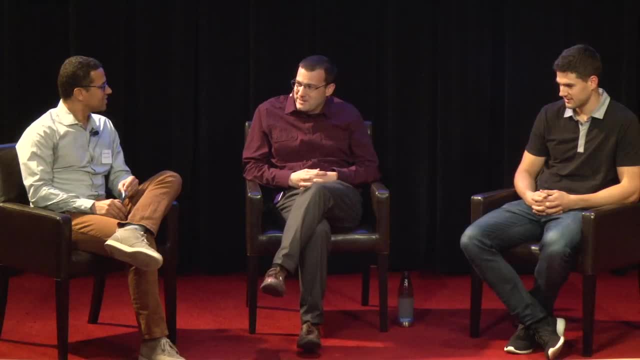 that the International Linear Collider will be built. If it is, it probably won't be in the US, And so one option would have been to stay in the field. I could have gone to Geneva, Switzerland, work in the LHC. 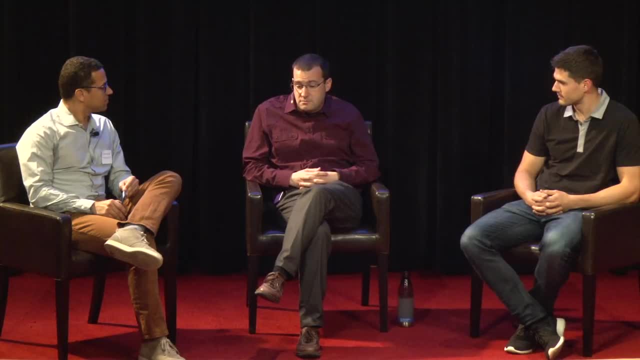 I was already working on the LHC, But I like California. There's one reason And I knew somebody that worked on the Kepler mission and I asked him: you know, do you have anything interesting going on? And after speaking to him, 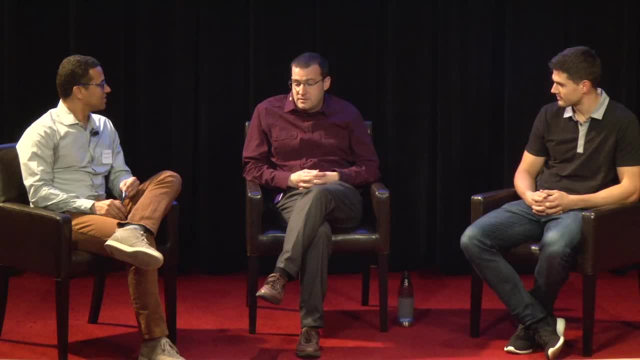 and other people. I found out that even though the application is completely different, the techniques in many ways are quite similar And the ways that we model the data and simulate the data and fit the data is quite similar. So I realized that my skills 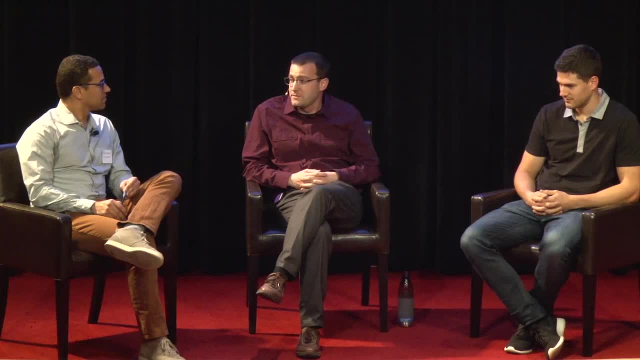 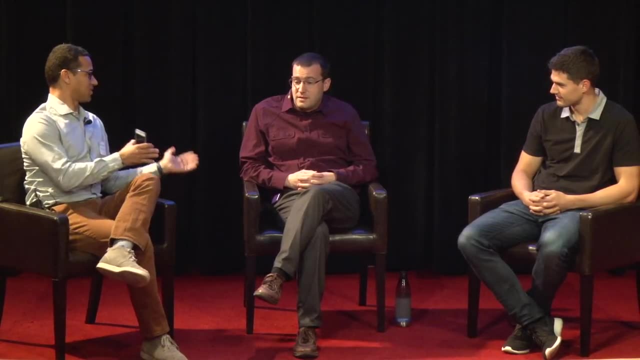 kind of carried over and I've been here ever since And it's been fun. So I started in 2010 on Kepler. So basically, data is data, data in physics And if you can translate it quickly from looking at the tiny things, 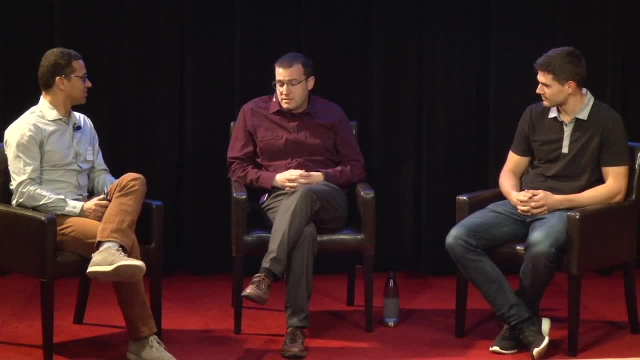 to looking at stars Right. Well, once it's ones and zeros, you know. anyways, it's quite similar And it's also for me personally finding I have to find good, strong meaning in whatever I'm working on. 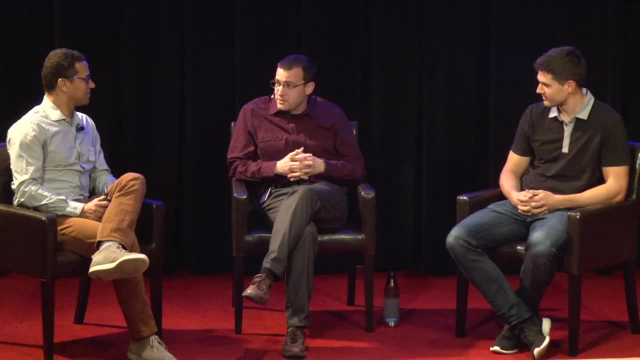 And searching for some type of discovery is important, And I find searching for extrasolar planets just as significant as searching for, you know, Higgs, boson and whatnot. So I have the same question for you, Chris. I have a question. 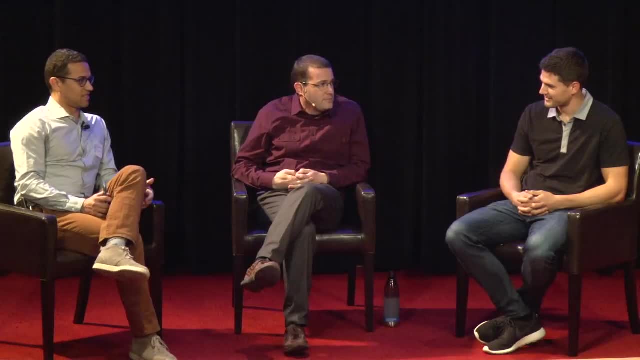 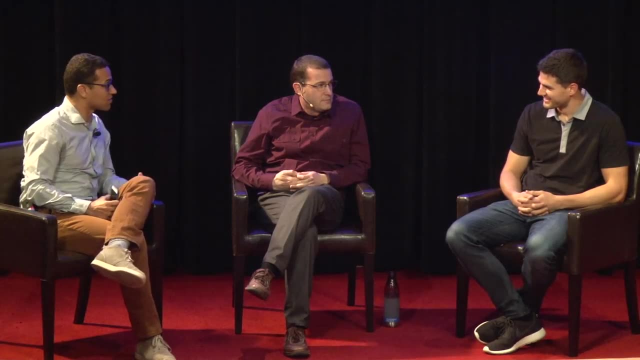 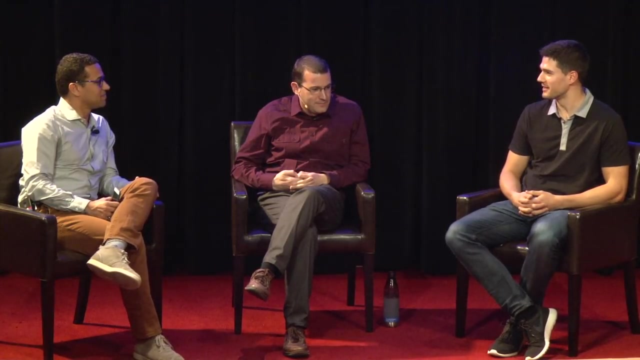 for Google, How this idea of using this new technology came out for searching exoplanets, Why you could have done plenty of other things like characterize dogs, races and why why exoplanets? So I was actually just reading a book. 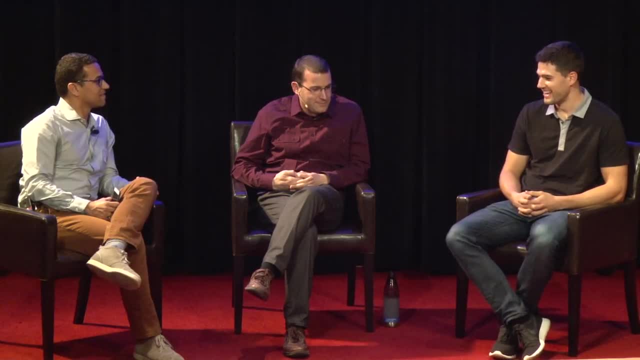 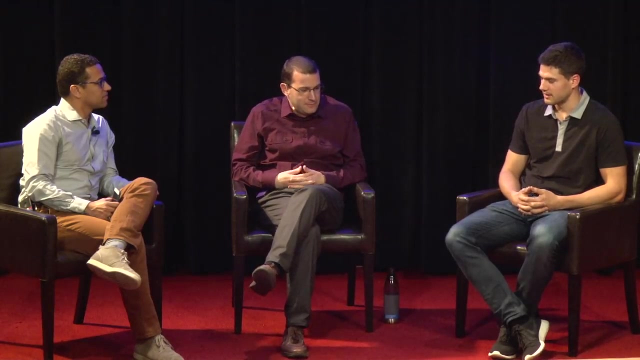 in my spare time. It was Human Universe by Brian Cox And he was talking about the Kepler mission and how many planets had been discovered, But I definitely don't know. what he said was that in astronomy, like other fields of science, we're now getting 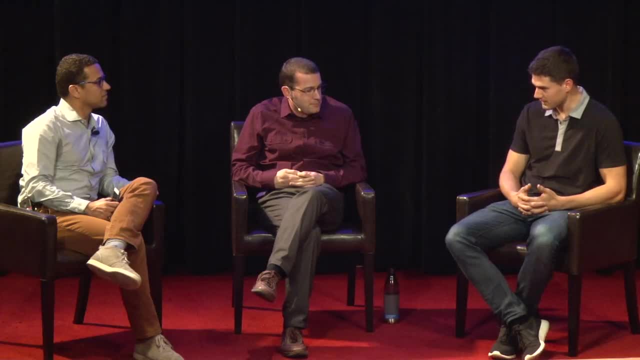 to the point where we're collecting more data than humans can analyze manually. I guess the traditional way that science was done was that astronomers would gather data and then they would examine it themselves. But we're getting to the point now where our technology has sort of 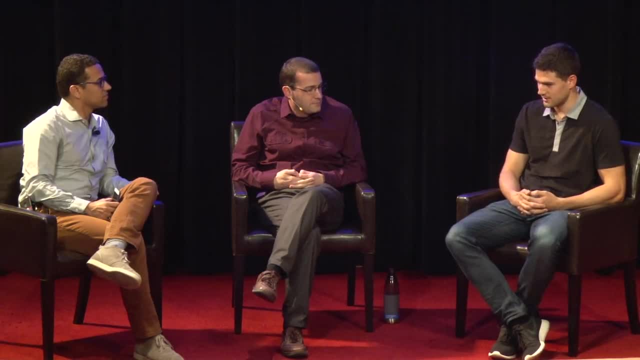 outpaced how quickly humans can discover planets, So I just wondered whether anyone has ever tried to apply machine learning to the Kepler data set. And so I did a little bit of research online, and I found an astronomer: Andrew Vanderberg. 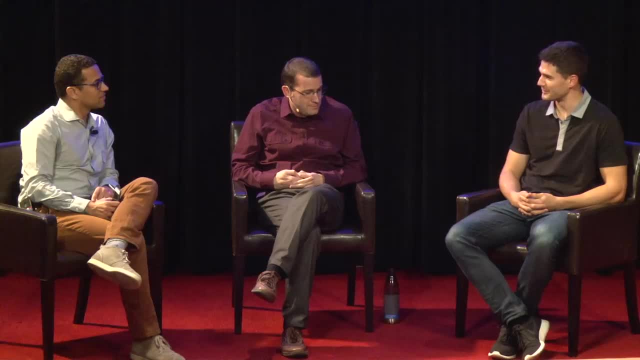 who was at Harvard at the time And I just sent him an email and said: hey, I work at Google, I work in machine learning. Would you be interested in applying machine learning to the Kepler data set? So I was able to. 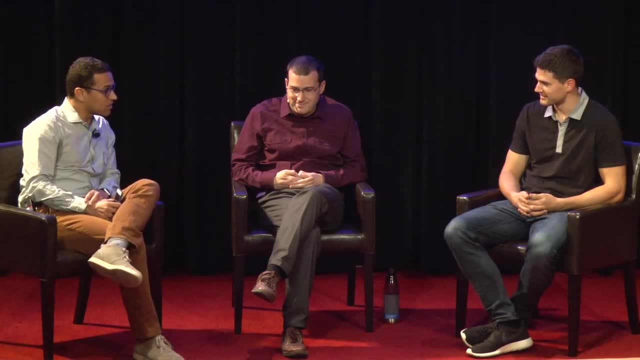 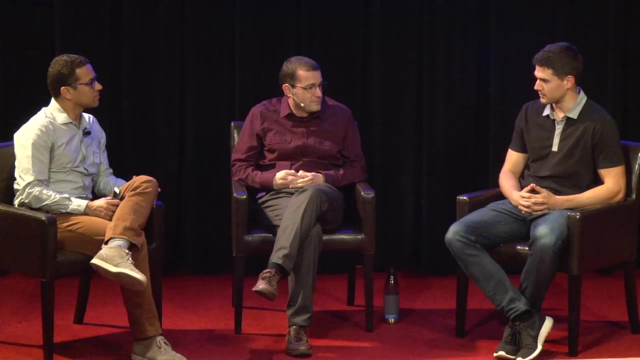 do a little bit of research in the past with a couple of other researchers in the University of Pennsylvania, And I actually found a couple of people that had fraction of the Kepler data to see if we found anything interesting, and so we started with 670 stars, because these are the stars that already had multiple 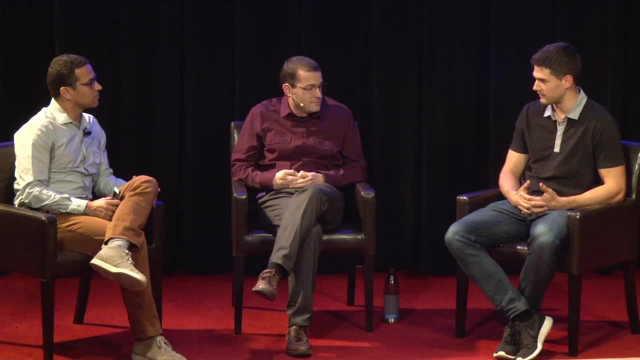 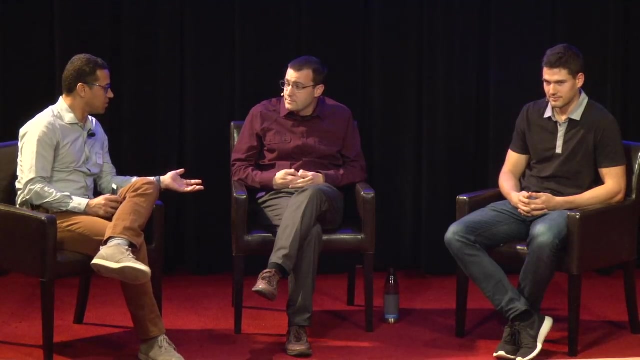 planets discovered around them, and so we figured it was more likely to find additional stars around those planets than if we just searched around other stars. but that's that's certainly something that we're working on right now- is to apply the same technique to all 200,000 stars. so, Jeff, you, you. 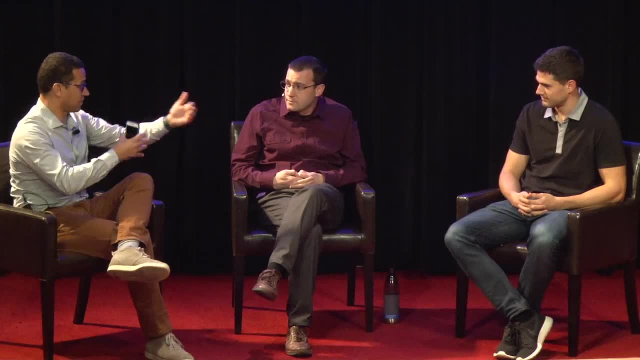 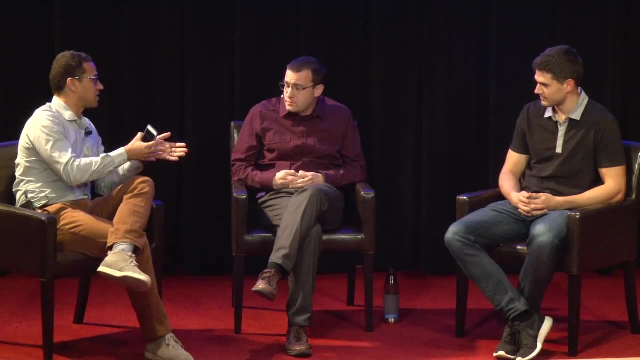 basically feed with this pipeline, you basically feed the machine learning you, you give them some transit which has been already validated as planets or some artifacts. so it means that you're still working on the Kepler data, we're still processing those data. so there is some new discovery that we come from you. 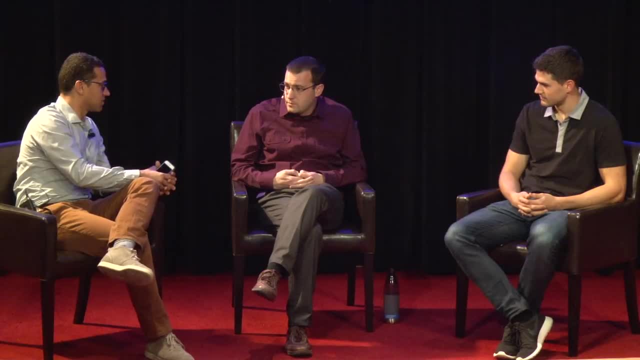 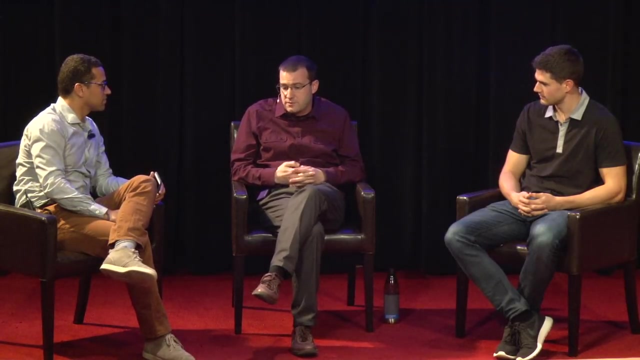 and combining those two. those two works right, definitely. yeah. I mean, the pipeline work for for Kepler is basically over, but we we have this huge data set and, as Chris mentioned, there's a lot of vetted data already where it's already been confirmed if it's a planet, and we've 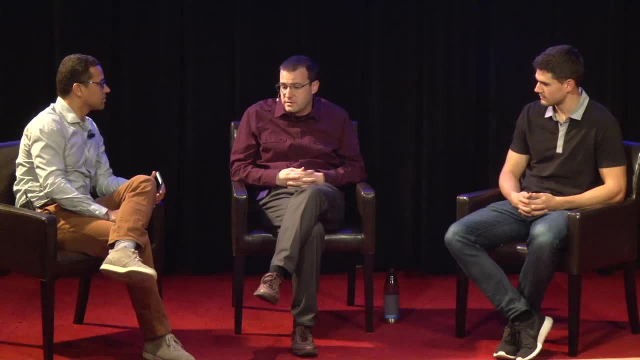 already classified things, that there's this huge training set and Kepler and it's and a lot more can be done in training a machine learning algorithm to detect even more and and really it's like the examples I showed: once you get near that noise threshold it's hard to tell and whatever you can do to help. 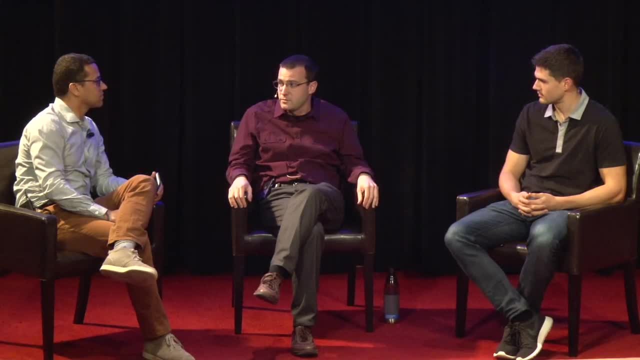 figure out. is this real or is this just some artifact to be very useful and and lots of times it's just humans looking at it with their eyeballs, and that only goes so far and and, as people can appreciate, if you're staring at the moon and see a face and I, we see things that aren't really. 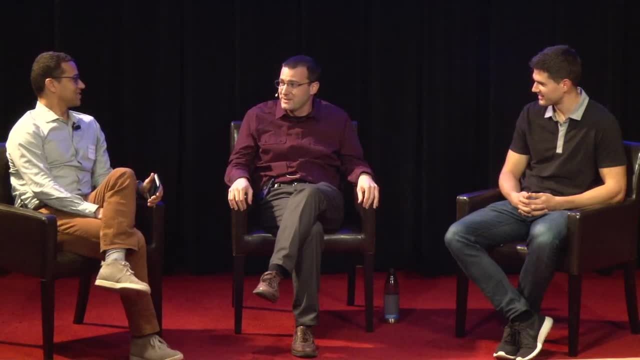 there, so machines are sometimes better than us in that case. so we mentioned to Chris like a year ago we had a meeting where we talked about using machine learning to dig into the Kepler data. that was a year ago and you remember this discussion we had together, so you were ahead of us. 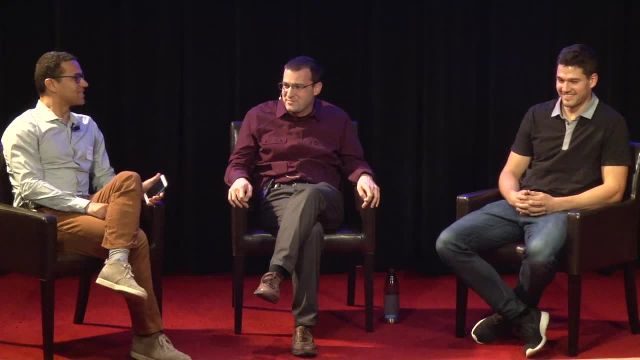 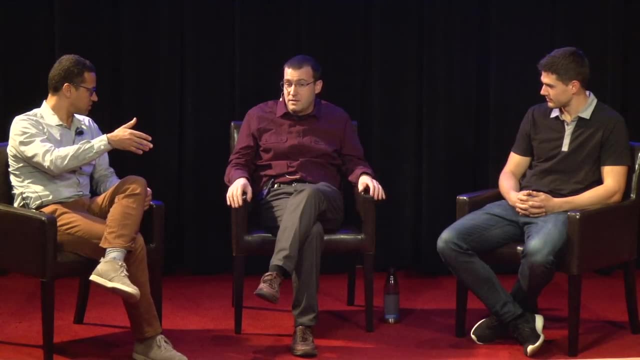 So for the test data. so this mission is not launched yet. It's going to be launched at the end of this year, April. April of this year is the current plan. One of the problems with machine learning is that you need to train this algorithm. 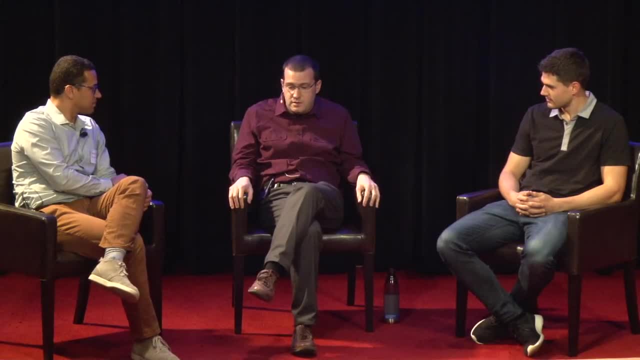 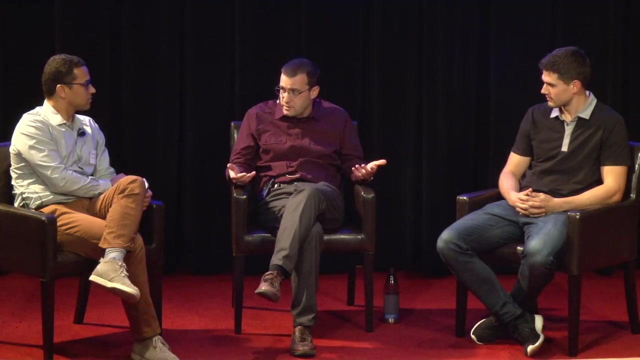 So what solution do we have? Well, we would love to use a machine learning algorithm in order to classify the transits we detect, And right now we have a very sophisticated simulator that simulates the night sky and also simulates the instrument and puts in all the instrumental artifacts and everything. 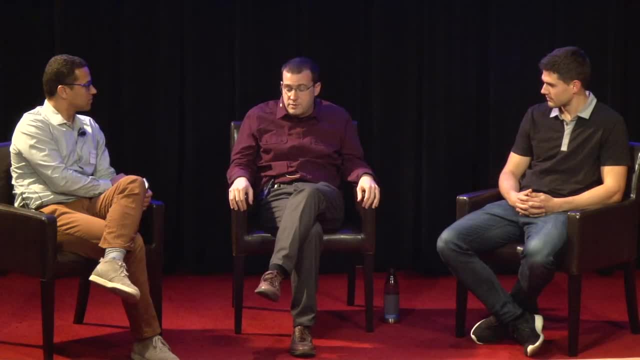 It puts in clips and binaries and all the other stuff, And we've been using the simulator to tune our algorithms for well over a year now, And so we do have a mechanism to generate a large amount of data, A large amount of simulated data with absolute ground truth. 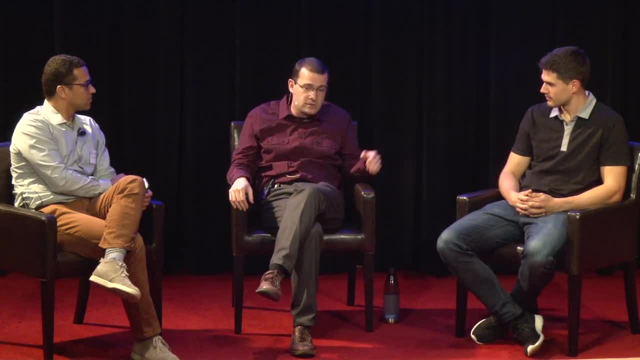 And we know what the answer is because we put it in there And so, like Chris was alluding, this could potentially be very useful. but you've got to be careful, because simulated data never really looks like real data, But if it's close enough and if we think we can rely on it, 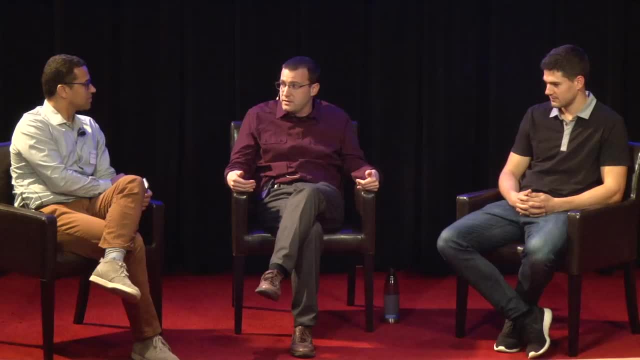 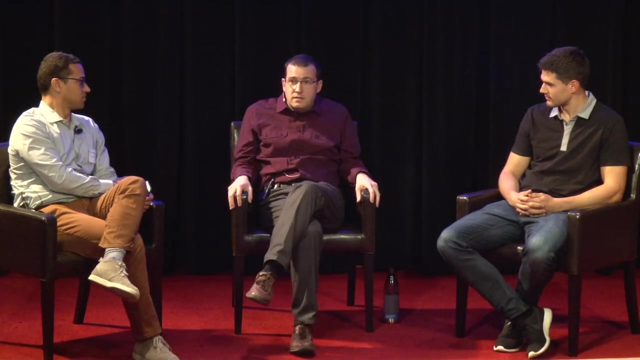 then, before we actually get real flight data down, we might have a trained algorithm ready to start classifying it. So the goal will be to have, like in every three months, a catalog generated automatically by a machine learning algorithm. That will be the best for you. Yeah, well, every month, because it's every 27 days for tests. That would be ideal, I mean. one problem is that we need to do ground-based follow-up measurements in order to figure out if these are really planets or not, And it will set in the sky very early on after tests detect them. And we'll only have a couple of months to do the ground-based follow-up measurements. And we'll only have a couple of months to do the ground-based follow-up measurements. And we'll only have a couple of months to do the ground-based follow-up measurements. 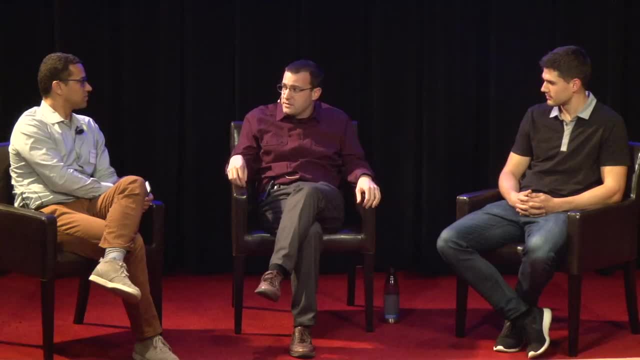 before they're obscured by the sun. So whatever we can do to speed this up, to eliminate all the chaff and figure out what is really interesting that we want to look at, the faster we can do that, the better. So are you going to work together on this, or what's the? 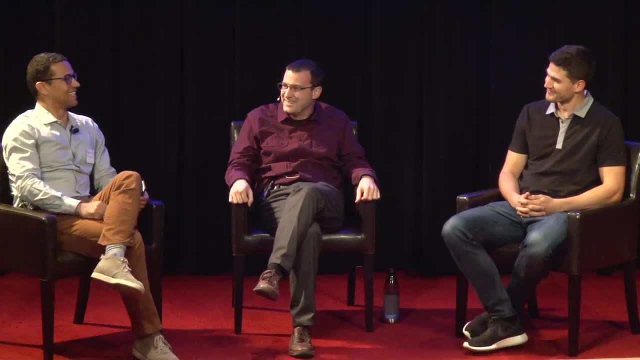 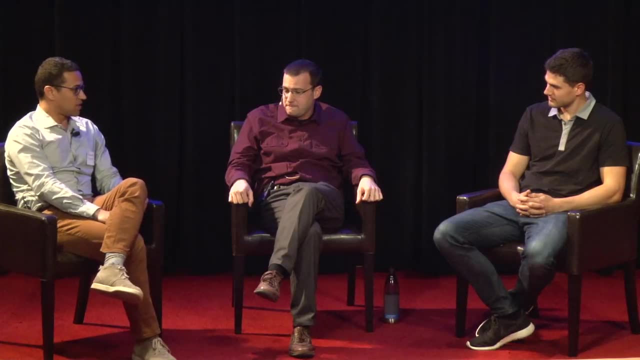 Well, I hope so. We've been talking All right. So you? so? these are detection by transit, but you may know that astronomers are now trying new techniques to look for exoplanets. We try to image them directly, for instance. 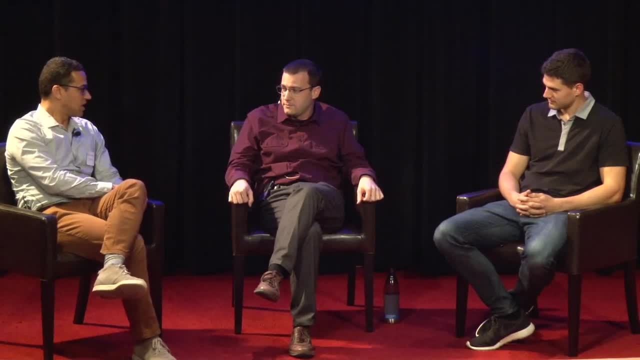 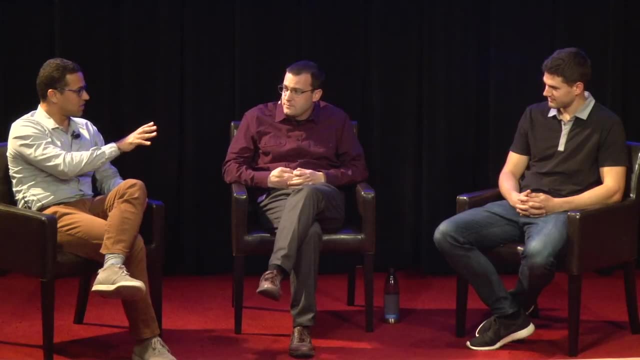 One of the projects is a project, GPI, that I work on And we have a ton of data and we have the same problem than you. I mean, we use very complex algorithm to clear the data, et cetera, But then at the end it's a human being, generally a student or postdoc. 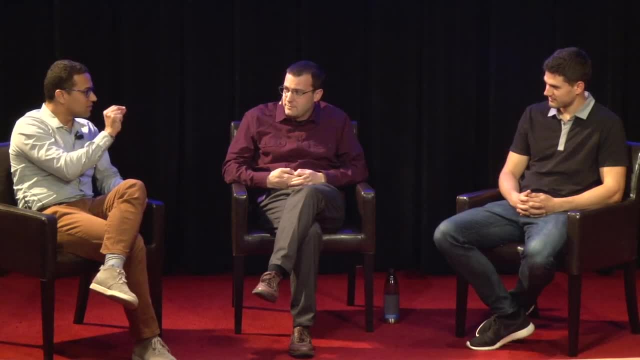 who is patient enough to look at each of the, each frames, that will identify this tiny dot. that could be a planet. So maybe there is a new job for you. Maybe you should start thinking about using this same kind of algorithm, but for coronagraphic observation of. 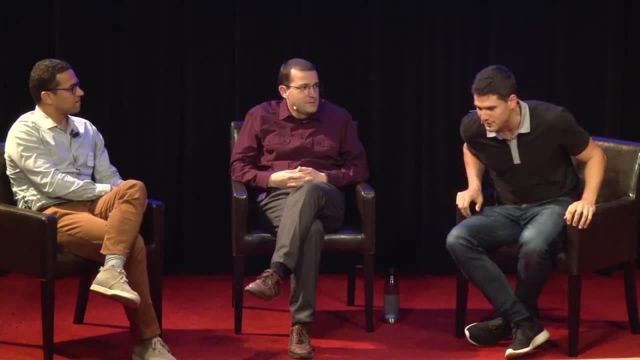 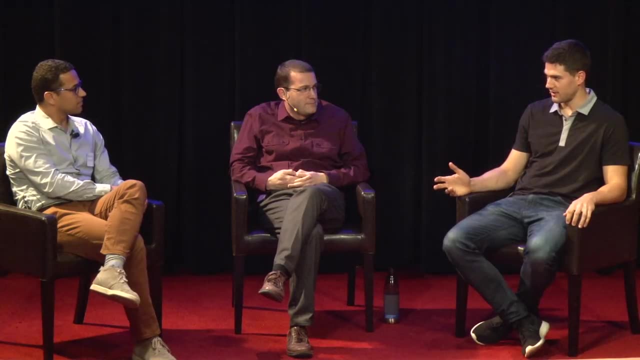 of exoplanets? Yeah, definitely. I think my first question to you would be: how many labels do we have? Because that's, I think, that's that's the big issue. I think in astronomy and many areas of science, we certainly have the data. 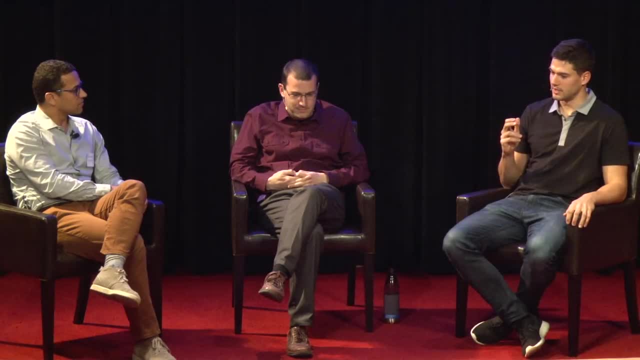 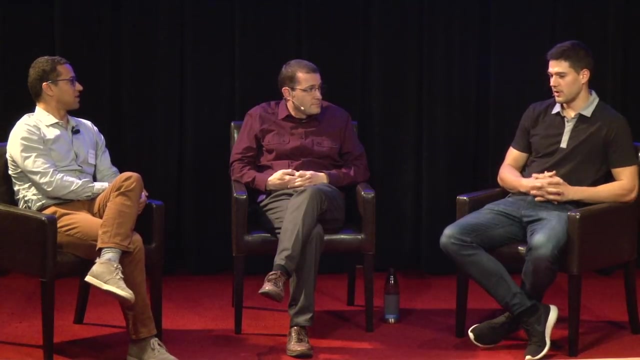 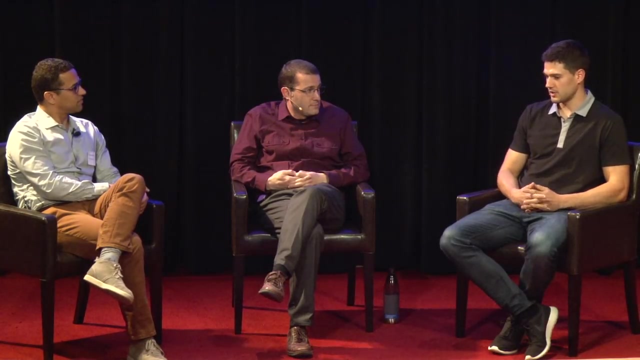 We have the machine learning techniques and we have the computational power, But our best machine learning techniques require labels, And so labels usually require humans to look at the data first. So what do you mean by labels? Right? so in in the case of of Kepler, the labels. by the labels I mean a collection. 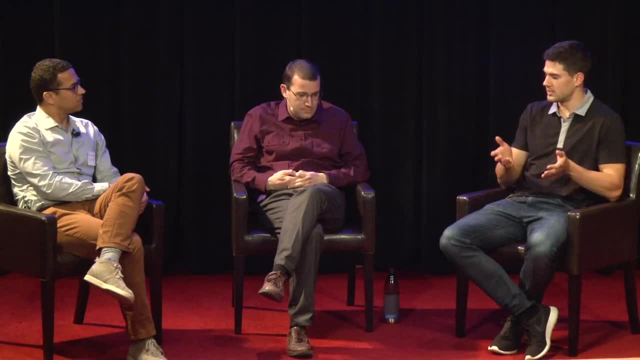 of signals, and the label for each signal is: yes, this is a planet, or no, this is not a planet, And so we need the labels to guide the machine learning algorithm during its its training phase. You know what? what? what is it that we're looking for? 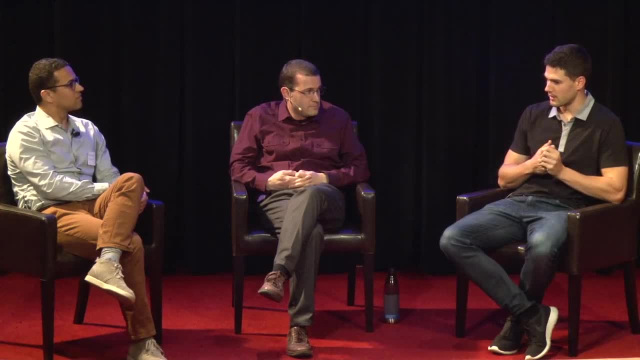 What is it that we're looking for? What is it actually trying to predict, you know? So in in this case, we were trying to predict whether it was a planet or not, So we needed a large set of labeled signals that were were labeled with: yes, this is a planet. 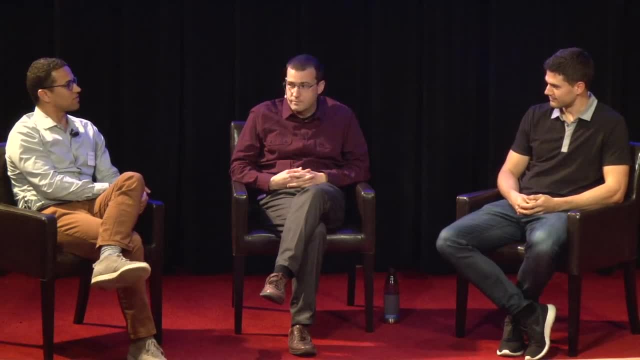 or no, this is not a planet. Okay, So we do have labels, I think. So maybe we should talk about that. We should talk about it, All right, So I have a questions which kind of keep me awake, for about machine learning, 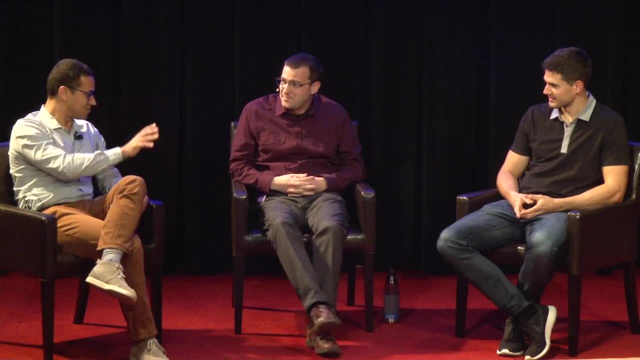 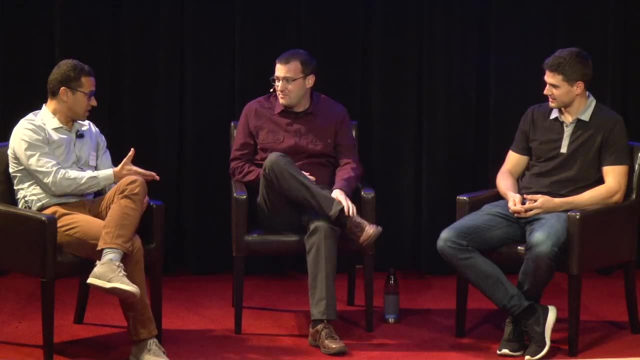 and artificial intelligence in general. So I'm going to ask you this- and please feel free to tell me if it's a very stupid question. We we have a program at at CETI called the FDL that we started three years ago- almost now. 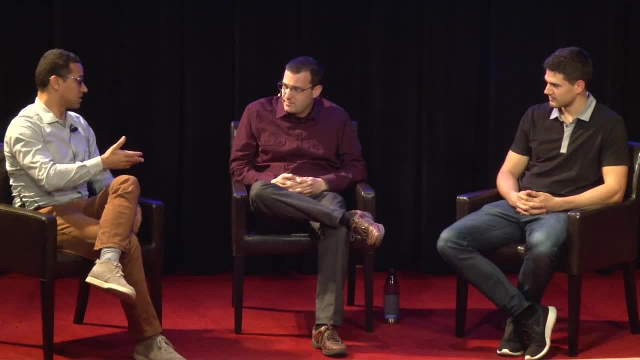 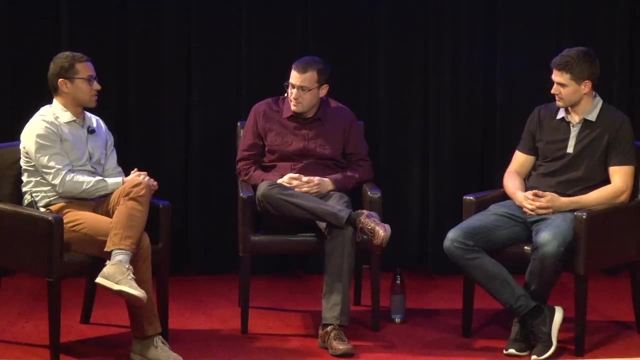 We start, the goal of the program was to basically introduce artificial intelligence to planetary astronomy, to, to, to solve different problem in astronomy. So when we started this program, I do remember my colleagues were kind of skeptical about it. Say huh AI. 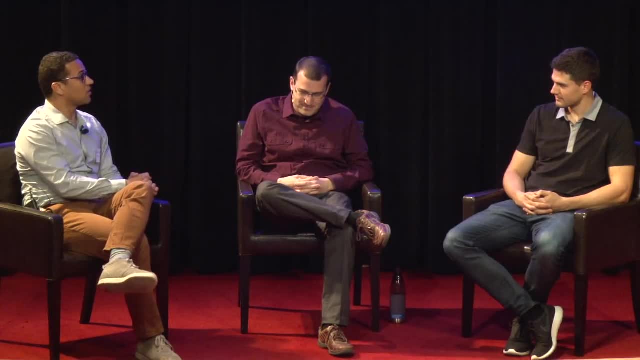 We heard about it, We heard about this And then after the first year people get: oh, that's very interesting. We get some interesting results here because we did have, we did manage to solve some of the problem that we had in astronomy. 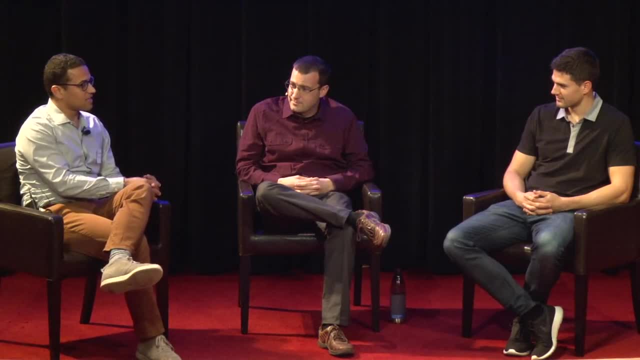 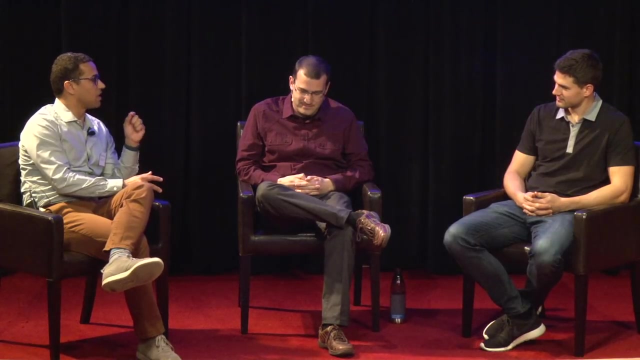 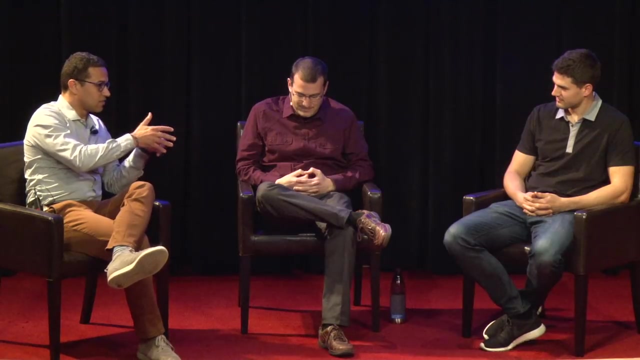 And now we're entering in the third phase, where scientists are getting a bit afraid of it. And they're afraid of it because they say that we are, with machine learning algorithm, we are breaking the scientific method. You do remember, the scientific method is all about solving the problem and by collecting data, 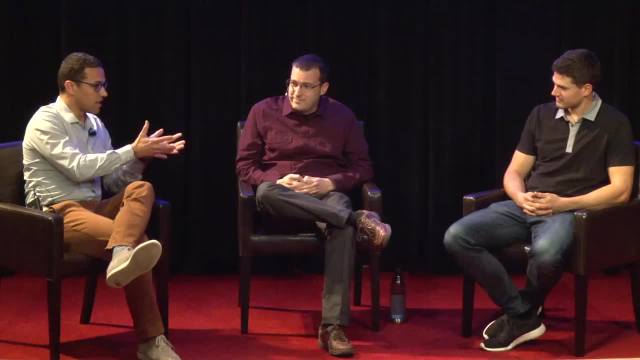 and from this data we are building a theory, and theory based on physical laws and physical processes and making predictions right. People who use machine learning: they have a lot of data, They feed the computer with it and that's the way scientists see it. 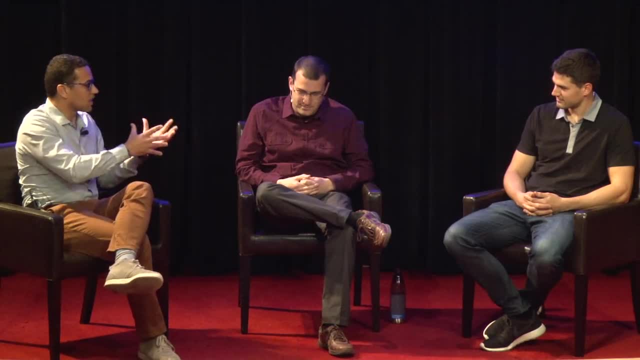 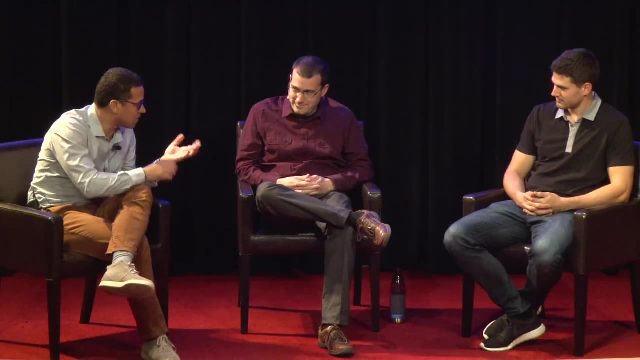 And then some kind of low, some kind of I'll go with, From this algorithm. they can predict, but they don't know why. We don't know why this prediction works. We don't understand the underlying physical processes. Some scientists will say that's because we're ignorant. 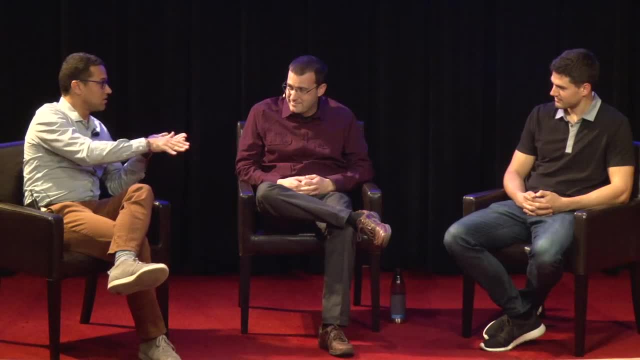 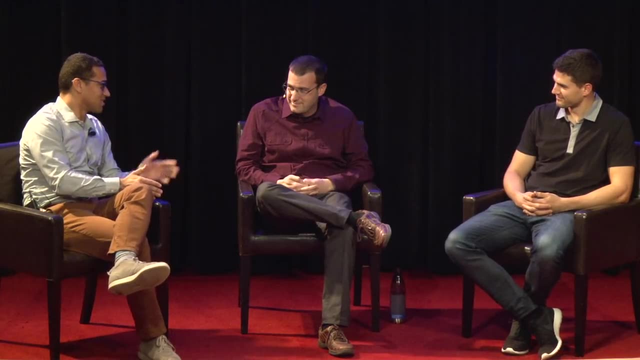 and probably there is physical processes that are hidden and we don't see them and we don't understand them, And some other scientists will tell you: well, this is not science. So what do you think of that? Well, that's a wonderful question. 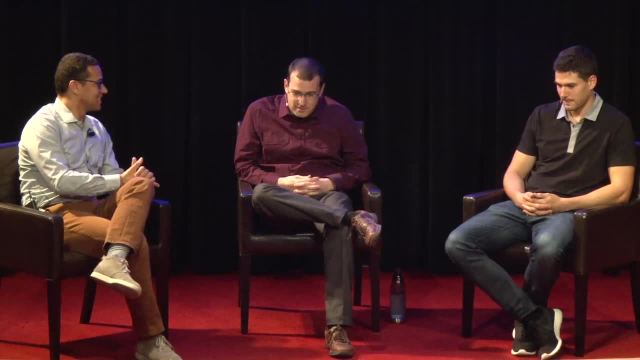 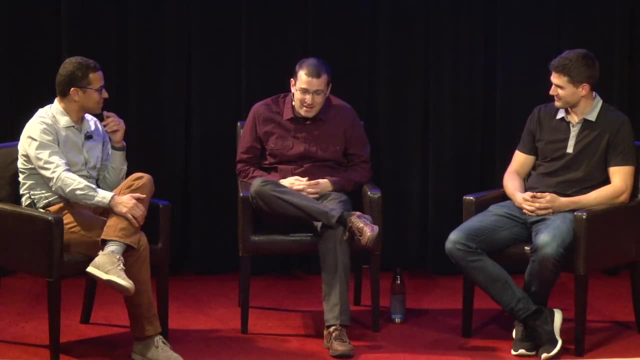 I've thought about this a lot myself. I think people give- maybe people won't like me saying this, but I think people give- humans too much credit in some ways When we- it is true a lot of people- don't trust machine learning and the artificial intelligence. 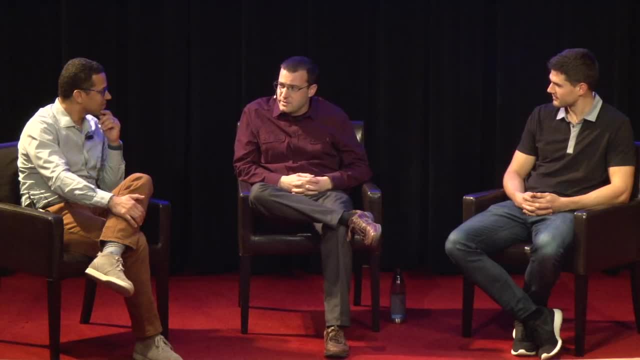 and they think it's thinking machines and they're doing something that we should be doing and maybe replacing humans. Well, first of all, people don't trust it because they think it's a machine. They think that they can't read the mind of the machine. 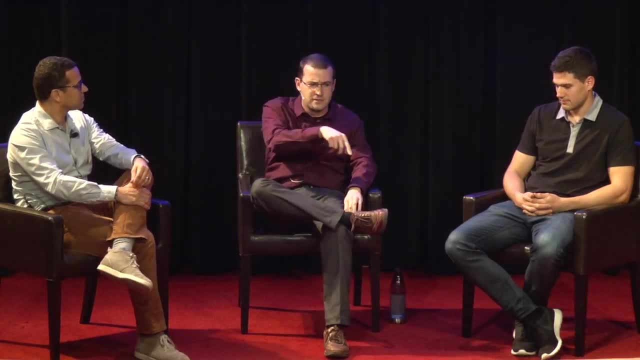 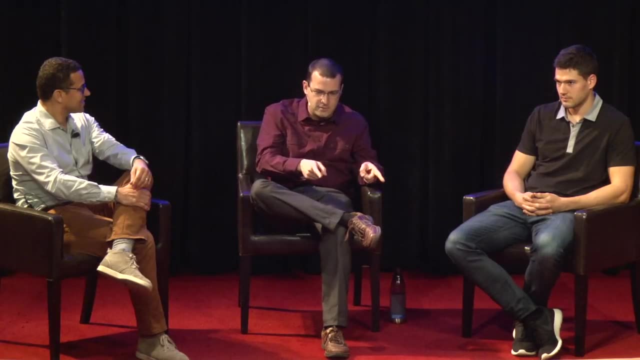 You know, I know what I'm doing, I can figure out: oh, I logically, rationally, did this, this and this and I came to this conclusion. And do you really know that you rationally made all your decisions before you got to your conclusion? 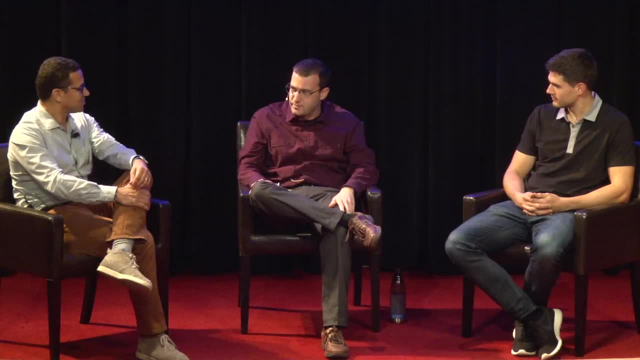 I mean, do you actually know all the synapses and everything that happened in your brain to get there? You know, the human mind is so complex and we do these convoluted routes to come to some conclusion. that is a machine doing some complex neural network. 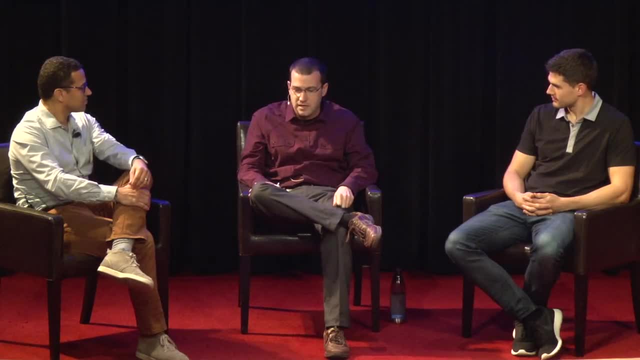 in order to come to some conclusion really different than a human using their neural network to come to some conclusion about some problem. And just because a human decided it, does that necessarily mean it's more rational than a machine, And so I don't have this fear of artificial intelligence. 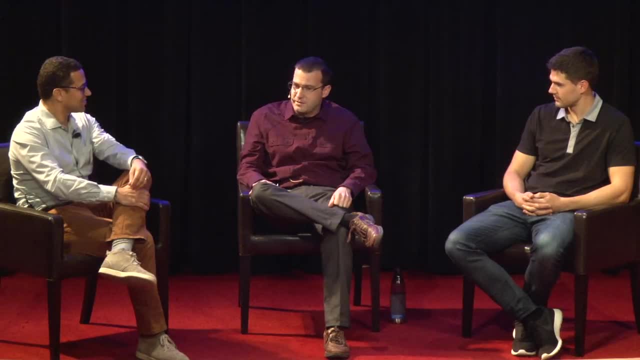 Some people do. I view it as just another tool we use, and not necessarily replacing a human or doing better than a human. It's just a tool we use and it's just another tool we use to come to a conclusion. What about you, Chris? 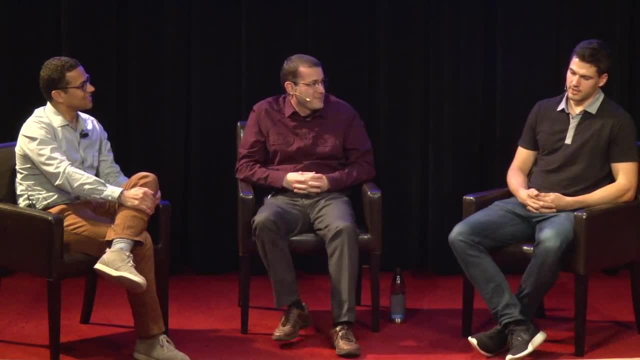 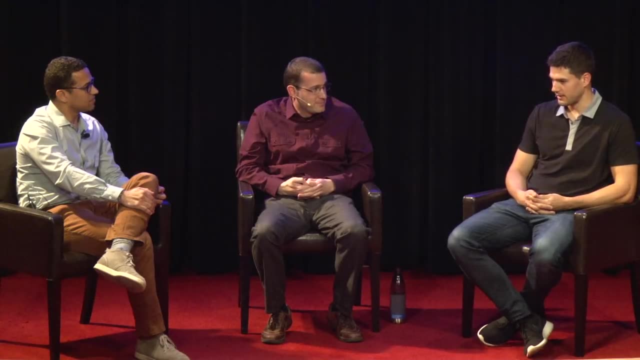 Yeah, I think that's a great point. So I think we're certainly at a stage now, in astronomy say, where, you know, perhaps it would be great to have a million grad students searching the Kepler data, looking for planets, but we don't have a million grad students. 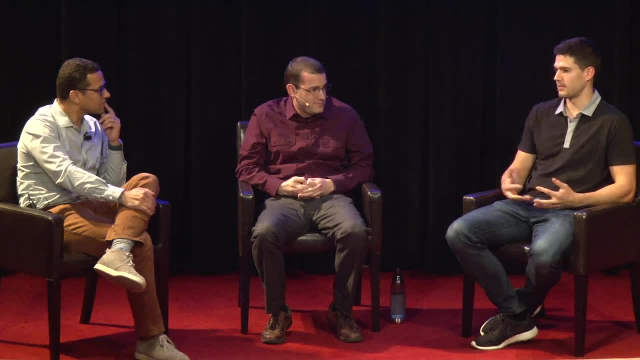 Um, So we need some sort of automated approach And, as our current state-of-the-art approach for any automated system that is going to look for certain patterns, You know, here I'm even talking about identifying images of dogs, different breeds of dogs in photos. 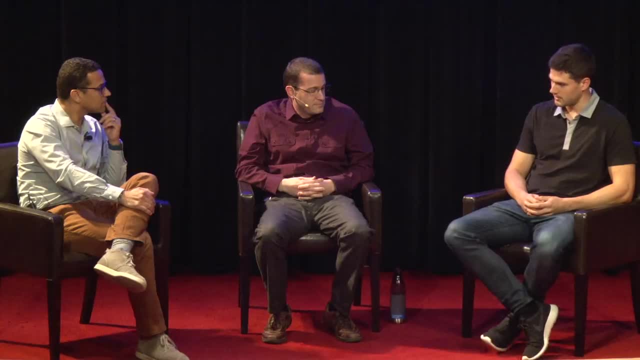 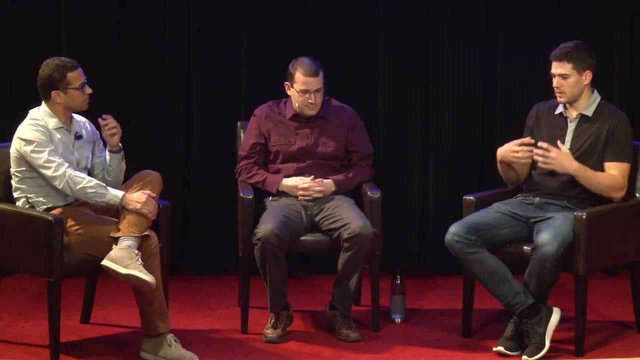 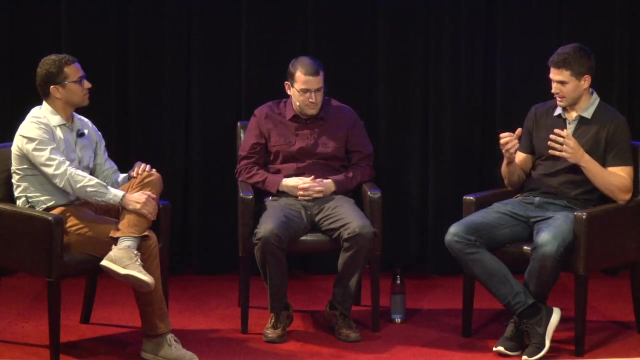 The best technique we know of at the moment is machine learning, And that's because you know, as humans, we know what dogs look like, right, But can we program that into a computer? If you think about it, it's actually really hard to do. 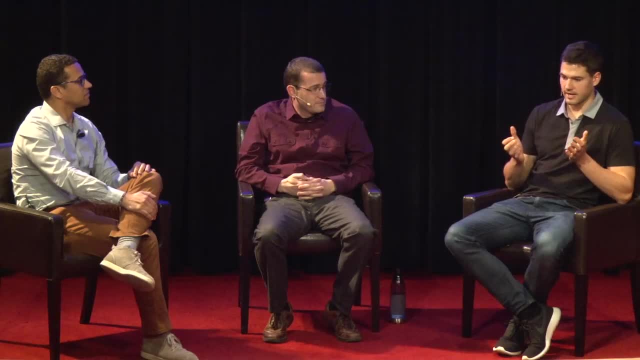 because you might try and say: OK, well, a dog is something that has four legs and a tail, and you know pointy ears, And then you would sit down and you would try and write some rules as to you know. 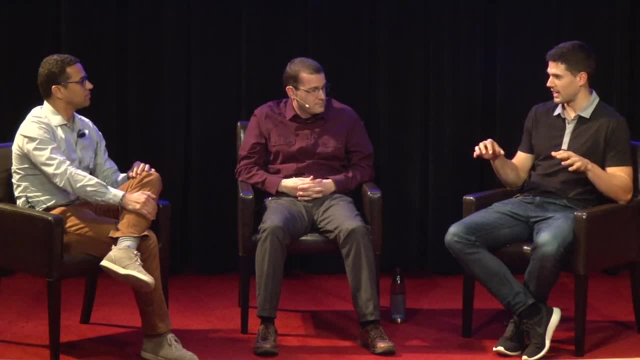 well, what do legs look like in photographs? And OK, is it still a dog if one of the legs is sort of hidden behind the other legs And it turns out to be really, really difficult to sit down and write a computer program? 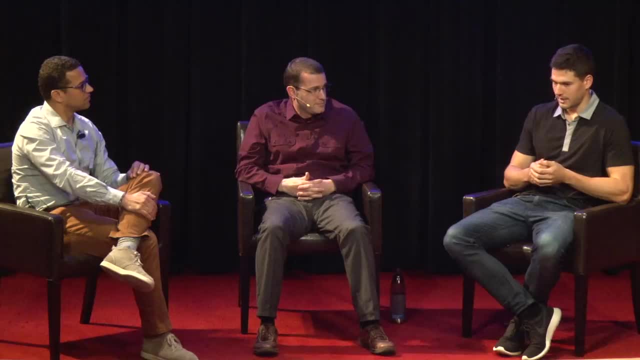 to actually match those patterns. Um And so, yeah, the best techniques that we have at the moment are machine learning approaches where we say, OK, we are going to show this system just thousands and thousands of examples of the patterns that we want it to detect. 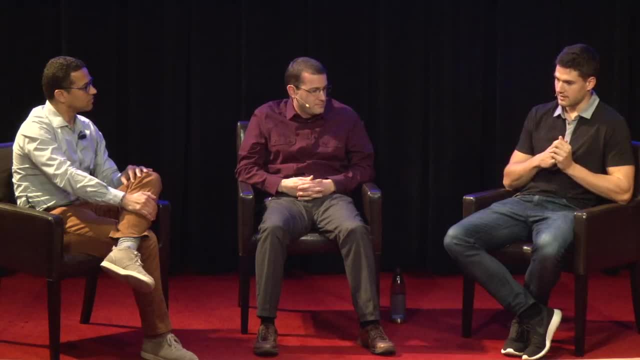 And then in the end we're going to have a system that does not have rules that we can go and read and understand and check, but it is actually going to be very, very precise at looking for those patterns that we wanted, And so I think 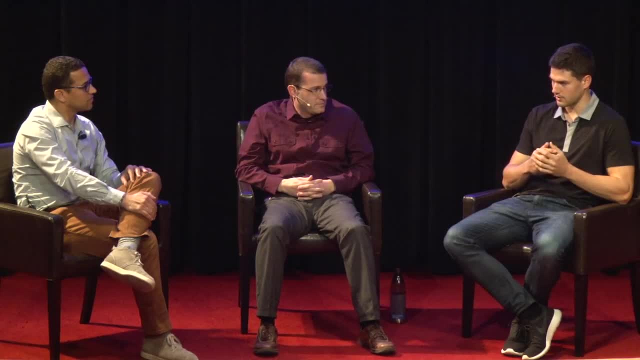 I think like that's why machine learning is, you know, going to become, I think, very important, And there's going to be discoveries that we perhaps won't be able to make without machine learning, And I think it would certainly be a shame. 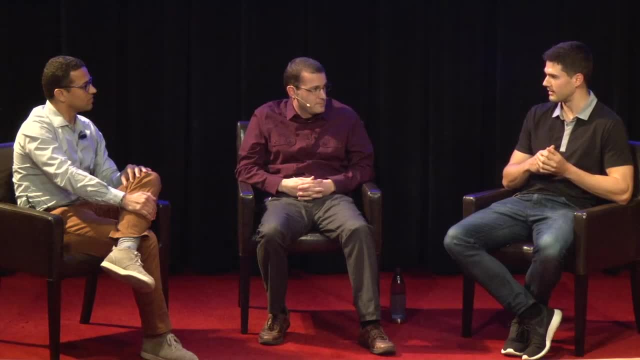 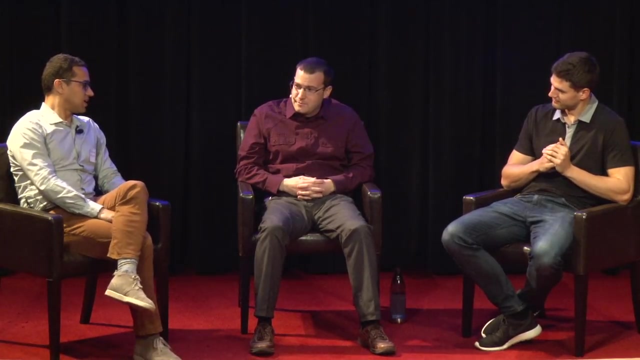 not to make those discoveries because we're worried about, you know, the fact that we can't ask the machine learning model. you know what it was thinking. OK, So that means that in the future, like in 2040, when I will go to conferences, 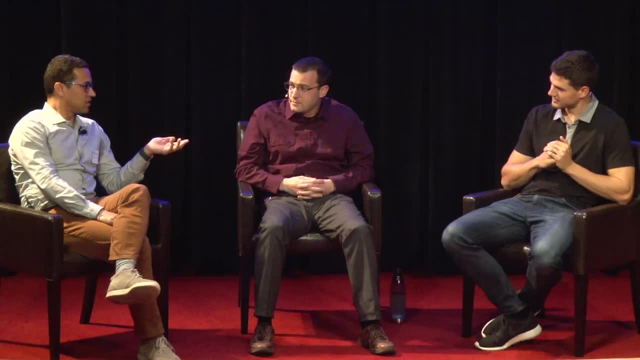 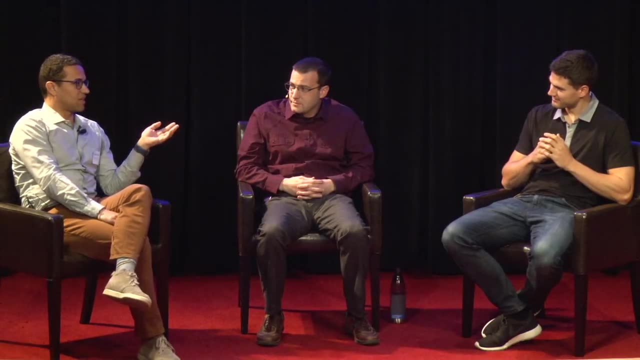 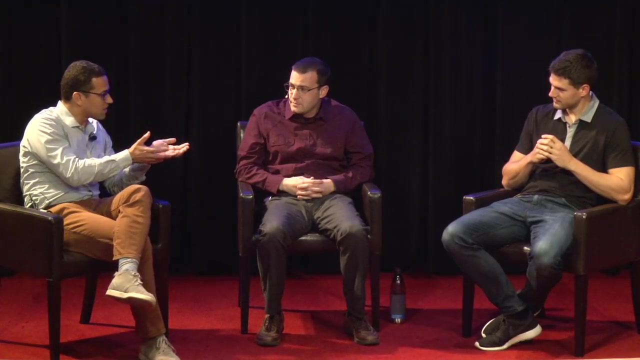 people will be presenting their results and they will say: I use this neural network XXX state a name, and that will be kind of. They may have some difficulties to explain the process behind it and the laws, but they will basically give us the information. 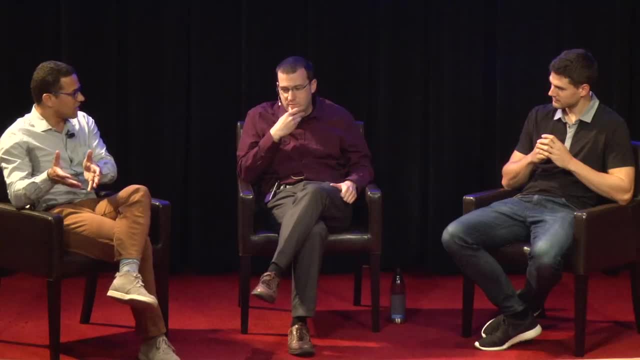 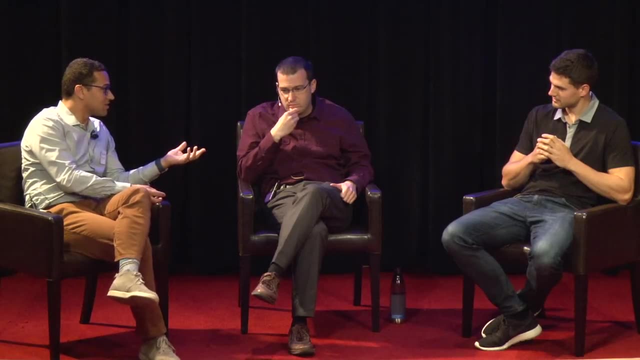 the feeder, the tool they use and the outcome. But that's not really the scientific method we had in mind in the past. There will be no explanation, So yeah, so actually, there's a lot of work going on at the moment. 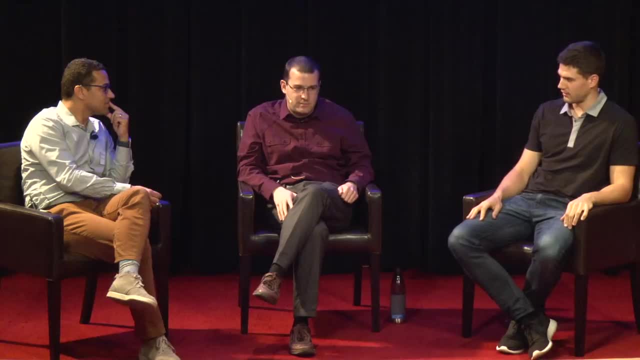 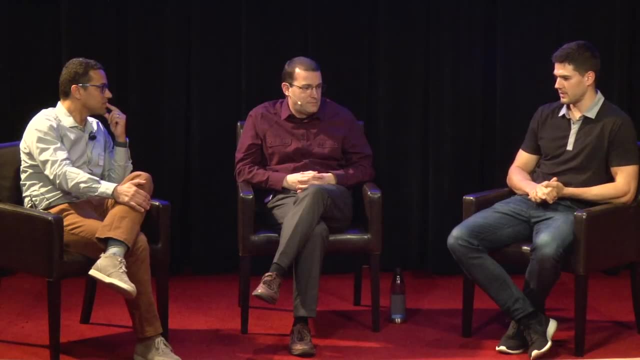 for interpretability and understanding of machine learning models, And you actually can in many cases come up with excellent sort of visualisations and sort of other explanations for why a model made a particular decision, And certainly the problem is not solved, The task is not completely solved. 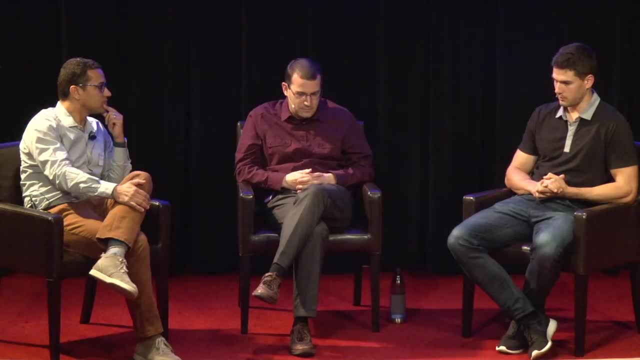 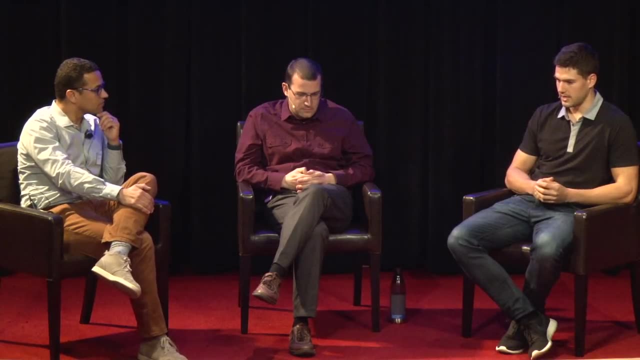 There's active research going on, But when we trained our model, for example, we fed in certain signals that we knew were planets and we used some techniques to try and highlight which portions of the light curve the model was using in its decision And the model would highlight. 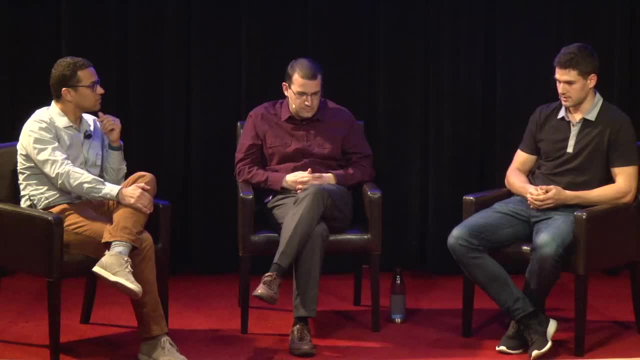 the transit, which gave us some confidence that it had learned which shape was causing it to label this a planet. And then we fed in some various other types of signals that were not planets. Jeff mentioned eclipsing binaries, So we fed in an eclipsing binary. 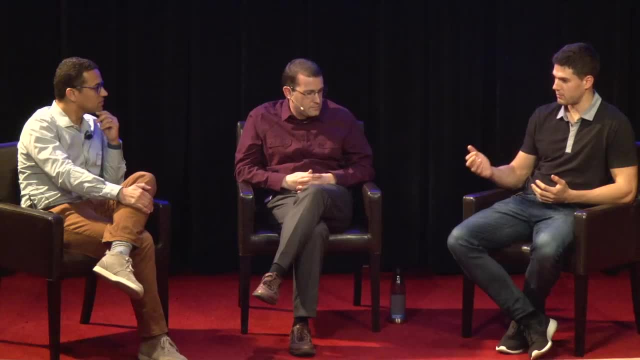 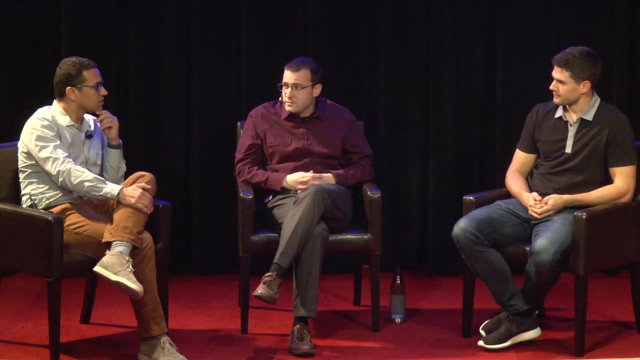 and when we visualised that prediction, we actually found that it had zoomed in on a secondary eclipse, And so we were confident in those two cases that the model was looking at the right places in the light curve at least. You wanted to add something about this. 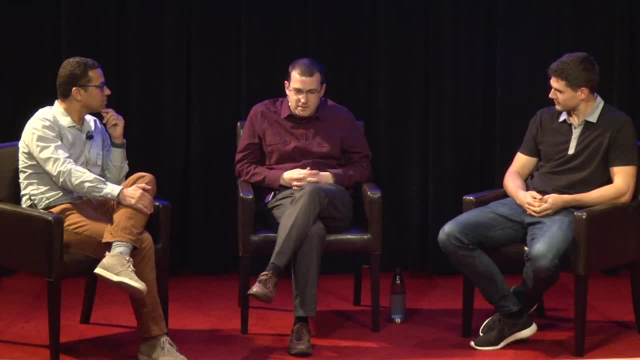 Well, I guess this might be a little bit of a different take on it. So you mentioned scientists going to a conference and presenting their work and saying: well, how did you come to this conclusion? I said, well, I don't know. 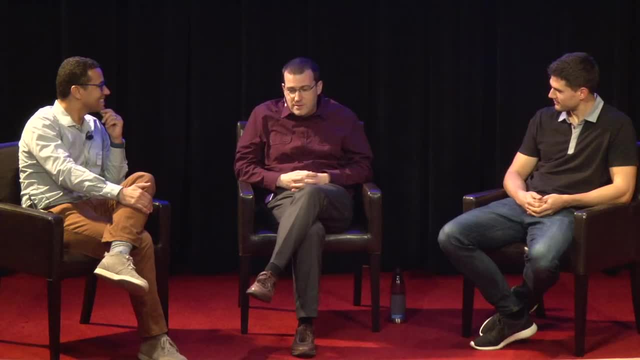 The machine did it And how many scientists or engineers know every single aspect of their work. You know there's plenty of aspects in Kepler that I don't know anything about. I'm not a CCD engineer. I don't know how that all works. 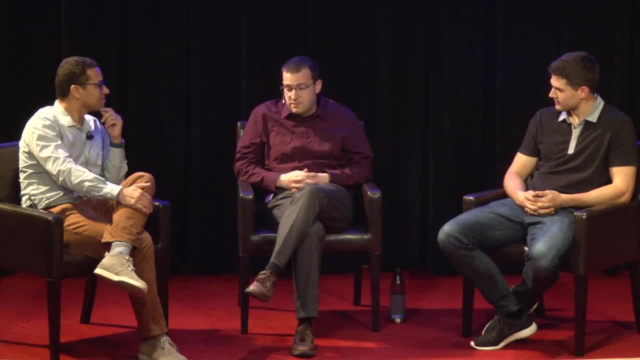 But in some parts you have to believe the experts and that particular aspect and it's teams of people working on discoveries and the individual giving the presentation might not necessarily know every aspect of what's going on And there are machine learning experts. 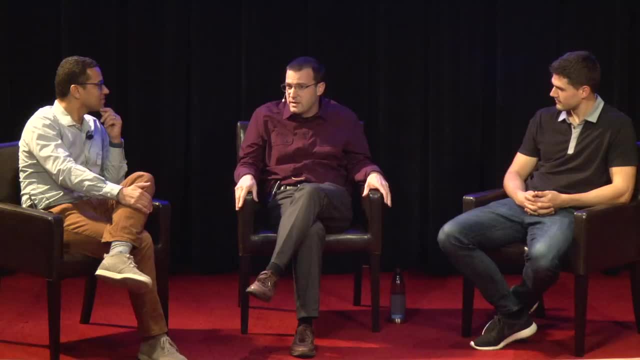 and there are people that understand how these work, And so I guess it already happens that a scientist will present work and they don't actually know how the discovery was made, or at least not every aspect of it. All right, So that's a fair point. 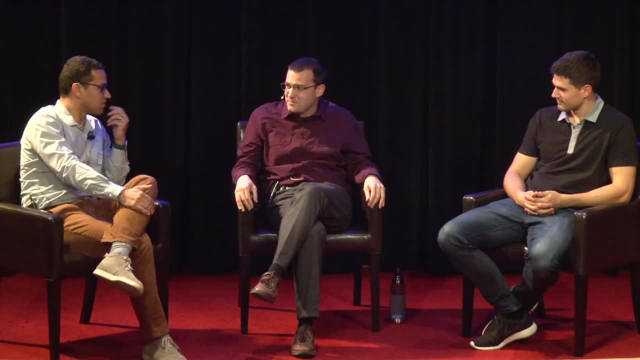 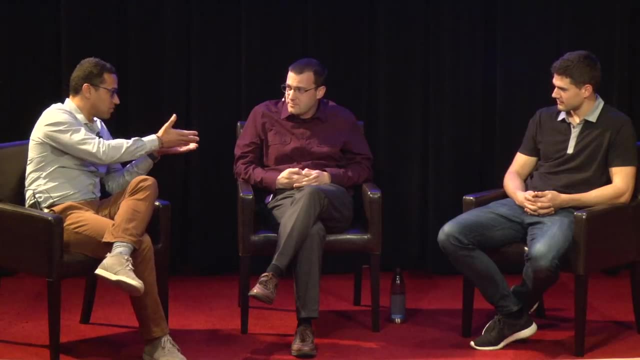 So the future, basically the way we should see that summarize this- is that in the future machine learning will help us. It will be kind of another part of a discovery process. As you mentioned, you find some interesting target thanks to machine learning. 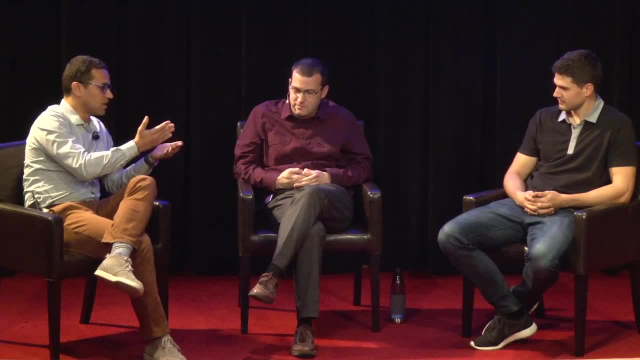 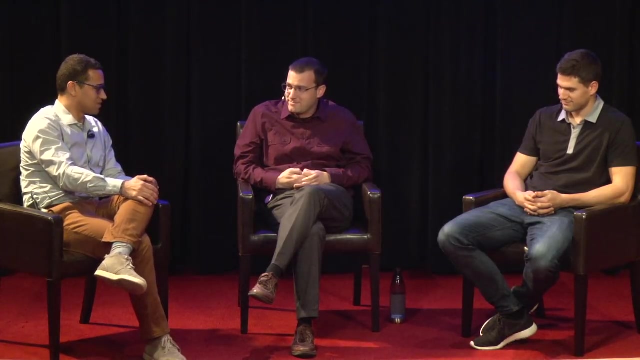 and then you went back into the data and you analyzed them and you discovered that this was. you validated the result. So the computer is like something that helps you, like a grad student or postdoc, but faster and cheaper, Okay. 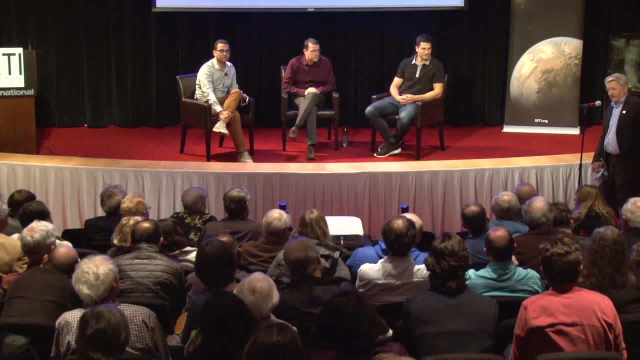 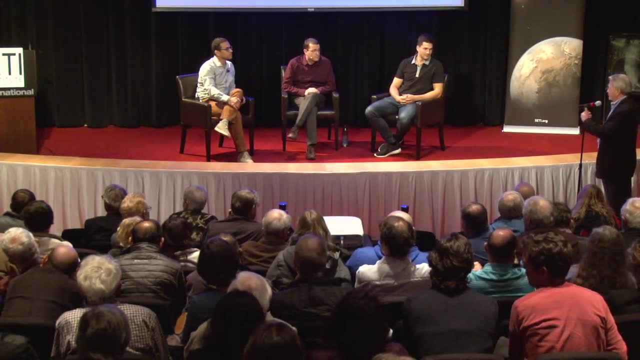 The floor is open for questions. So if you would like to ask a question, please come down to the microphone. and I'm going to start with a question, Jeff, that I think comes up a lot because of course this is a binary problem. 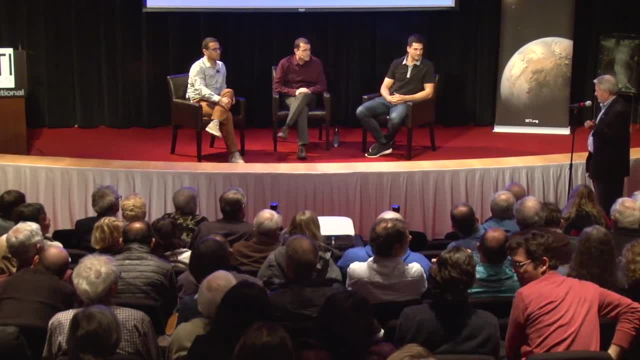 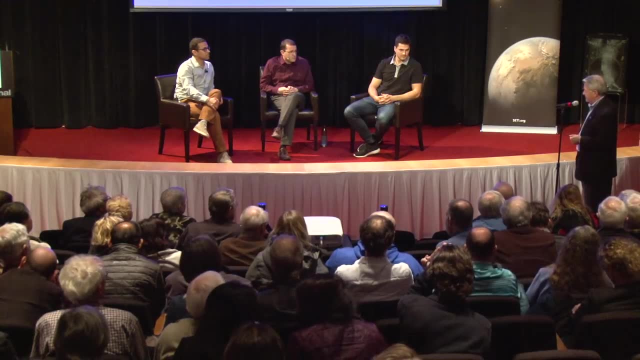 planet or not a planet? I think some people here might be curious as to what is the validation process. So you say, well, I mean we've seen in the data sets you showed us tonight, light curves which look remarkably the same. 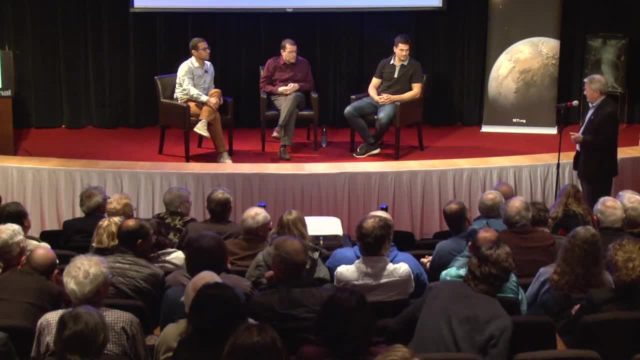 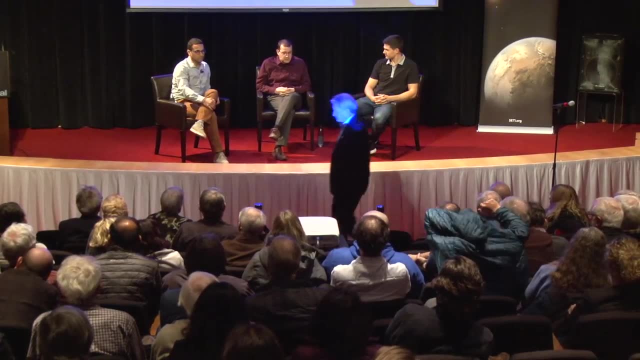 and in one case it's a planet and in another it isn't. Maybe you could comment a little bit on how planet discoveries are. Yeah, Well, that's an absolutely critical aspect of this discovery process, because Kepler and TESS are just these survey missions. 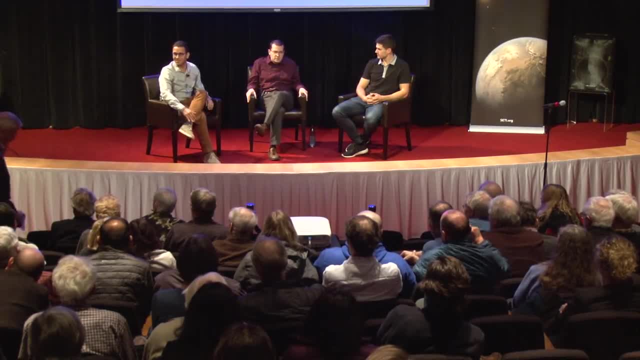 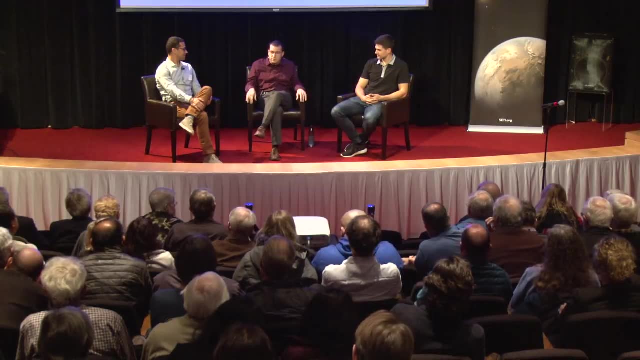 trying to see whatever signals we can get out there. but just because Kepler or TESS detects something doesn't mean it's really a planet. So most of that is background-based observations, follow-up observations, to see: is there something else that's looking like a transit. 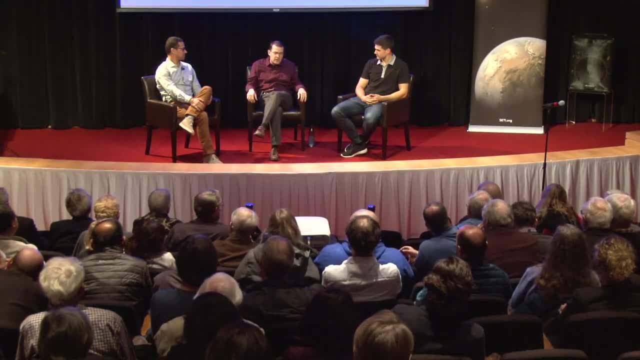 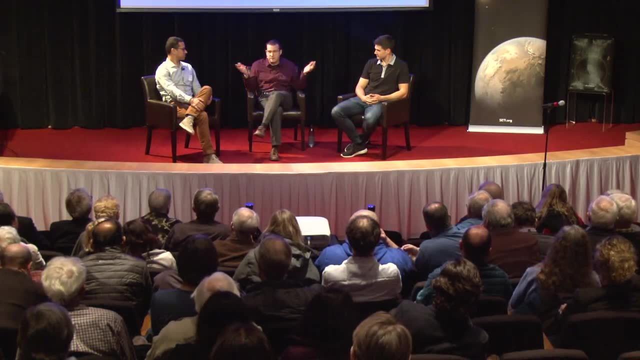 that really isn't Many times it would be a background object. There are cases where you can statistically look at the systems on their own and statistically say 95 or 99 percent are going to certainly be planets. but you can't necessarily say this one's a planet. 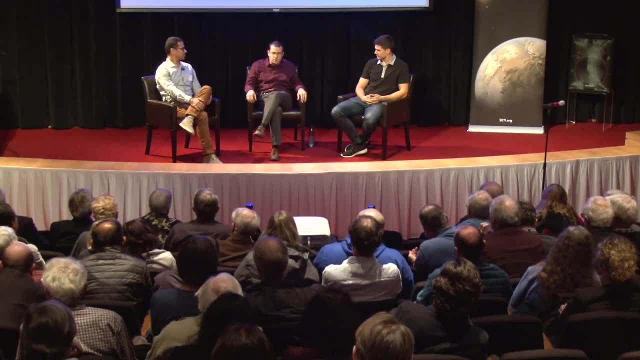 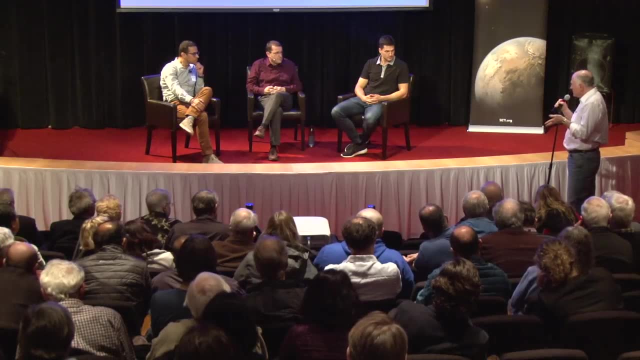 You're just saying 99 percent are something, But the basic answer is follow-up observations, ground-based observations. Okay, So you said you trained on 15,000? So that seems like a small number to me, Did you do? quote. 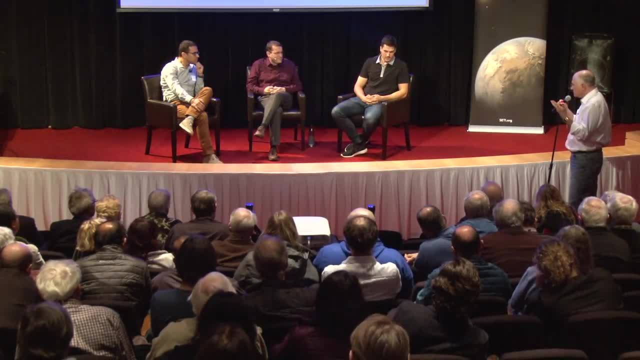 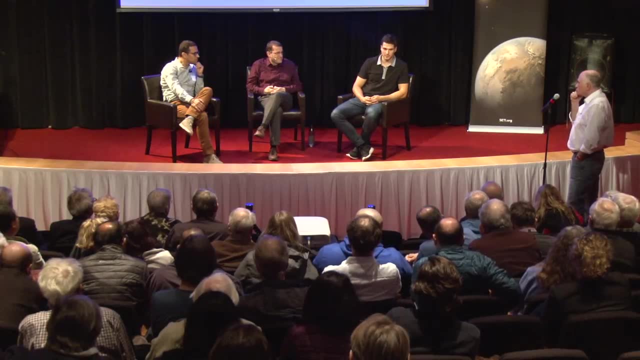 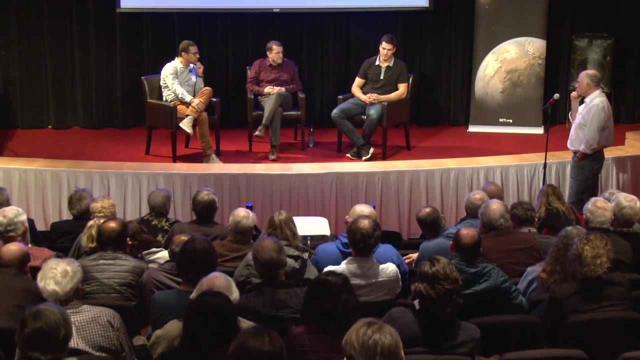 data augmentation or some other scheme to generate more data. Yeah, So 15,000 is definitely small on the scale of the machine learning models that we usually train. The one data augmentation trick we used was we took all the light curves and we reversed them. 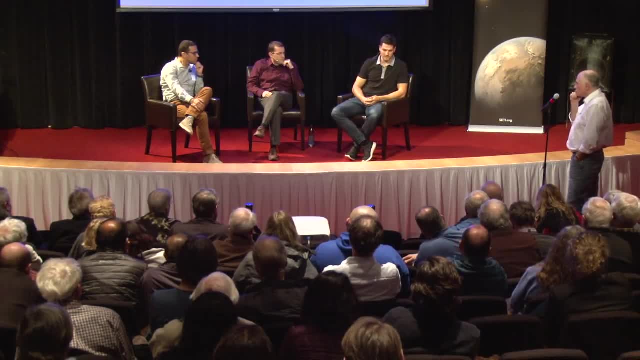 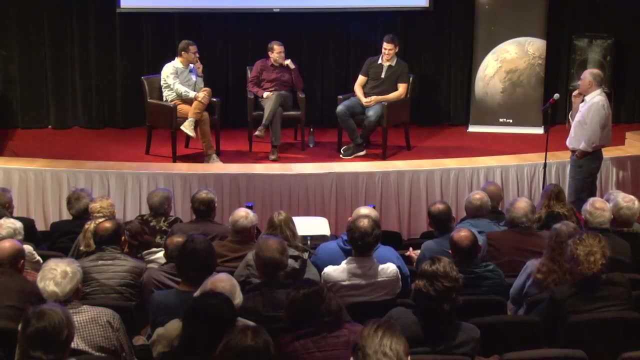 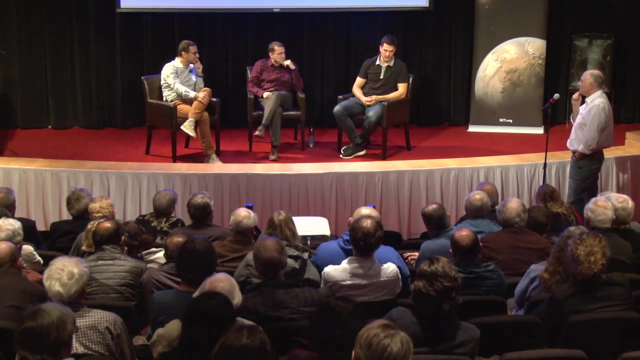 And so in that way, we were able to double our training data to about 30,000.. Then you flipped them too, and that's another doubling. No, didn't go upside down, But we reversed them left to right And we were unsure. 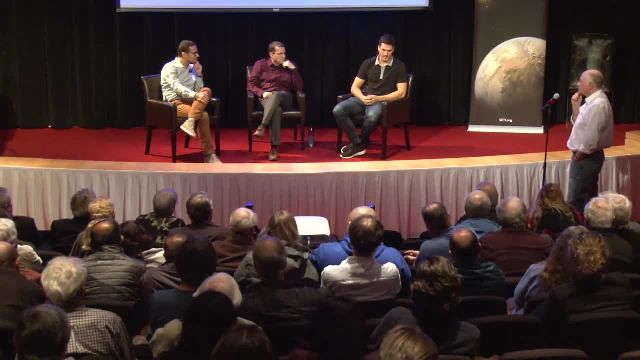 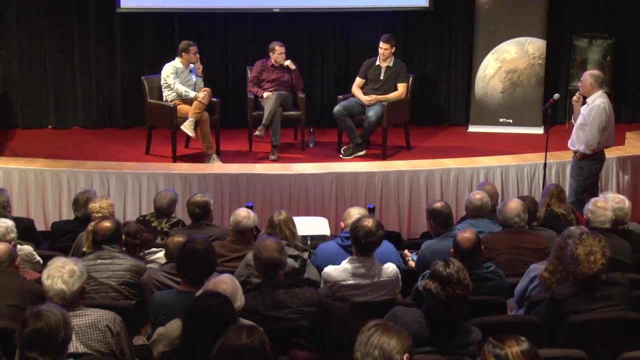 whether those 15,000 would be enough, but we kept our model relatively small compared to some of the other big models that we use. on those, you know data sets of like over a million training examples, And you know. 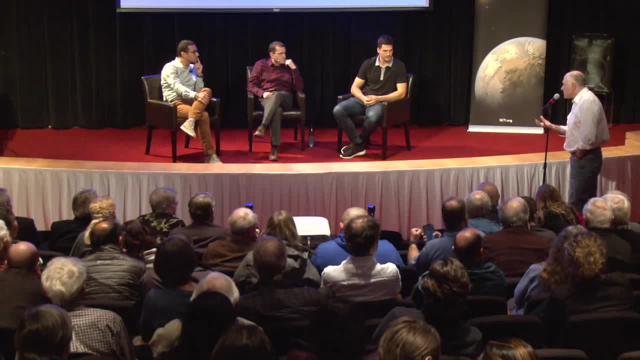 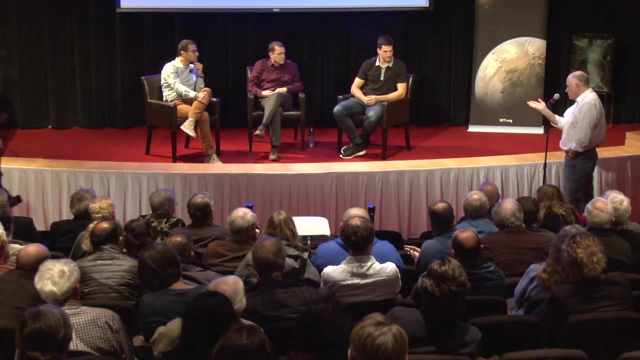 we found our model to be fairly accurate still, And you had a measure of error in the training set in the first place. I mean, it's not perfect data right, So people will goof and they see a planet where there's none. 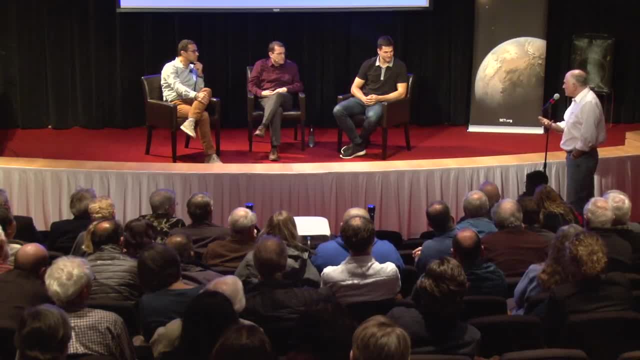 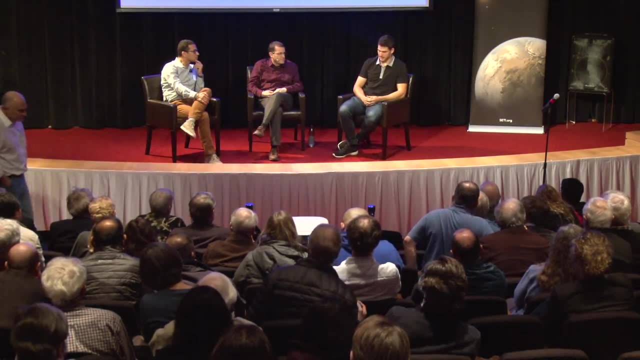 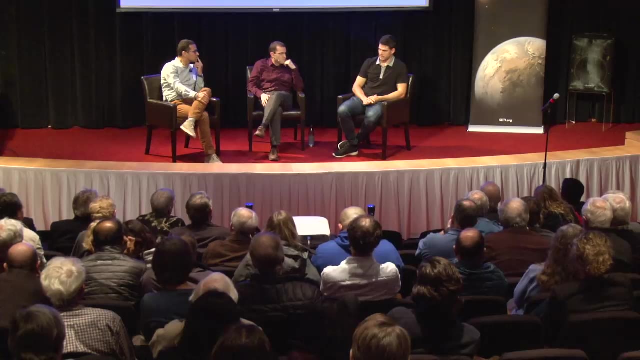 and they see no planet where there is. So how did you handle that? Sure, yeah, So it's certainly true that some of the examples in our training set may have been mislabeled. What we did was we held out a portion of our training data- 10%. 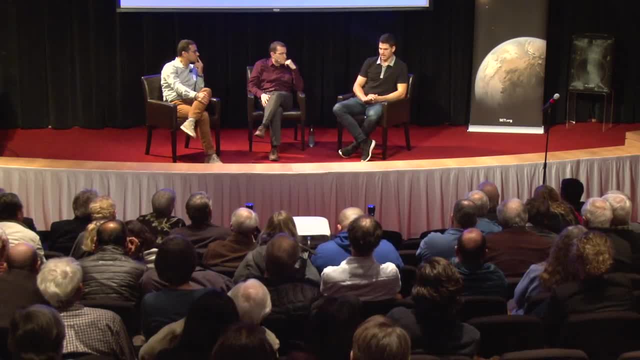 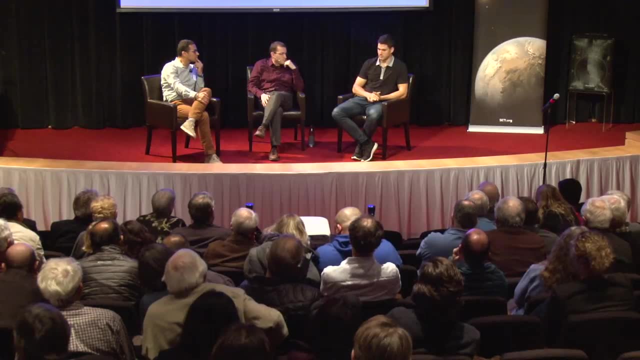 and we did not show that portion to our model at all during training And then to test how accurate our model was. once we trained our model, we evaluated it on that 10% and we found it got 96% accuracy, which we thought was pretty good. 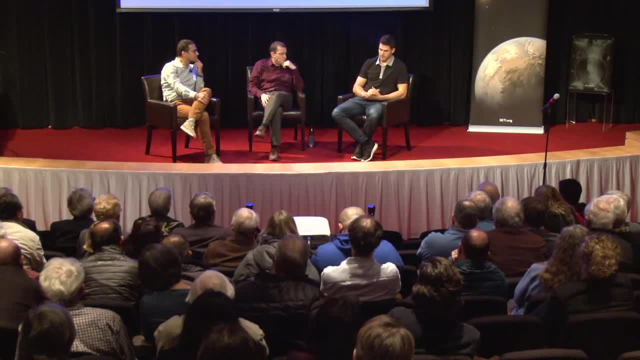 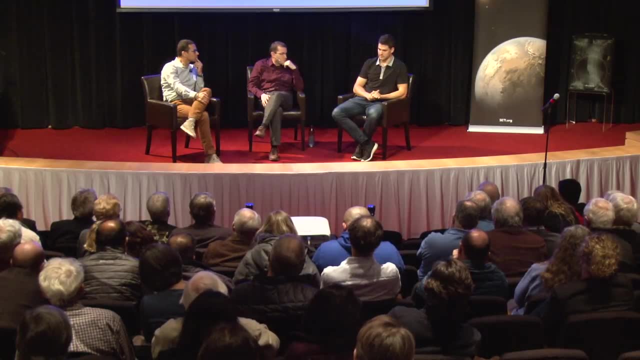 It does not mean that if we then use that same model and go searching for these through these weaker signals, that it's also going to be 96% accurate, because a lot of the signals that our model trained on were very strong signals So it's unclear exactly how accurate it is. 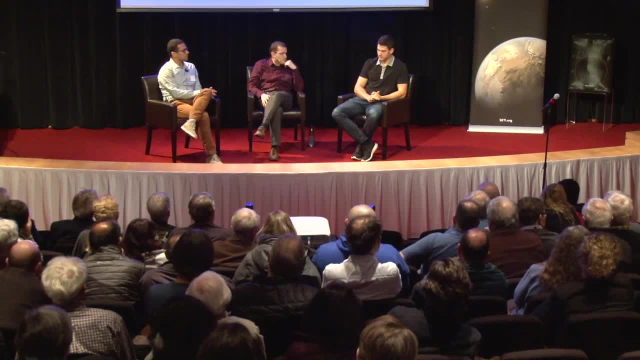 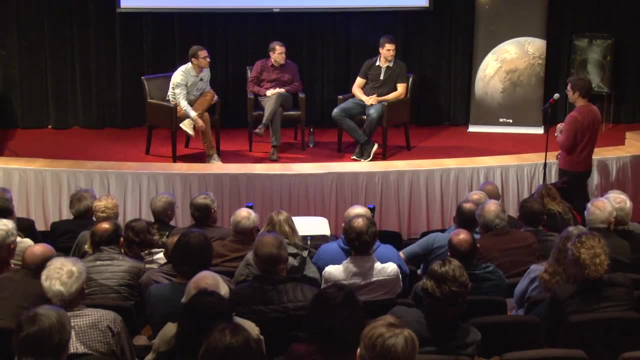 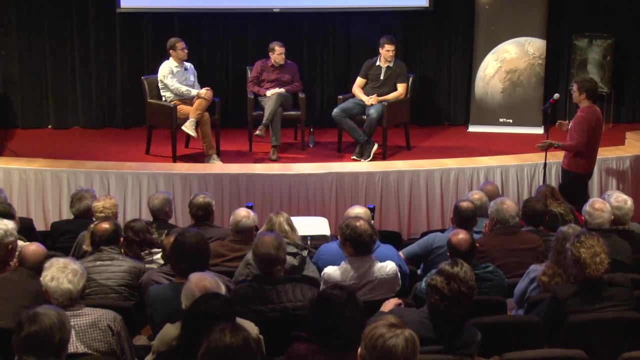 on the weaker signals, But we believe it's quite accurate on its training data. Go ahead. You had mentioned that you're using a simulator to simulate the test spacecraft that you're then using to train models. Are there any plans to after the spacecraft's launched? 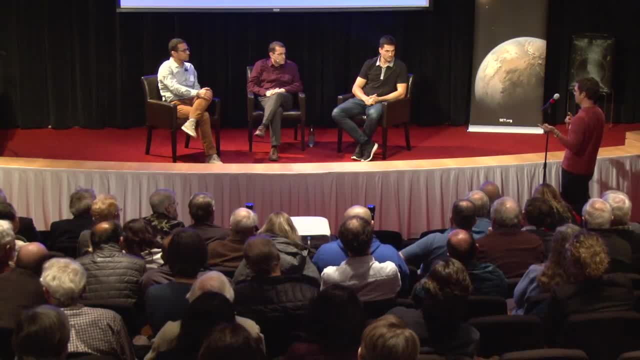 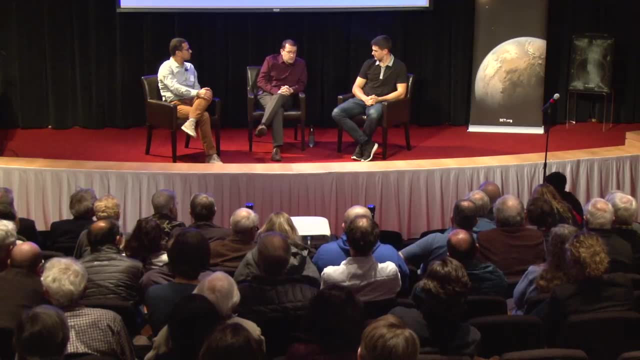 basically take some real data and compare it and use that to tweak the simulator. Certainly, Our simulator is based on our experience with Kepler and there's big differences between the two, So we don't know if what we're simulating is exactly right. 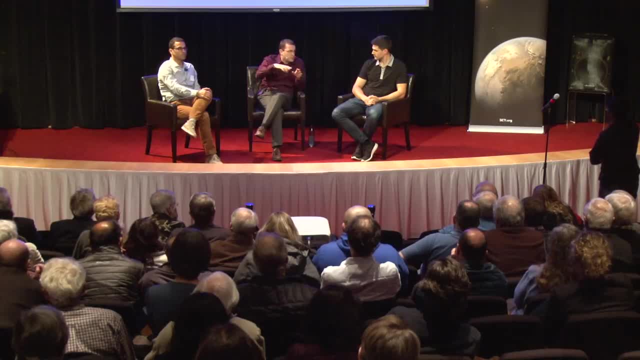 Thermal equilibrium, the time to get thermal equilibrium and things like that could be completely different. In fact, it probably is, because it's much smaller And we think we scaled it right, but we don't really know. We have a lot of algorithms. 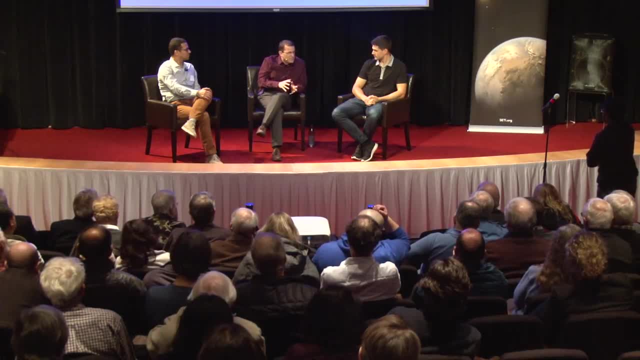 in the pipeline that are tuned kind of well and we don't want to spend too much time tuning it to the simulated data, because once we get real flight data things are going to be different. So there's certainly lots of opportunities to look at the real data. 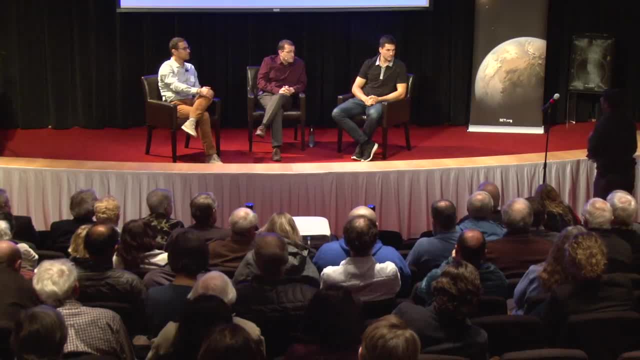 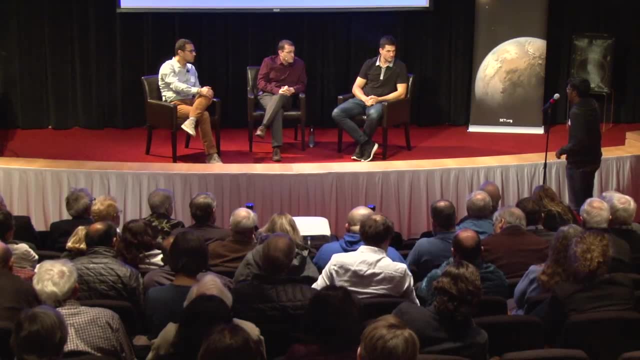 and figure out what we got wrong in the simulator. Thank you for the talk. So I wanted to ask: now that we are using AI and machine learning models to predict planets, is there any, or are there any changes that you made to the kind of data? 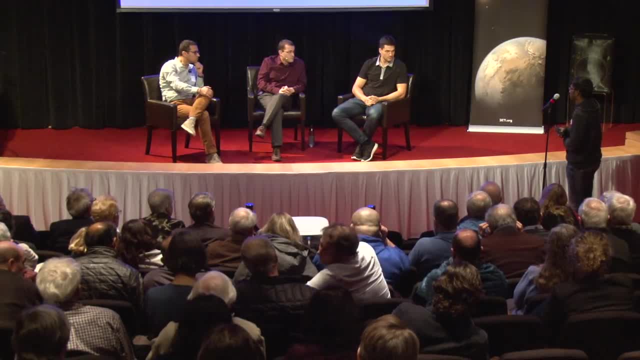 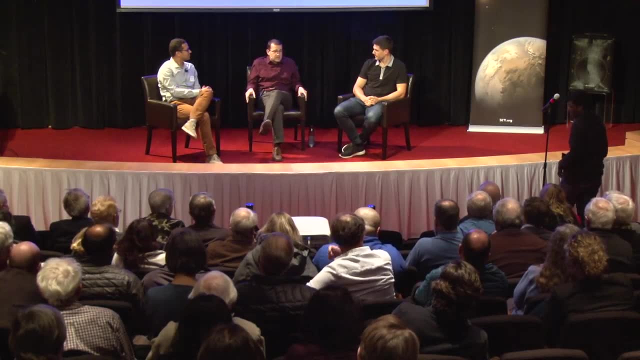 that you're gathering or any changes to the procedure in which you want to gather data. Well, I have ideas, Even though, technically, there's aspects of machine learning and there's a couple things. There's, technically, an unsupervised learning method. 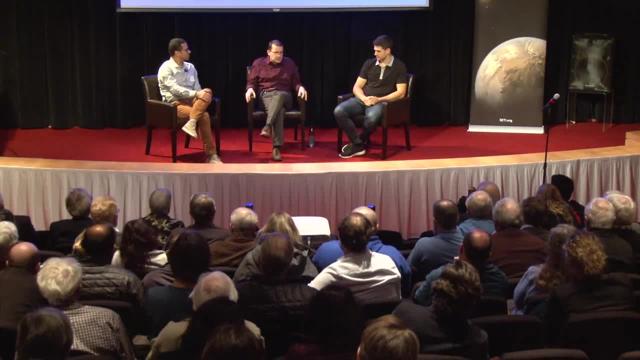 that's used in the pipeline and a couple other things. There's nothing like deep learning. There's something like that. that's in there, And I have ideas of ways we could incorporate it in and to aid in the actual processing instead of just simply. 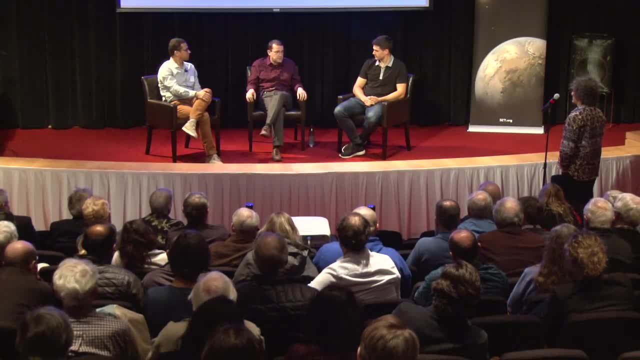 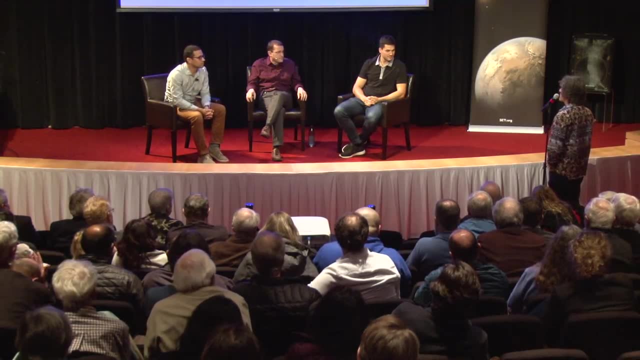 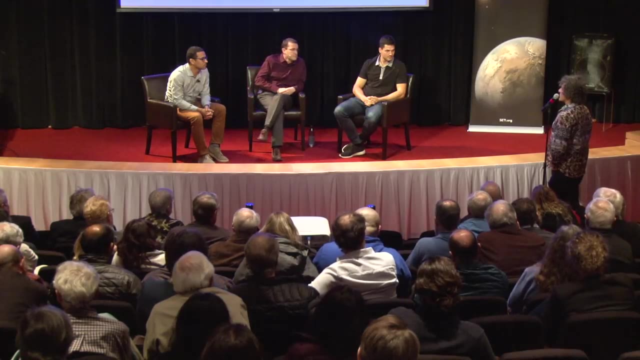 taking the products and classifying them. So there's certainly opportunities there. I have one question for Jeff and one for Chris, or Jeff, In a lot of the sample curves that you were showing to illustrate how difficult the problem actually is, some of them looked very noisy. 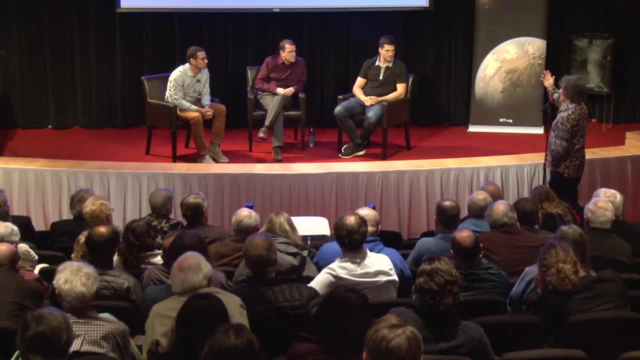 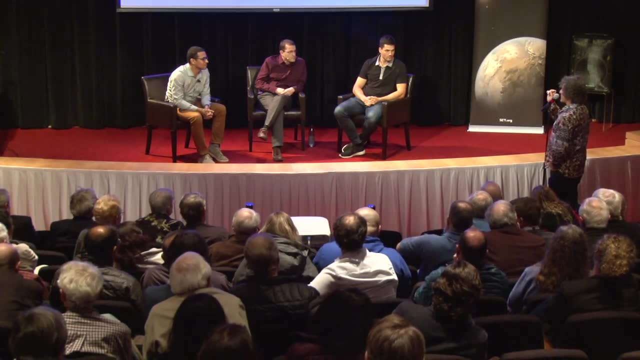 and others- and some of the noisy ones- said planet and others said no planet. Some of them looked a lot like planets and they said no planet. So I wonder if you could possibly just elaborate a little bit on how the humans make these distinctions. 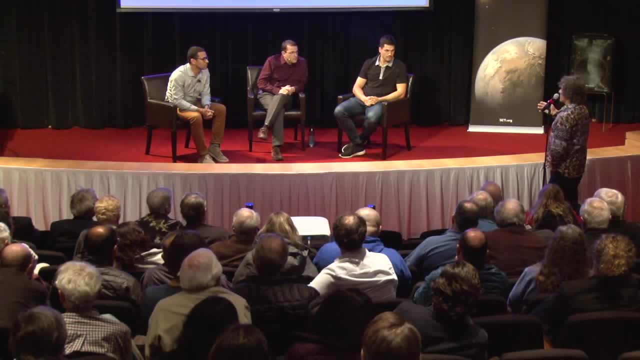 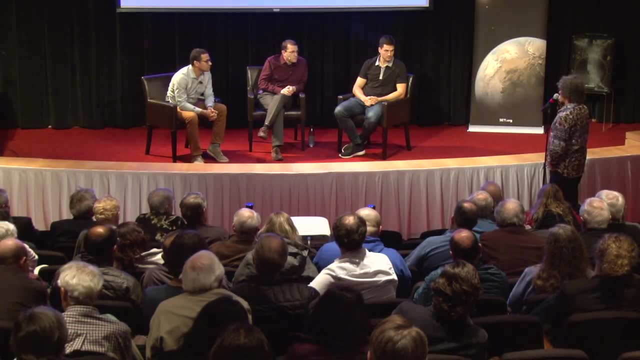 when, to the untrained observer, the light curves are either content free or would fool you into thinking it was a planet. And then for you, Chris, the question is: it was interesting that you had the curves at multiple scales being fed into the bottom layer. 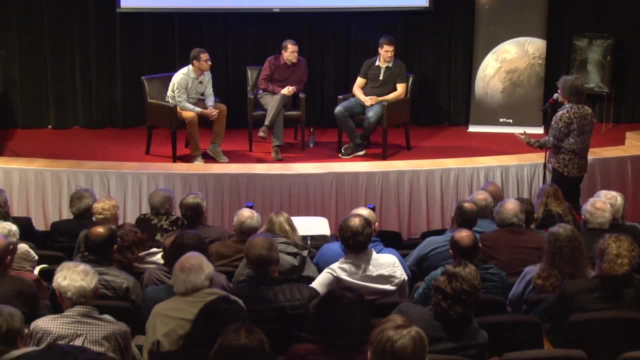 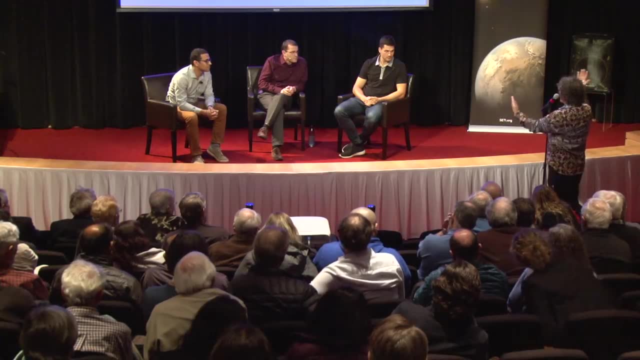 Were you feeding the raw curves or the calibrated curves with all these artifacts removed? And were you feeding in the whole really year-long light curves, or were you folding them? And if you folded them, how did you figure out where to fold them? 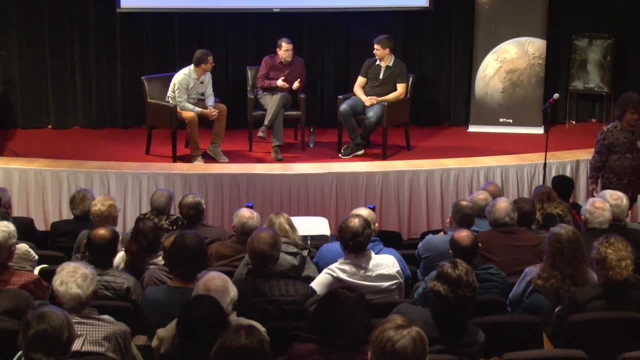 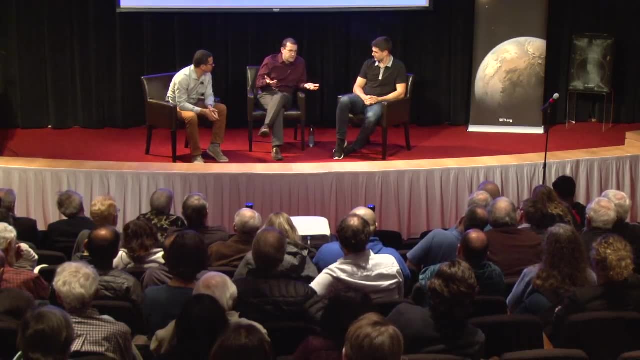 or did you just try everything, Okay? Well, those are both excellent questions. What I'm showing you is just the light curve and there's actually all kinds of supporting information, And there's actually for every individual planet that we look at. 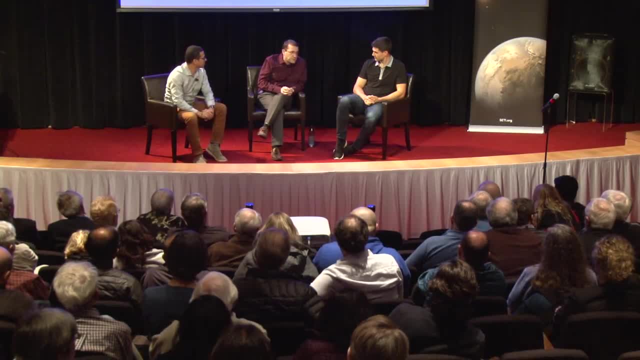 there's upwards of 100 pages of information in these DV reports And so if I showed all the information and I went through it all, I'm not sure about every single one of those, but some of them we could identify. ah, that's a background object. 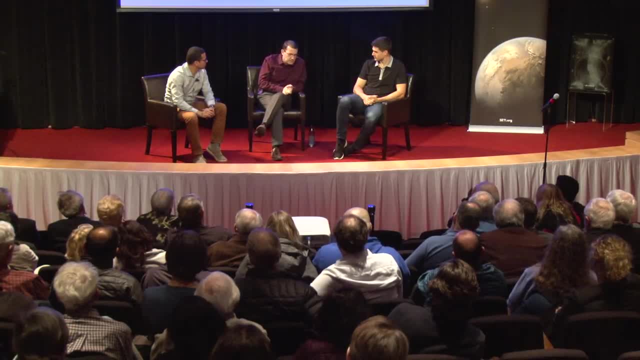 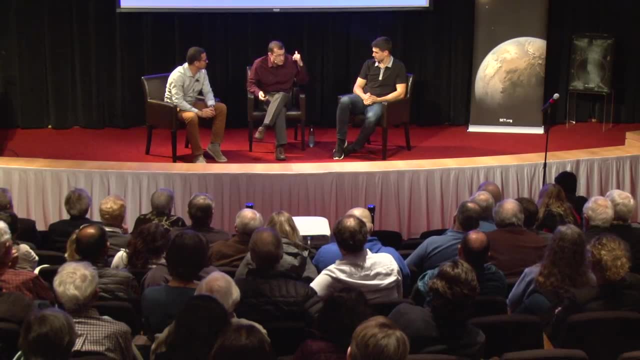 Or we have these statistical tests. There's this bootstrap test that determines if the detection is indistinguishable from random noise, And the one that I showed that was indistinguishable. that was actually random noise. our bootstrap statistic actually showed that it actually fired off. 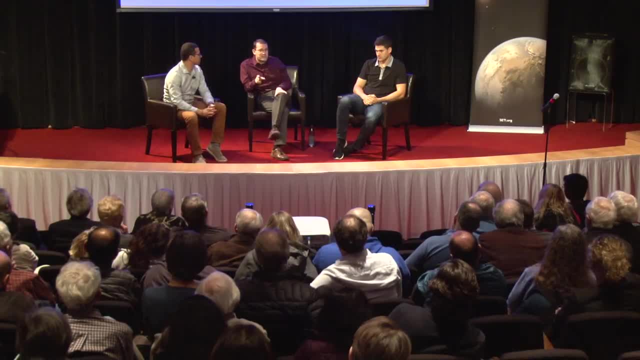 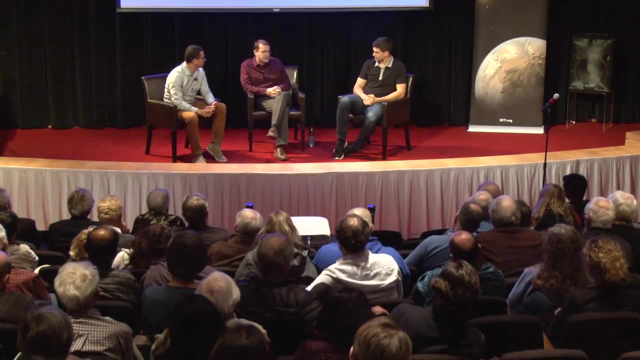 saying this looks like noise, So I'm kind of being mischievous here by just showing the light curve. We actually have a lot of information, but all that information takes a lot of time to go through, And that's kind of the key here. 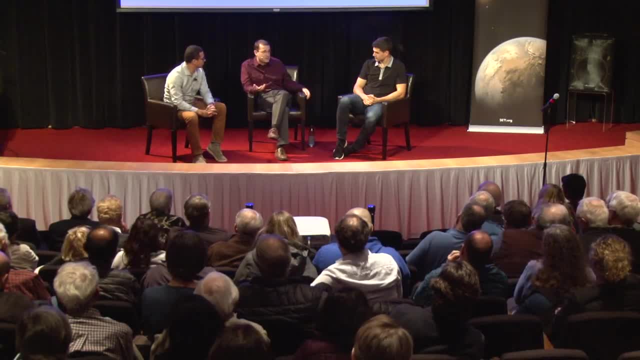 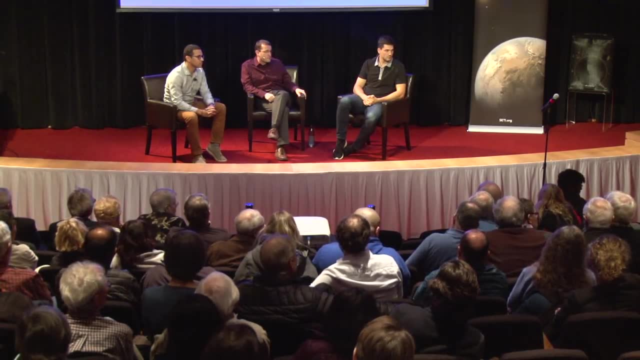 is. you've got to go through 100 pages of information to determine if you really think it's a planet, And a machine could do that a lot faster. Were follow-up observations involved in saying whether it was or not a planet? Could follow-up observations? 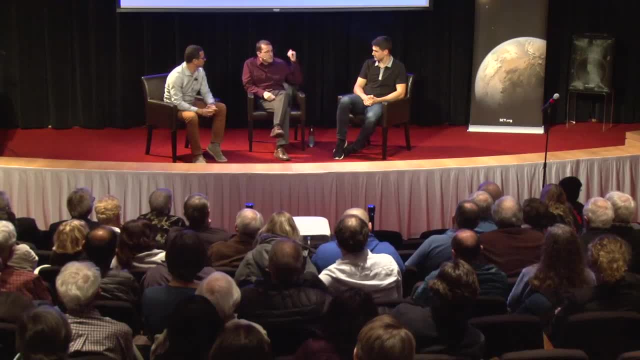 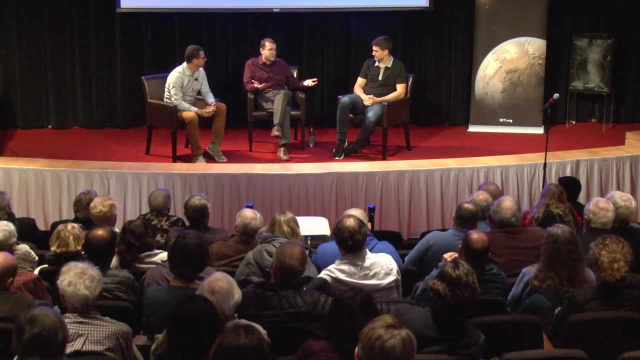 Were they involved? Well, they are In real life. they are. I mean, these were simulated, But yeah, this was what I showed. The light curves at the end were all simulated, So I knew the truth. Yeah, so to answer your questions. 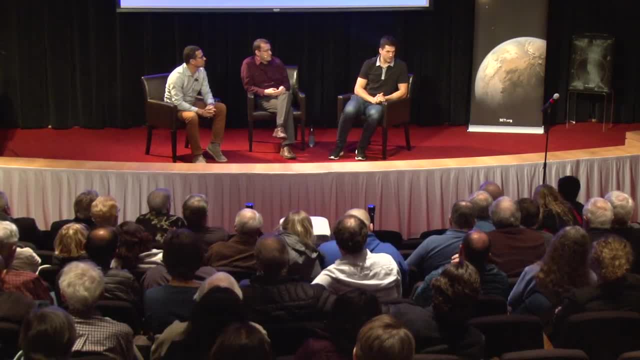 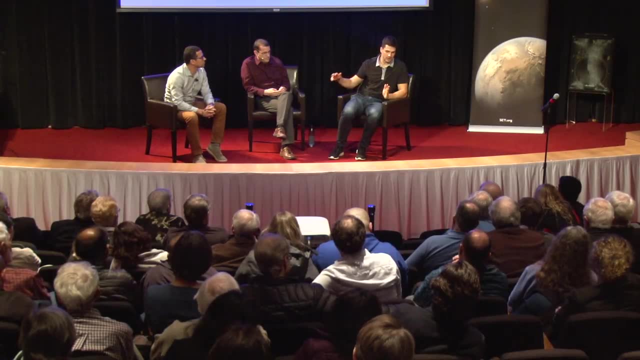 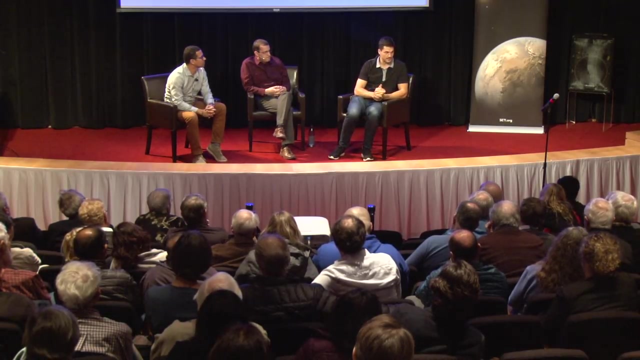 we used the calibrated light curves. We did some processing to flatten away any of the stellar variability In the images I showed of the transit. we did in fact phase fold. We knew where to phase fold because everything in our training set was an existing detection. 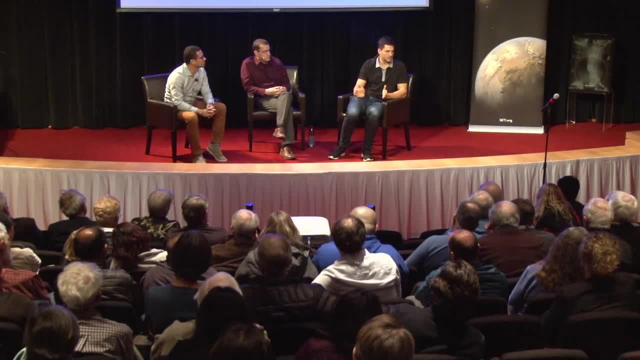 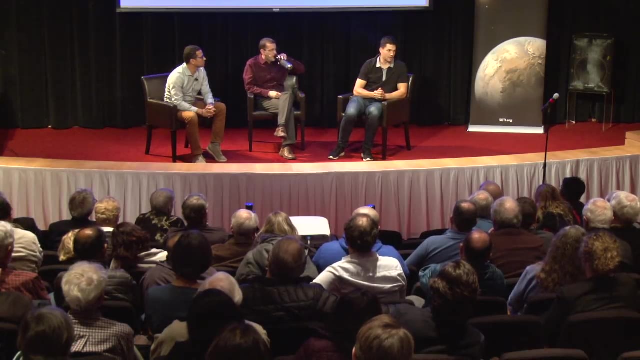 So we knew where the detection was and what its period was, And so that's how we phase folded everything in our training set. When it came to using our model on new data, we needed to first run an algorithm to actually come up with candidates. 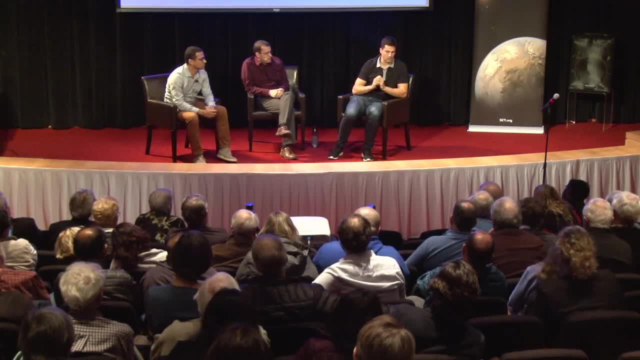 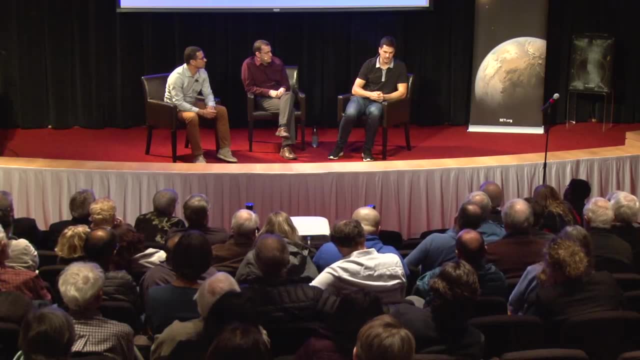 to feed our model, So our model didn't then go and just look at raw Kepler data. We first ran a first-pass detection algorithm to come up with candidates. I think we came up with something in the range of 500 candidates, And then we used our model. 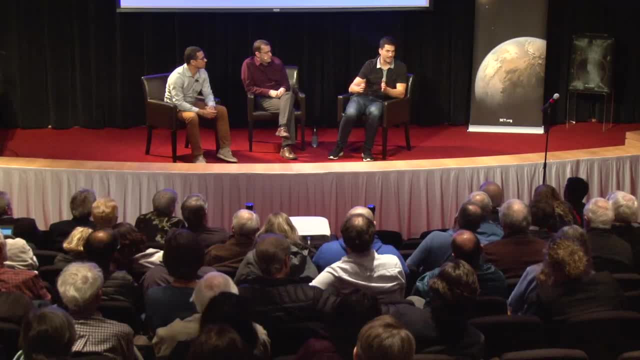 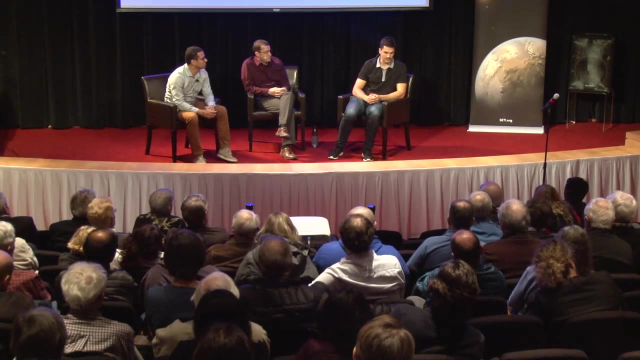 to predict the probability that each of those 500 candidates was a planet, And almost all of them it said no. And then there was, I think, only eight or nine that it predicted were probably planets. And then Andrew, who's the astronomer in this project. 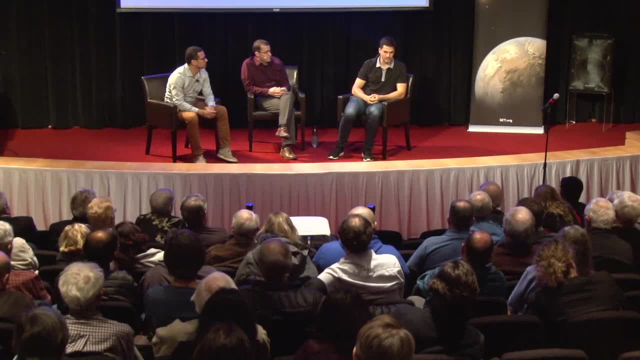 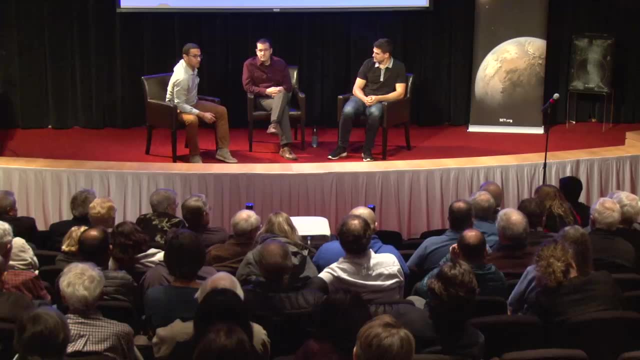 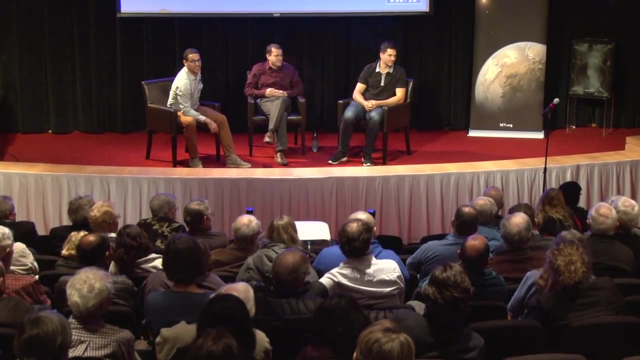 went through and looked at them and decided he was very certain that two of them were planets. So those are the ones that we validated, Okay, Well, it's time to end this. One question, All right, one, Go ahead. I'd say ten already. 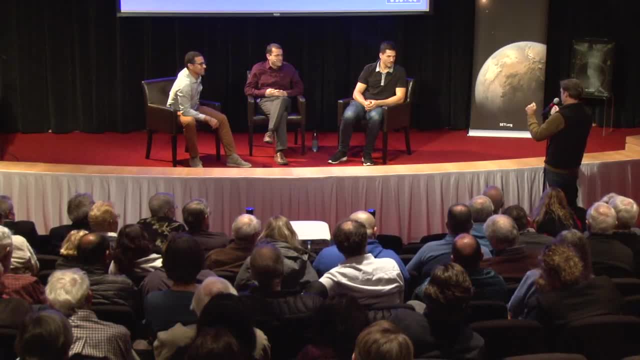 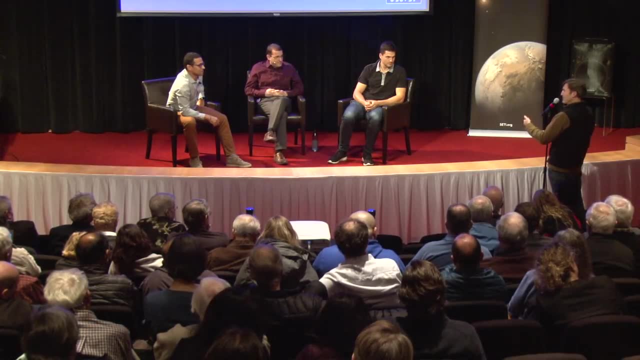 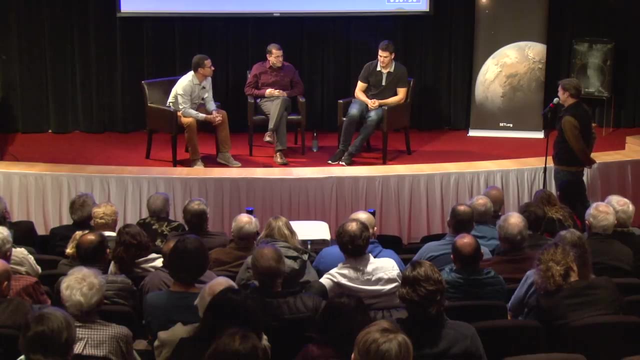 I have a question about now training. Now, since Kepler and TESS have spatial and temporal resolution differences, will you be able to use Kepler data to train for test detections? So this is a question about, I guess, domain transfer. So we see this sometimes when you know. 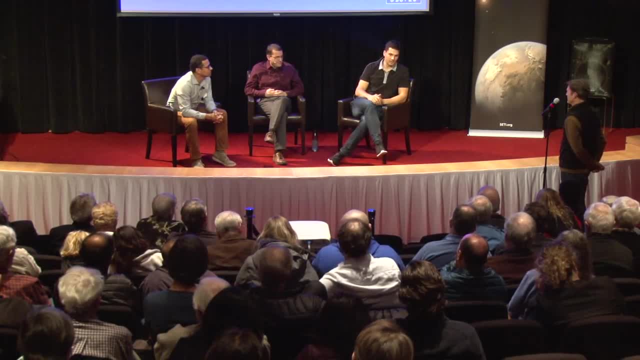 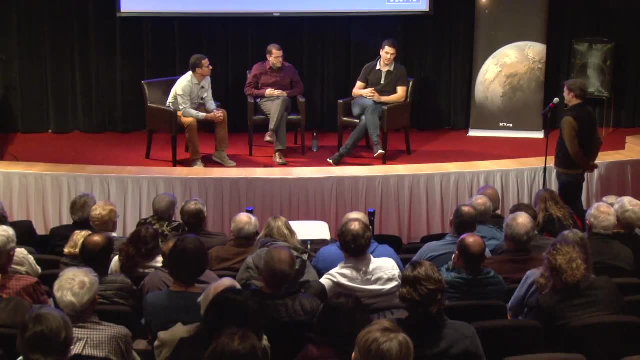 if we have an image classification model and we train it on images pulled from Tumblr and then we have images from, like, a different website, Flickr or something like that, it turns out that even though both websites just have photos, a model trained on one of those data sets. 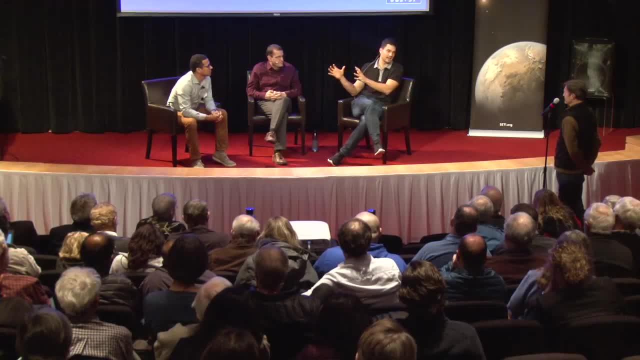 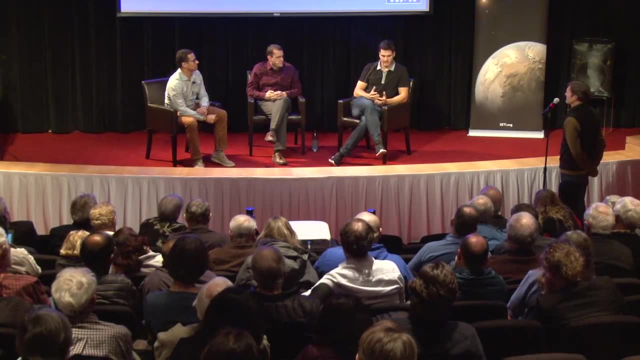 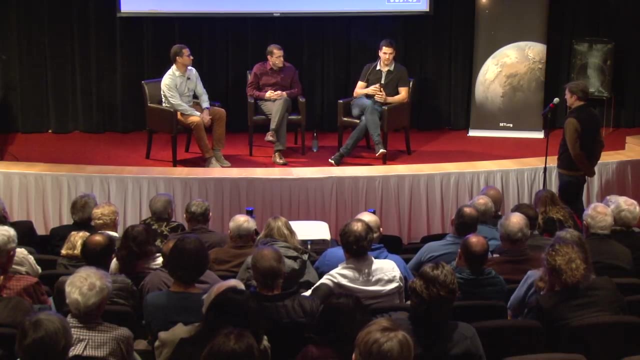 does like significantly worse on the other data set if you don't take some sort of like recalibration into account. So it is possible to take a model trained on Kepler data and start with that and we would do something like try and fine-tune it.